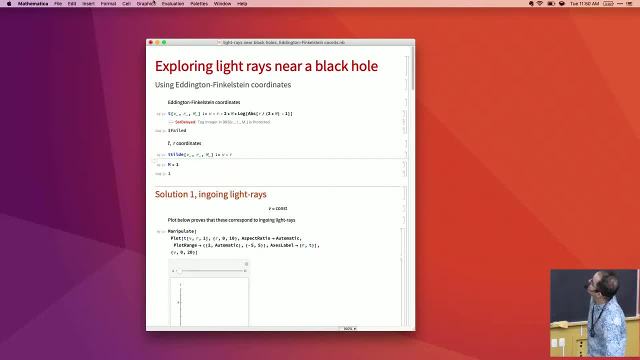 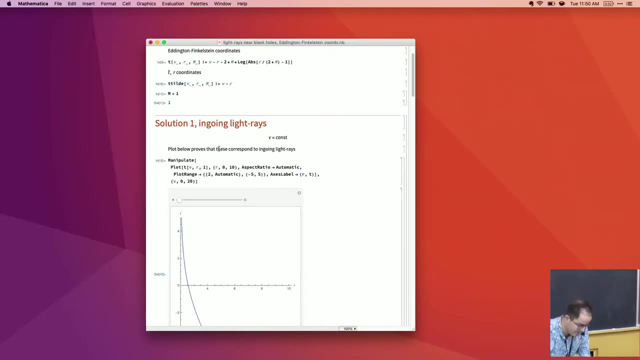 I can give you, I can share. Let me execute this. Let's see evaluate. So what I'm doing here is I'm taking some appropriate coordinates And I hope I will write Schwarzschild correctly. Is this correct? Is it Okay? As you know, the, if you write the, if you write the Schwarzschild, 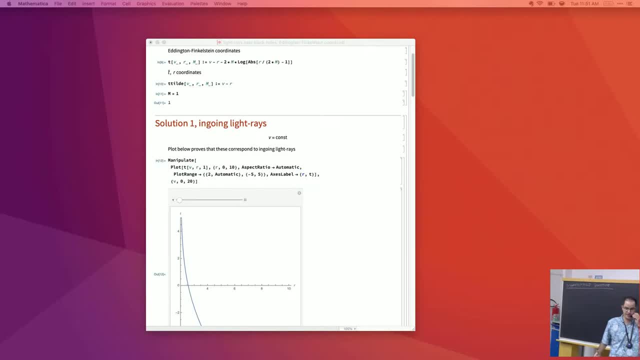 geometry, the geometry of the spherically symmetric object, and you use the Schwarzschild coordinates. the Schwarzschild coordinates, they are not very good because they have coordinates, because they have coordinates. So if you write the Schwarzschild coordinates, they are not very good. 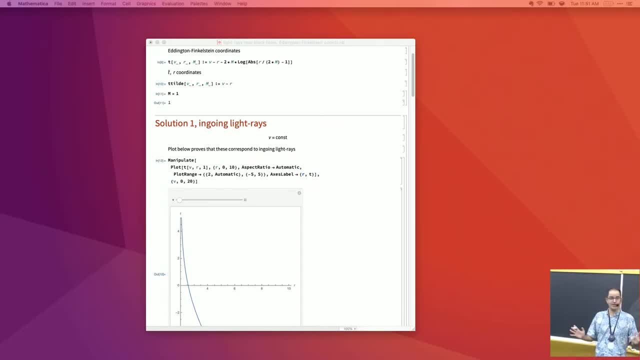 because they have coordinates. They're very, very tocar, So the coordinates they fail and they give you garbage results at the horizon. So what you have to do instead is you have to do. one suggestion is to use these coordinates called Eddington-Finkelstein. It's nothing fancy here. 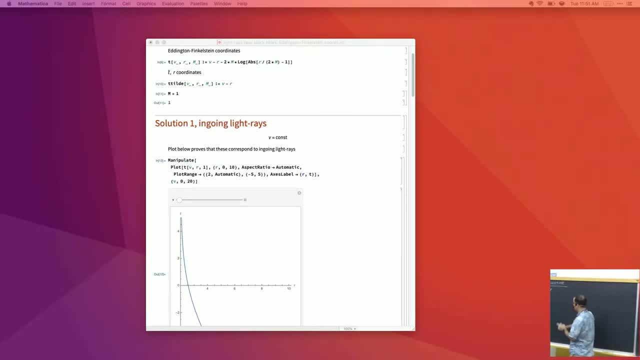 no dynamic, no numerical relativity here, just a static space time. So if you use these coordinates, you can write the line for these coordinates which I will not remember, But you replace time, the time, by some Eddington Finkelstein time, which. 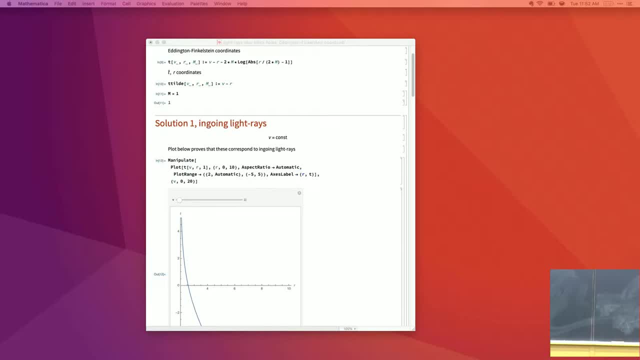 I will call v And then you. this is the only change, basically. So r theta and phi, they remain the same. And here what I will show you is: you want to understand what happens with radial light rays? So, radial light rays. what you do is then you set d theta 0, d. 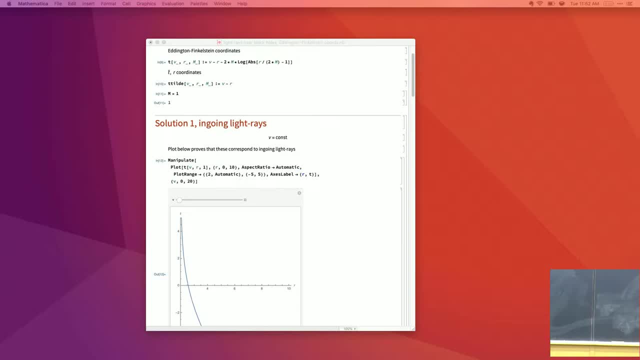 phi 0.. And since it's a light ray, you have to. So you do these requirements here And then, OK, here we specify the light ray. So you do these requirements here And then, OK, here we specify the light ray. 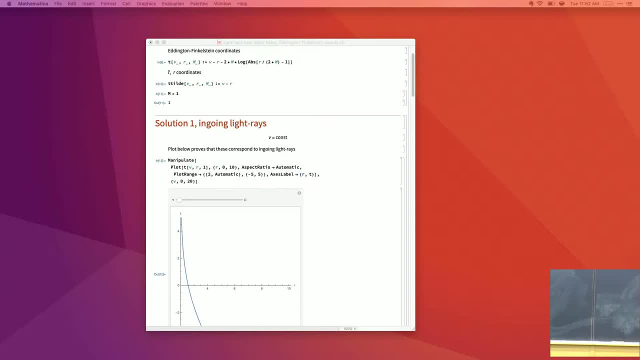 A radial light ray, And then you solve the resulting equation, And then you will have the equation of light rays charged with spacetime, And then you can plot what will happen with the light counts. And that's what I've done here. Let's see which one of these. Yeah, 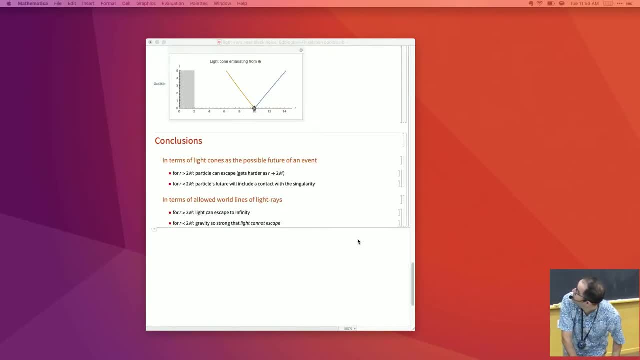 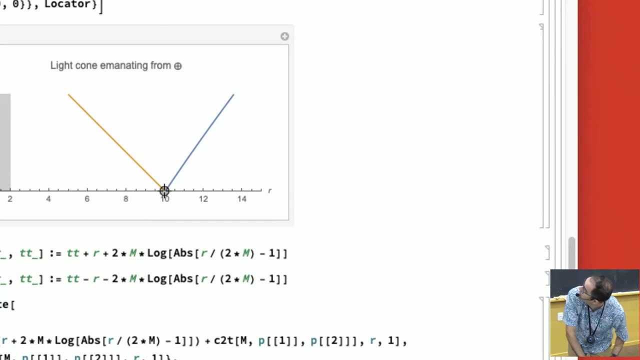 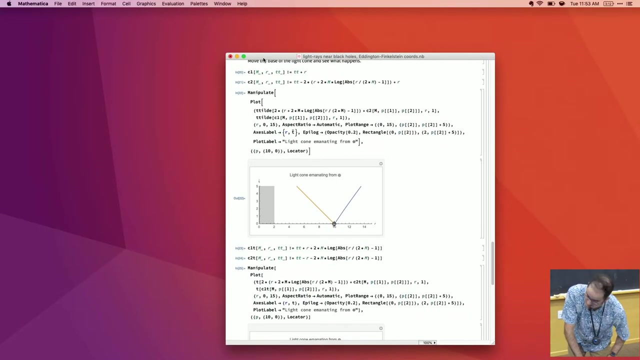 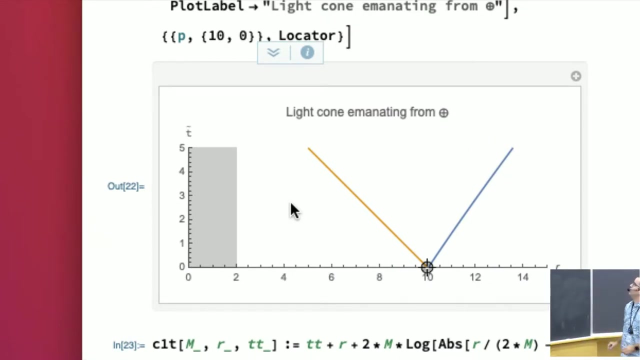 that's the one, Oops. OK, so the blue line corresponds to a radial light ray which is trying to escape the black hole. OK, so the light ray is like: look, I want to go, I want, I don't want to. 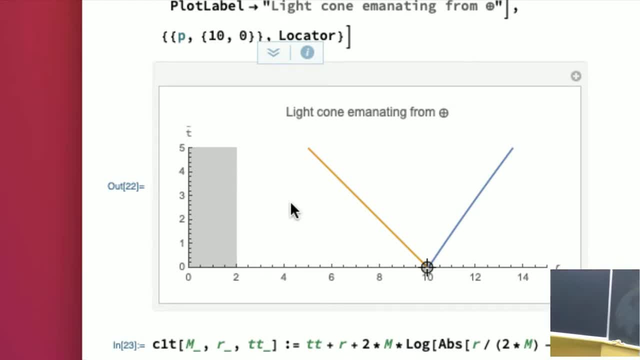 fall, I don't want to die, No, no, no. That's the blue light ray. And the orange light ray is: imagine you have a flashlight and you are falling towards a black hole. Well, that's a static event, but imagine you are falling in a black hole and you have a flashlight. 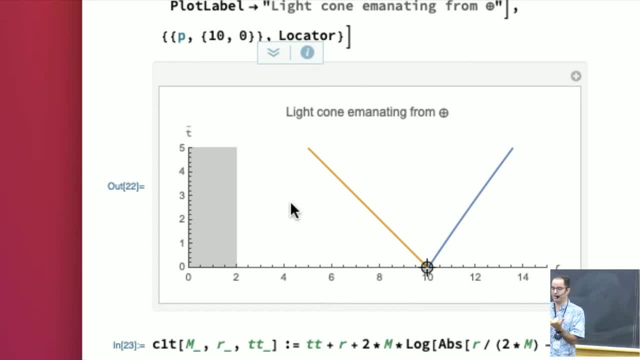 and you're throwing one light ray away and one light ray towards the black hole. So this is a space-time diagram, Our conventional R coordinate. that's basically time. Okay, it coordinates a proxy of time. Okay. so the coordinates were chosen such that they look like the traditional light cones of special relativity. 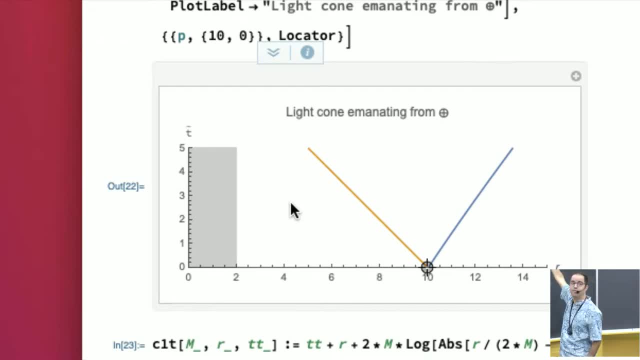 with the 45 degrees when you are far away from the source of curvature. Okay, so these are the light cones, the equation, the motion of light rays, And then this little app: here you can move your observer firing light rays. So this is the Schwarzschild radius. 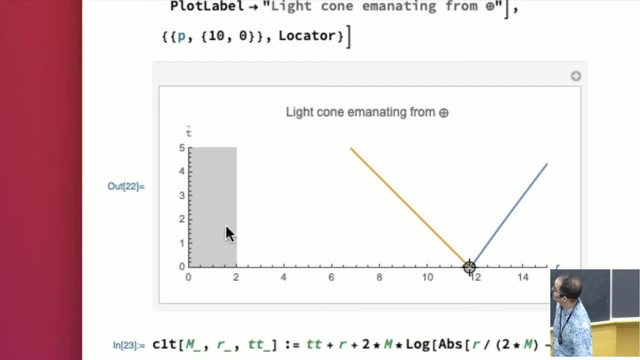 This is the realm Inside the heart of darkness, of the black hole, And what happens is as you move your flashlight, look at what happens with the light cones. Okay, you start approaching your observer, firing light rays from the flashlight. Okay, look at what happens with the light ray, the blue light ray, as you approach the Schwarzschild radius. 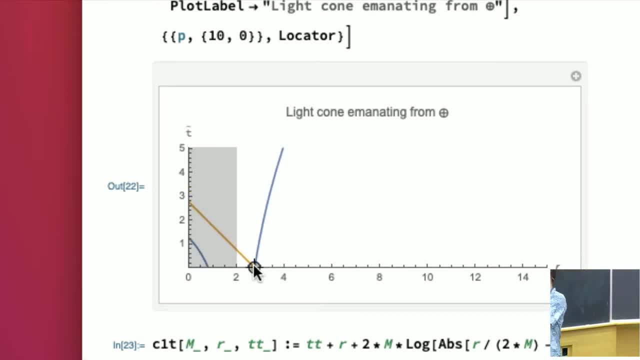 Okay, it starts moving towards a vertical line. Okay, What that really means is that it gets harder and harder and harder for the light ray to escape the gravity of the central object. Please ignore the other knowledge of that will appear here. It doesn't have a physical meaning for the purposes of this lecture. 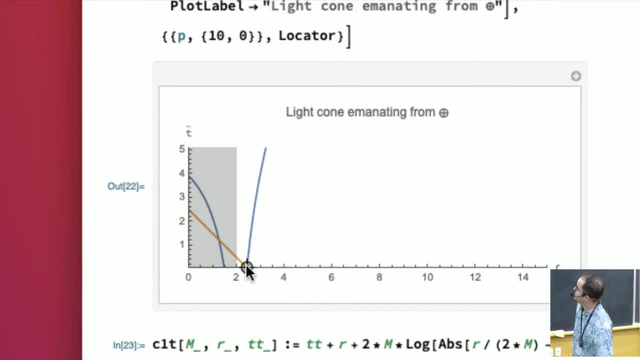 Okay, so just ignore this strange thing that is showing up there for the moment. So, as the observer is touching the Schwarzschild radius, it gets really, really hard for the light ray to escape. Okay, so just ignore this strange thing that is showing up there for the moment. 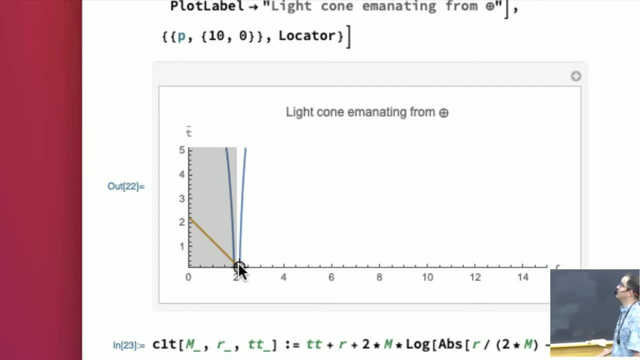 It doesn't have a physical meaning for the purposes of this lecture. Okay, so just ignore this strange thing that is showing up there for the moment. Okay so just ignore this strange thing that is showing up there for the moment. The light rays escape the gravity of the central object, but it still can't escape. 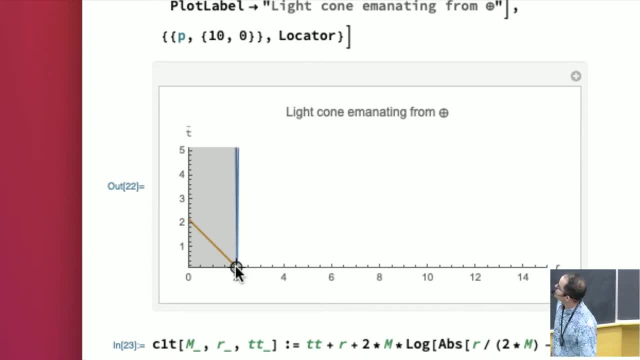 Okay, But once you touch the Schwarzschild radius, something funny happens. Okay, What happens is that you will have stationary light rays. The light rays, they will get stuck at the horizon. In fact, the surface, the surface that corresponds to the, is a null surface generated by, let's say, 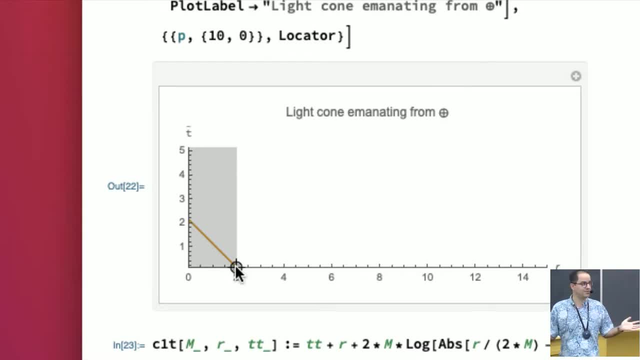 station light rays at the event horizon. okay, It's generated by the light rays that get stuck at a short radius, But then fun things happen across the event horizon. okay, Please ignore this strange thing here. I was not able to get rid of this other thing. 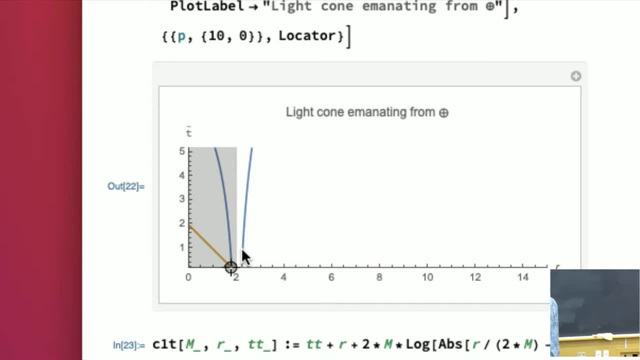 So what happens once you cross the event horizon? okay, you can still use the physics- you know nothing, as you know, nothing crazy happens inside the event horizon- But the thing is, your light rays are not able anymore to escape the short radius. okay, And once you cross the event? 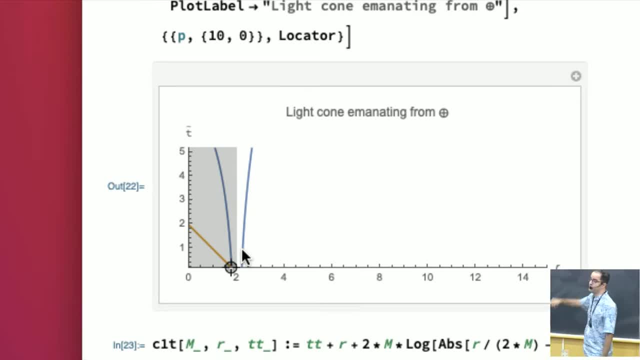 horizon. the central physical singularity- at r equals zero- is not anymore a point in space-time, but it will be a point in your time, Because at some point in the future it will be forced to cross the physical singularity, And I hope. 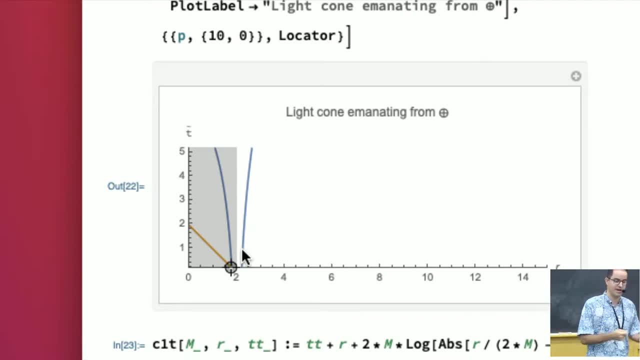 that before you cross the short radius, you sign, you know, you tell who will stay with your money once you cross the event horizon in this not-so-nice trip. okay, So again, this is what the event horizon is, you know. 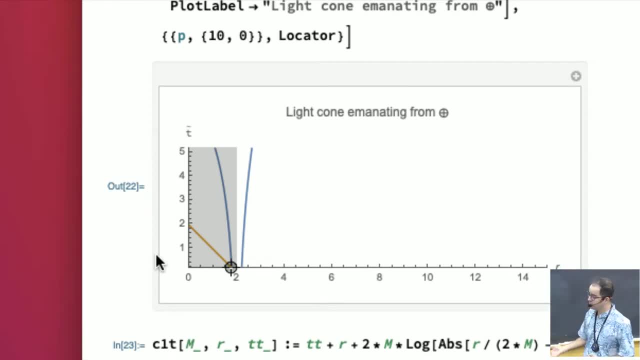 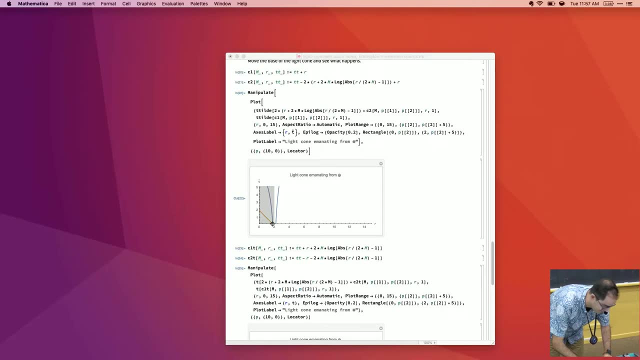 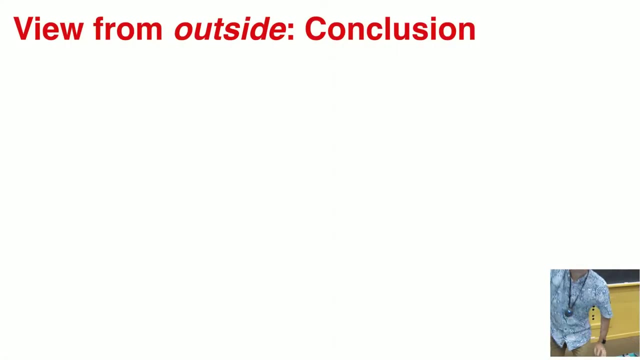 separating these two regions of space-time. And once you cross inside, well, you cannot come back. You can only cross it once. So if you fall towards the event horizon and then you cross the event horizon, nothing special will happen with you. You will reach the physical singularity. 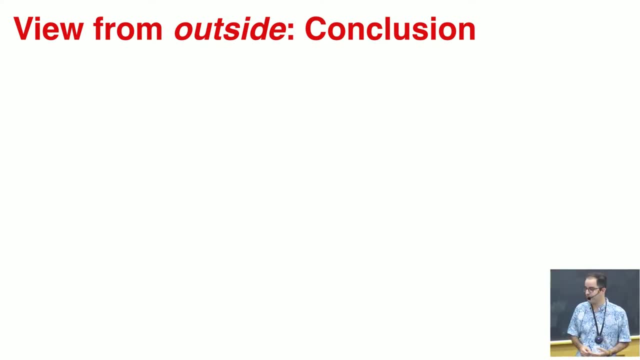 in a finite proper time in your clock. By the way, suppose you have a black hole with a mass of solar mass, okay. And suppose you are a very courageous explorer and cross the event horizon. This black hole? we are not sure, probably this kind of black hole is not. 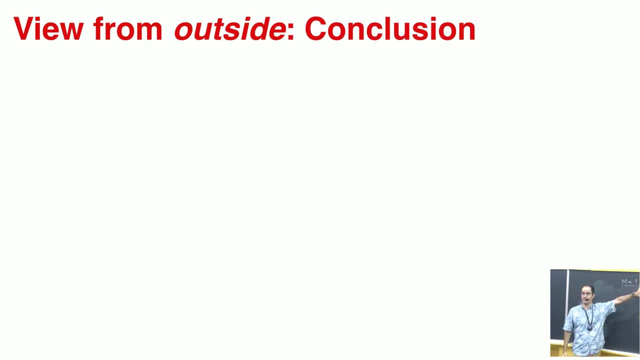 you can't form this kind of black hole in nature. okay, This is a kind of astrophysical black hole, because it will always be some kind of pressure that will be able to support a gravitational collapse for this kind of low masses. But suppose you cross the event. 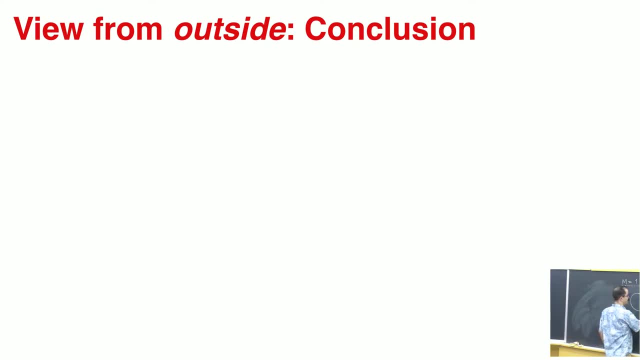 horizon of such a small space-time and you cross the event horizon size, black hole, OK, And then you will be forced to collapse to this physical singularity at r equals 0.. Do you fast? it will fall towards the physical singularity according. 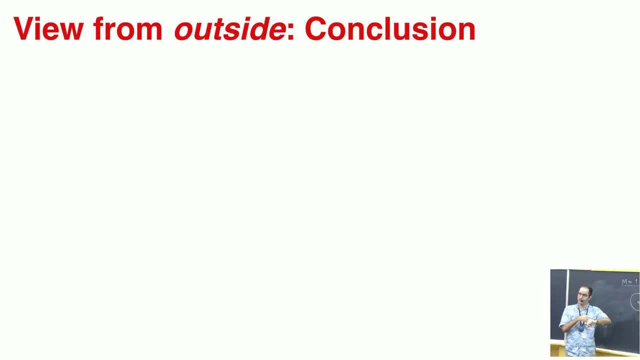 to the proper time measured in your clock. How long will it take to fall once you cross the event horizon? OK, I will give you a couple of options here. 10 seconds, one second, and let's see why not, Why not? 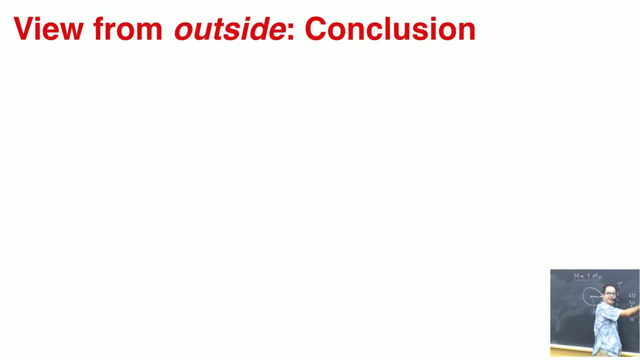 So who thinks that it will take one minute to fall? Can you raise your hands In the frame of falling, Falling towards the central singularity, once you cross event horizon in your frame? in your frame, How long will it take? You think it's one minute, right, Fabio? 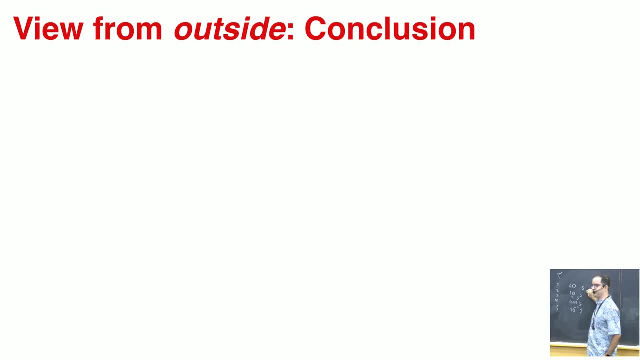 No, nobody thinks it's one minute. Some of you probably did this calculation as part of GR course, but it's fun to remind you 10 seconds One. The radius is it's a 1.5, sorry, 1.5- kilometer. 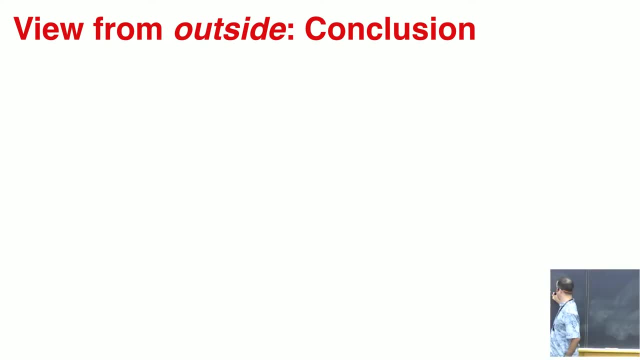 Yeah, So 10 seconds. who thinks 10 seconds? Nobody, One second, Nobody. 0.01 seconds. Everybody's leaping probably OK. So let's see 10 to the minus 5 seconds, why not? 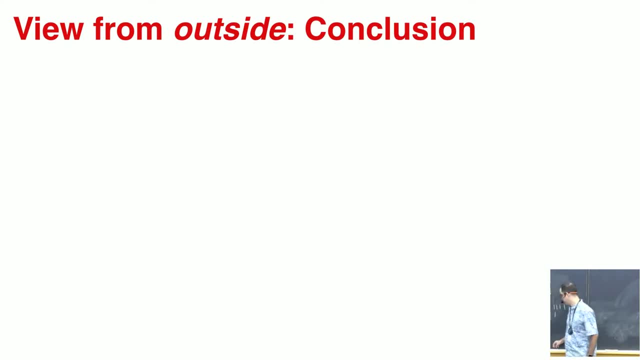 One hand: OK. So, guys, it will take 10 to the minus 5 seconds for you to fall once you cross event horizon to reach the central singularity. OK, 10 to the minus 5 seconds If it's a 1 million solar masses black hole. 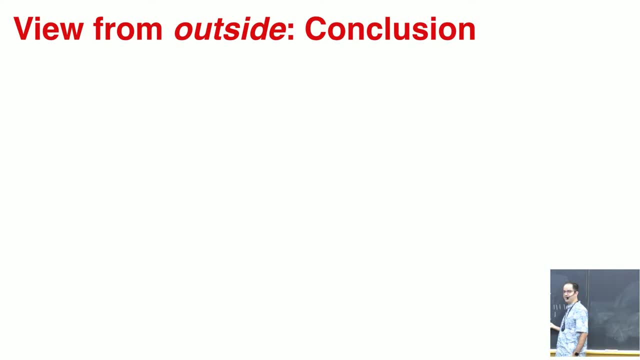 it will take you about one second. OK, If it's a 100 million solar masses, it will take you a couple of minutes to fall towards the central singularity. OK, so gravity is strong. OK, These guys are very. things happen fast. 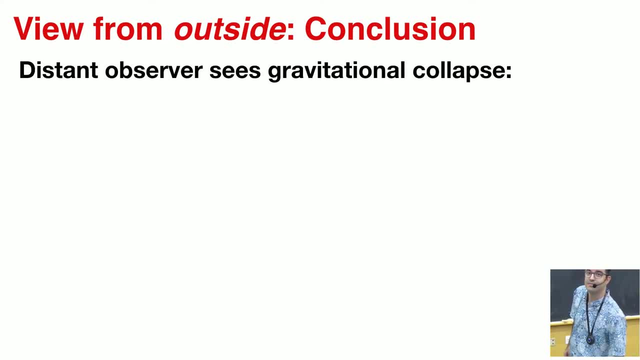 It is supposed to be the back of the envelope calculation. You can do this calculation using the static space time. OK, So the back of the envelope calculation is trivial. 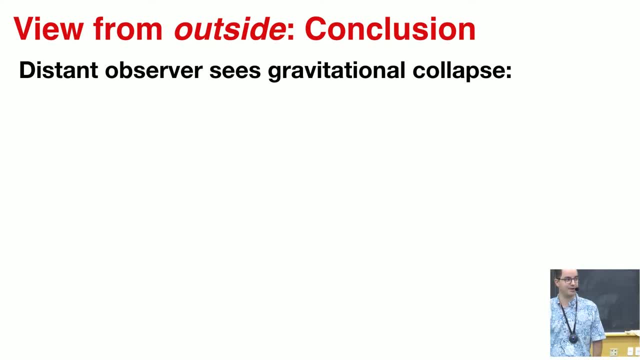 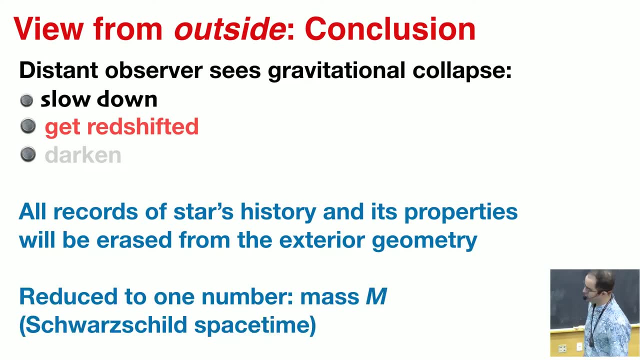 but the fun thing is doing the actual calculation of the proper time to reach the singularity Anyway. so if you are an observer sitting outside of a black hole, OK. once a star collapses towards a black hole, all records of the star history. 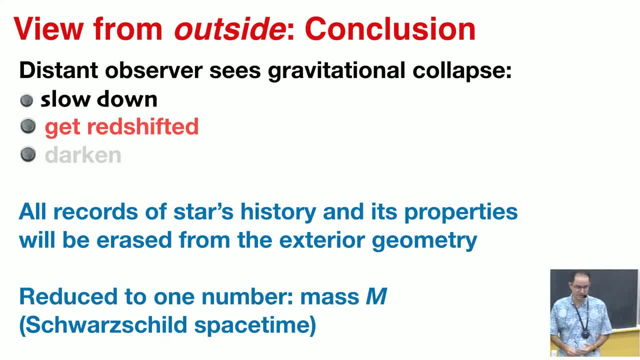 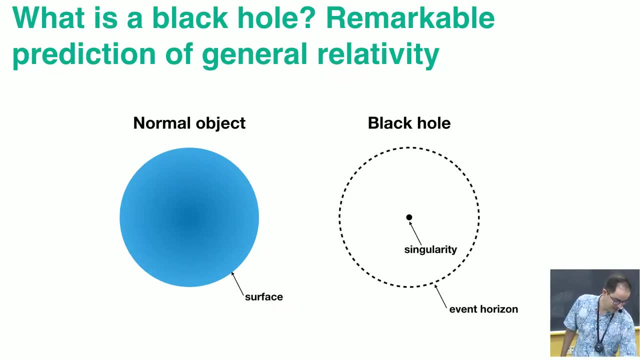 will be erased for an external observer, OK, And everything will be reduced to one or two numbers, depending on the angular momentum, the mass and the spin, according to an external observer, once the star crosses its event horizon. So what is a black hole? 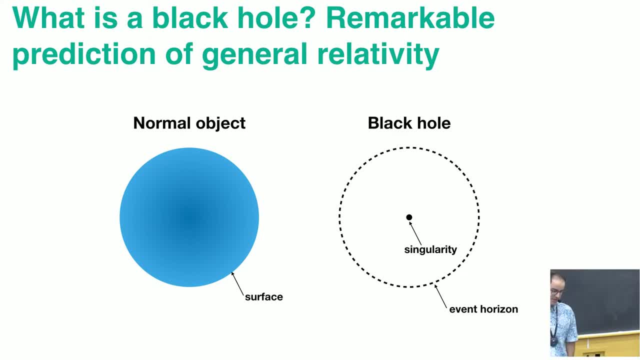 A black hole is a remarkable prediction of relativity, In the sense that it such that not even light can escape from its gravitational attraction. And so you have this, And at the center you have the physical singularity. The event is a one-way membrane. 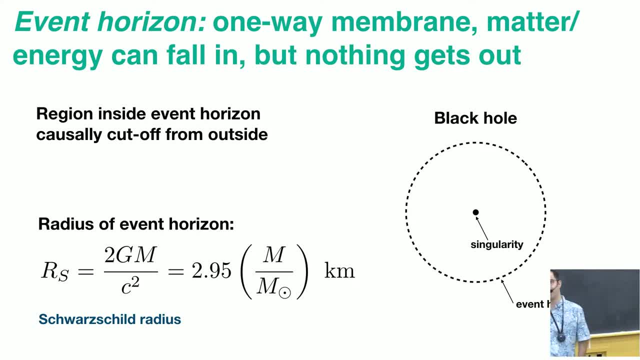 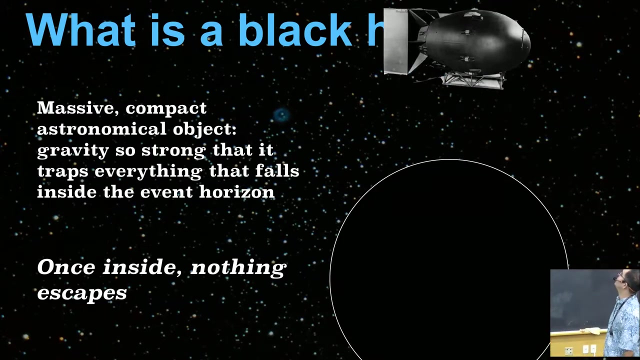 So matter? energy can fall in, but it can never get out, at least with classical process. It's about three kilometers. three kilometers, if you could, for solar mass, black nature, OK. so So if you take a bomb with a timer, a bomb of 100 megatons, 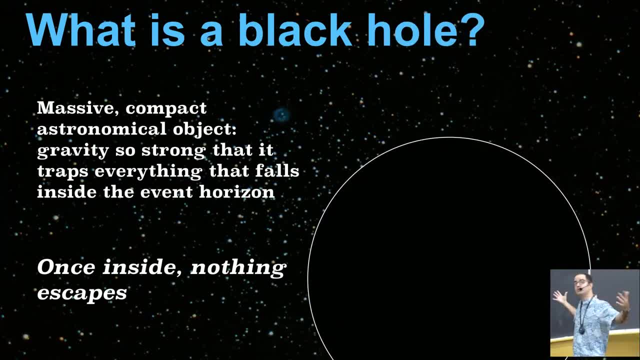 and you throw it inside a black hole. OK, it explodes inside a black hole, but you will never see the explosion happening because- and the light get trapped inside event horizon and event horizon will grow a little bit, The area of the black hole will grow a little bit once. 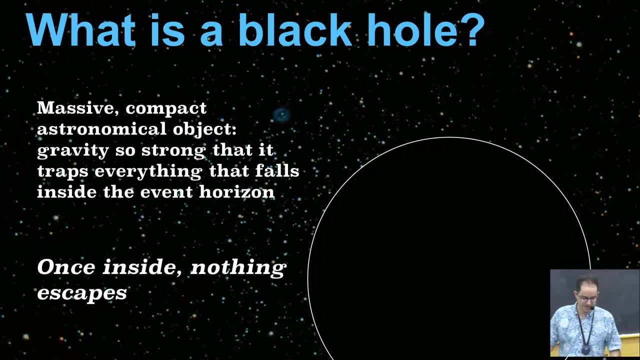 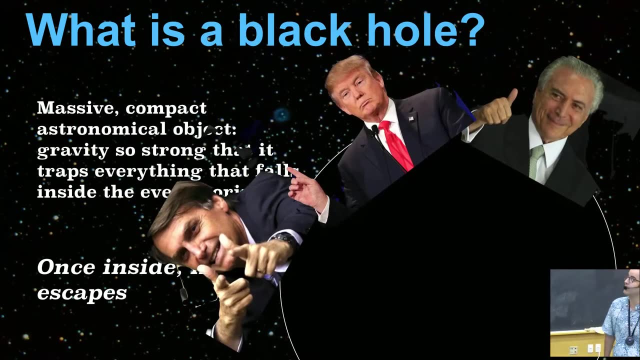 it accretes because its area increases a little bit. Then you take other things, not necessarily very pleasant, and then you throw inside a black hole. its area grows a little bit more, Then you take further unpleasant things and you throw inside a black hole. 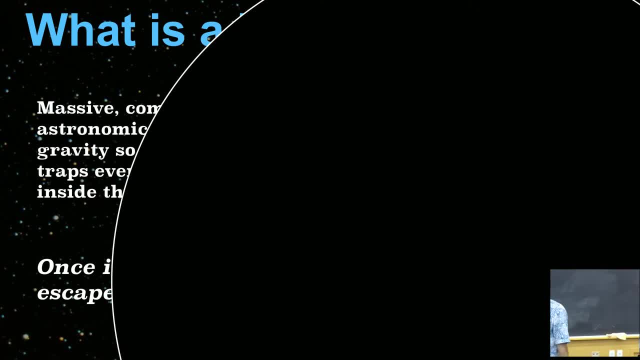 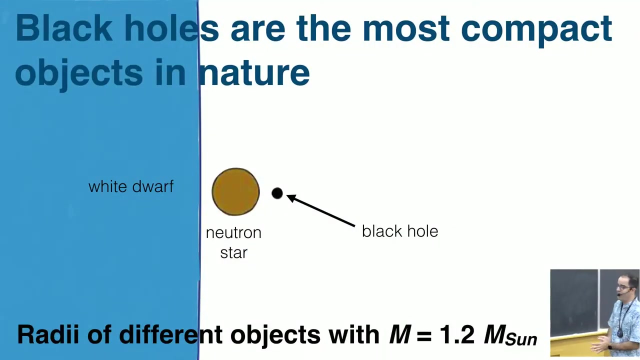 And in this case it grows really a lot And it And it keeps growing. OK, So the mass of the black hole will always increase. when you are classical things to the event horizon, classical processes, For you to have an idea of how compact black holes are. 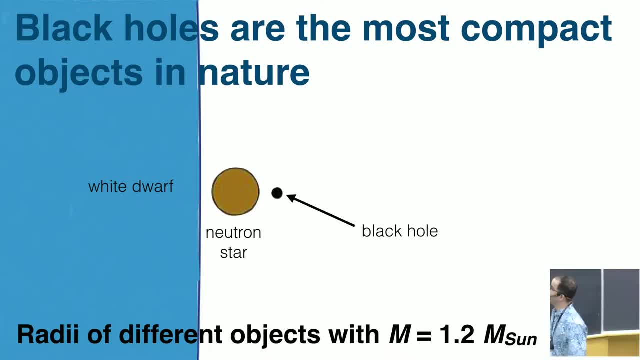 compared to other kinds of objects. this is a simple diagram comparing the size of the event horizon To the size of a parable, to the size of a typical white dwarf, to the size of a neutral star, then a black hole. all of them with the mass shown. 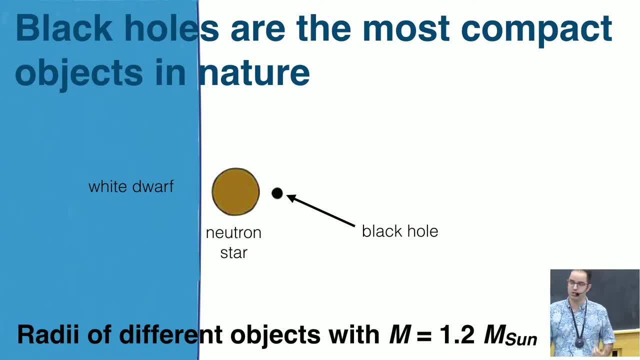 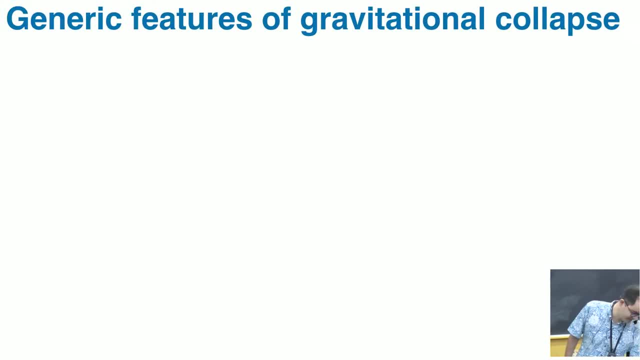 Black holes are the most compact objects that nature can form And therefore they have the most extreme gravity. having this cool in these three weeks, I think I can skip these generic features of gravitational collapse. So, as I said, if you keep feeding a black hole, 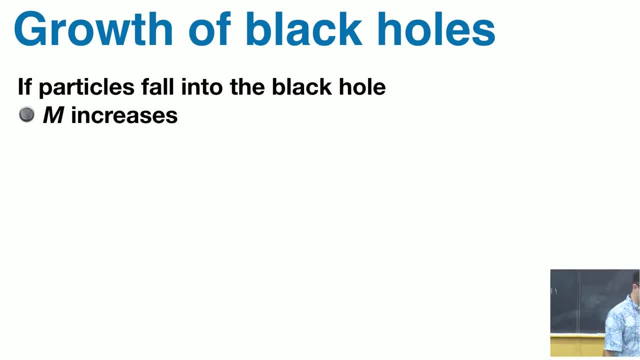 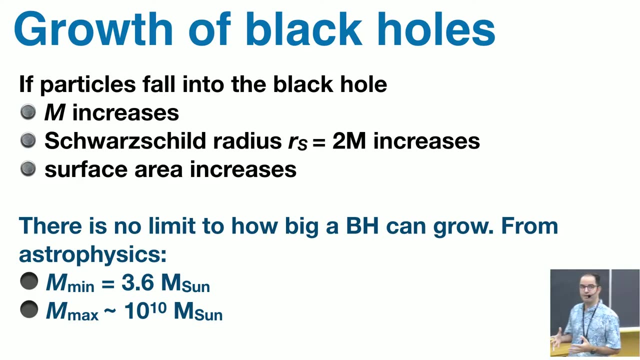 with particles. the mass of the gradually increase. It's should radius will gradually increase. because the mass is increasing, The surface area will increase. So in principle there is no limit to how big the mass of a black hole is. OK, in principle. 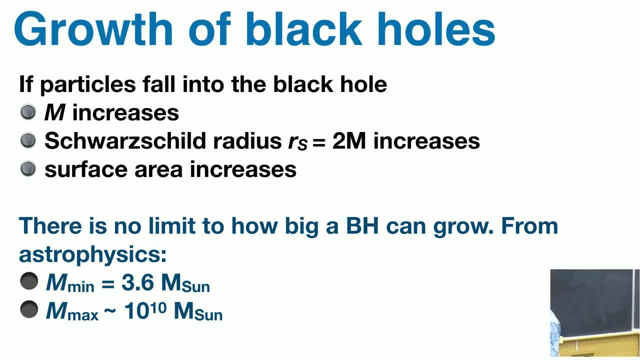 If the universe wants to keep feeding the black hole, the black hole will be happy. It will not give you anything. It might give you some things in return, But it will happily grow as you keep feeding the black hole. So we have measurements of the mass of black holes in nature. 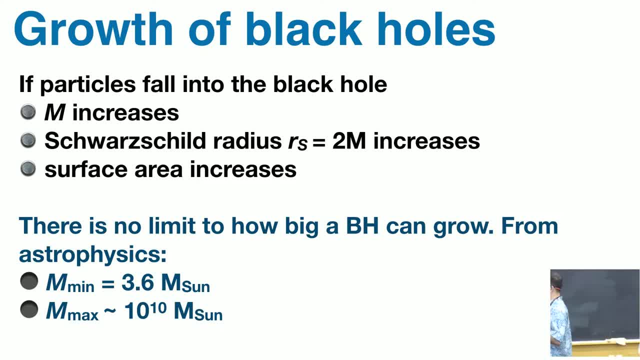 So it seems like the smallest weight, the smallest mass that we make for a black hole in nature, in a stellar mass, in a system called x-ray binary. it's around four solar masses. OK, And so far the record-breaking black hole that we measured. 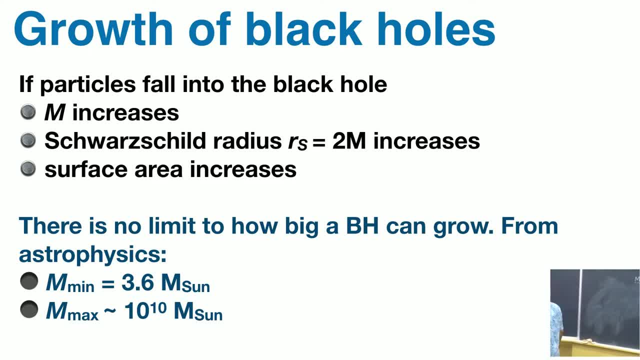 we estimated the mass sits in the center of a distant galaxy with a record-breaking mass of. Is this audio, or is it my impression? It's a bit intermittent, right? Maybe I'm doing something that I shouldn't do here. 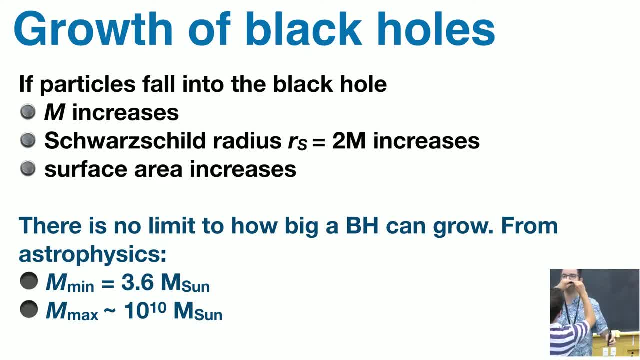 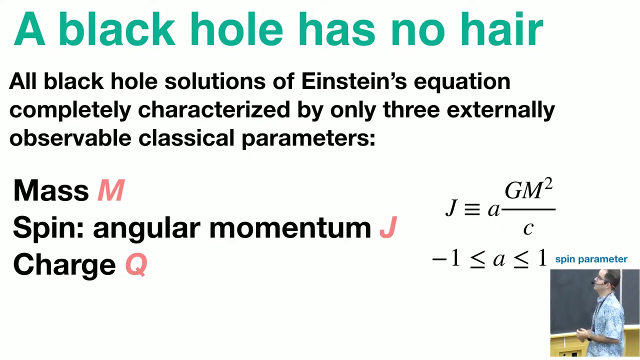 Okay, Can you hear me? My apologies for the intermittance. So, as you know, a black hole has no hair. So apparently for dynamical space times, the no hair theorem is a bit more complicated than I thought, as we learned with Ian Steinhoff. 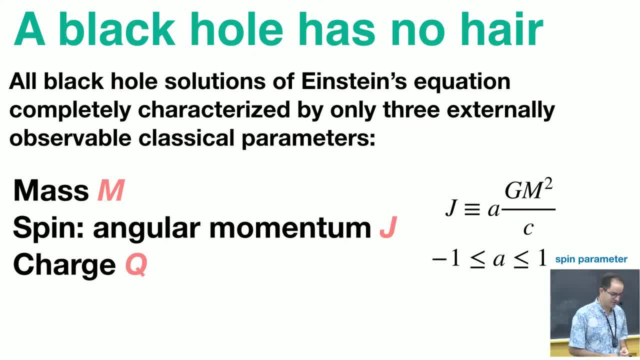 So all black hole solutions of Einstein's equation are completely characterized by the only three parameters: the mass, the angular momentum and the charge We use. as you might know, we characterize the so-called spin parameter of Kerr black holes Between minus one and one. 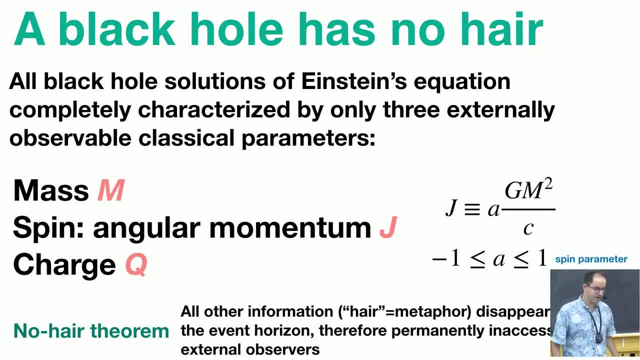 The no hair theorem assures that if you try to add properties to the event horizon, in other words, if you try to add hair to the event horizon, the black hole will get rid of the hair, keeping the exterior geometry characterized by only these three numbers. 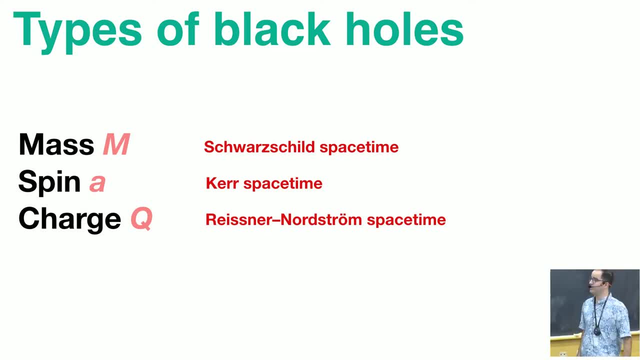 The three numbers lead to different kinds of space-time geometries: The Schwarzschild space-time, the Kerr space-time and, for a charged black hole, the Reiner, Eisner, Nordstrom space-time. But it seems that if you try to add charge to a black hole, 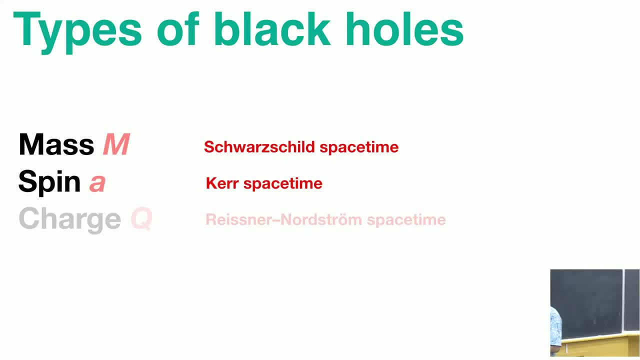 the black hole will very quickly attract a pulse charge and nullify its charge. okay, So it seems that in astrophysics you cannot have black holes with significant amounts of charge because they get discharged very quickly, okay, So, no, People don't really consider charge. 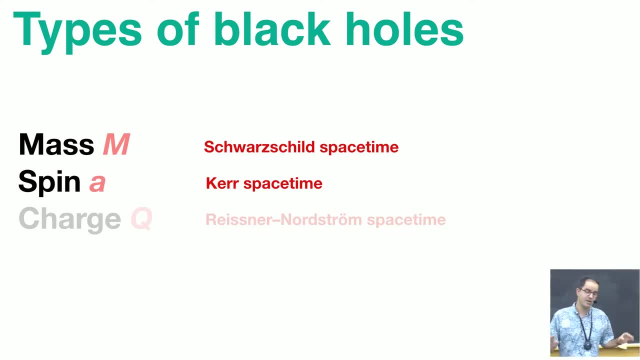 to be an important parameter for astrophysical black holes: gravitationally significant amounts of charge. So from now on, when we talk about astrophysical black holes, we will only consider mass and spin as the fundamental parameters. So we will have the Schwarzschild black hole solution. 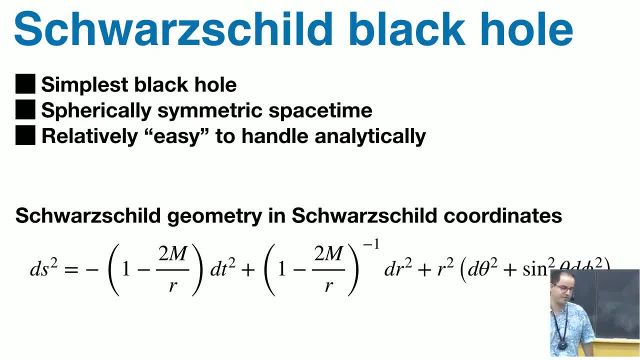 the first more or less simple solution of the Einstein's equation for a spherically symmetric geometry around a spherically symmetric object. okay, It's the simplest black hole. It's relatively easy to handle analytically. Of course, it depends what you want to do. 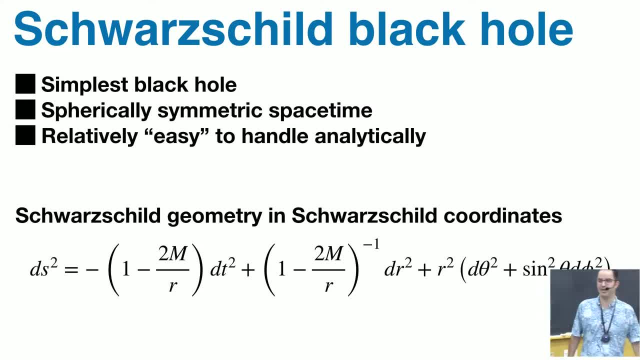 If you try to derive the precession of the perihelion to first order, you will realize it's not that easy to do this calculation which is supposed to be. it will take you, it will be a bit tricky to do that calculation. 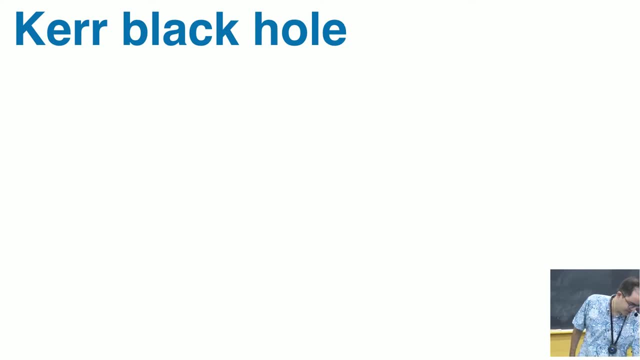 And then we have the Kerr black holes. okay, Kerr black holes, Kerr black holes. they are expected to be the norm in the universe for the simple fact that angular momentum conservation, angular momentum cannot really disappear. So if you have a collapsing star with some angular momentum, 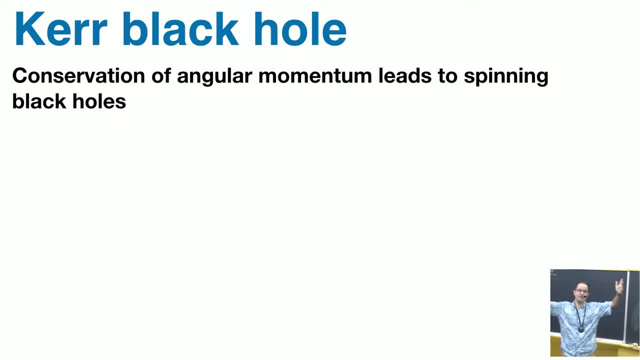 it is getting smaller, smaller, smaller, like a ballerina or a bailarino. you know it's spinning and then blows your arm. You spin faster. angular momentum cannot disappear, okay. And then if you have a spinning star, that collapses. 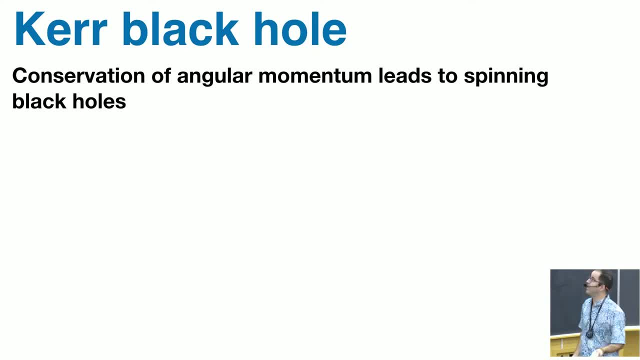 you will gather a black hole with angular momentum, the Kerr black hole. Of course, deriving the solution was not that easy. the first derivation by right care. That's why it took about 50 years after the short-shoot solution for him to obtain this. 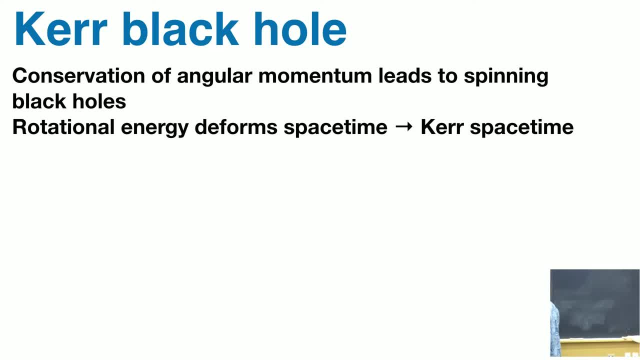 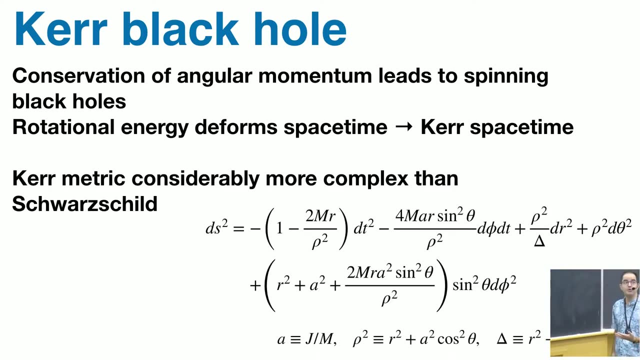 And the interesting thing is that you have an extra degree of freedom, that you have rotational energy, which also distorts The space-time around the black hole. okay, So this gives rise to a very interesting and very rich exterior geometry characterized by the Kerr space-time. okay. 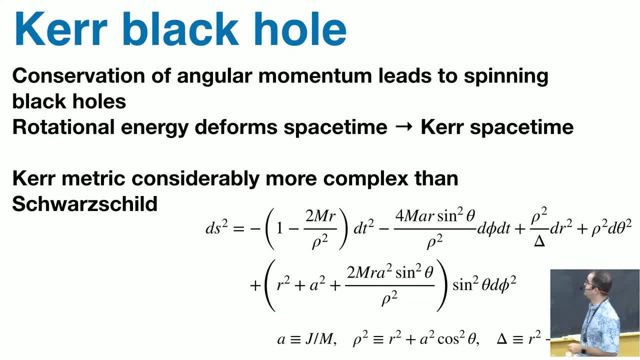 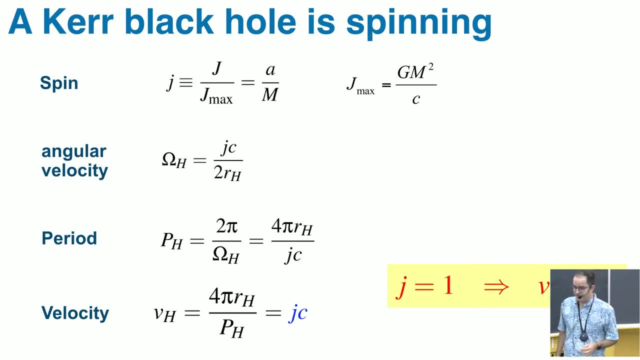 The expression is a bit more complicated than the expression for the short-shoot space-time. You have a. it's convenient to write this rho and this delta and then you have this thing here And a Kerr black hole can really, you can really understand. 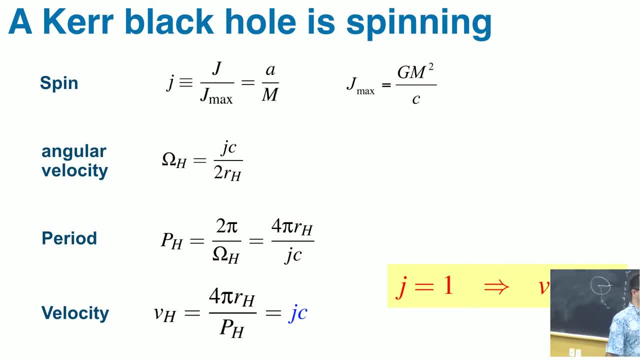 as a spinning object. okay, It's a spinning space-time, It's a bit more complicated than simply a spinning object, but you can really treat it as a spinning, let's say, ellipsoid. The space, the horizon has the shape of ellipsoid. now 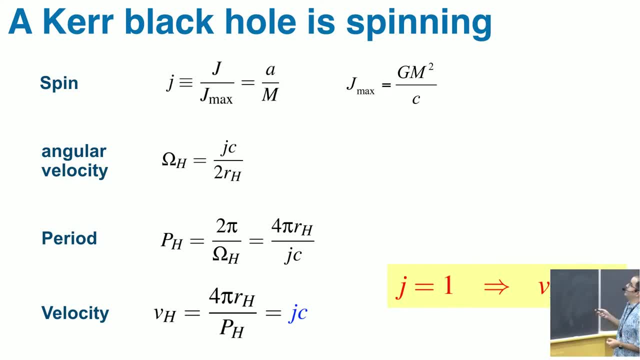 You can think as a rotating membrane which has spin. okay, for the maximal spin which is here, I call j equal one, the rotational velocity of the horizon is the speed of light. And if you could add angular momentum to a Kerr black hole, 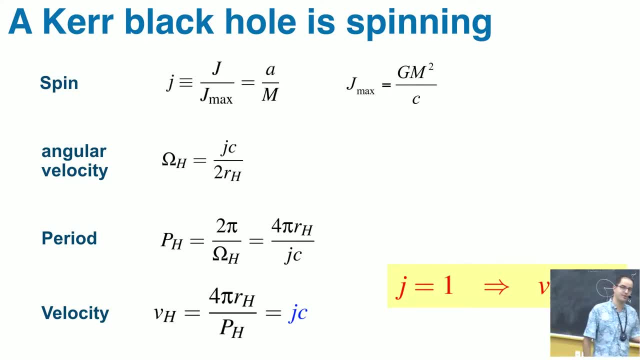 above the limit of j one, it will break the event horizon and then it will form a naked singularity. But so far people have tried to destroy event horizons and nobody was able to destroy and add overfeed with angular momentum of black hole. 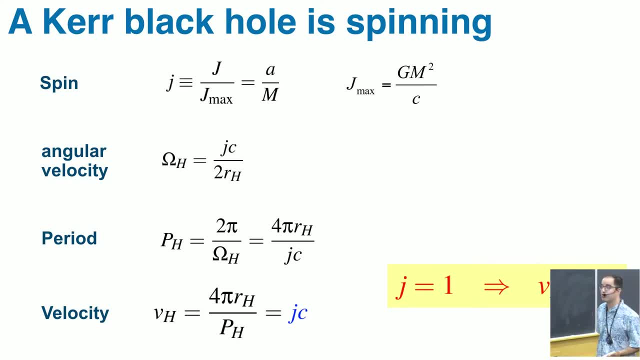 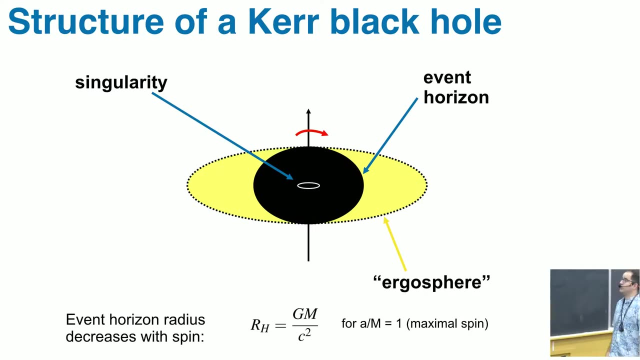 and reveal the naked singularity with calculations. People are trying, but it's very hard. So you can characterize the spinning event horizon with an angular velocity, with a period, with the velocity at the equator. This is the resulting structure of a Kerr black hole. 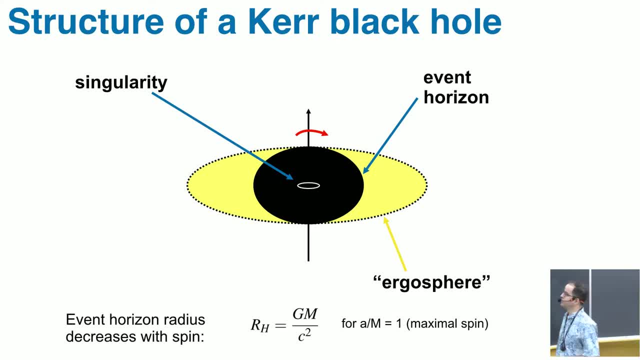 So you have more than one event horizon? okay. You have then the event, the traditional event horizon. okay, You have the traditional event horizon, but you also have inner event horizons which are not really relevant here because they are inside the traditional event horizon here. 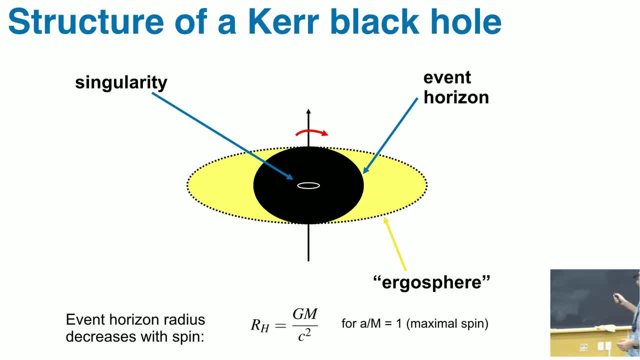 So they are. we don't need to really work with them. So, besides the ellipsoid, the ellipsoidal shape of the event horizon, which is a rugby ball- okay, It's like it looks like a rugby ball- You also have the so-called I'm using this laser. 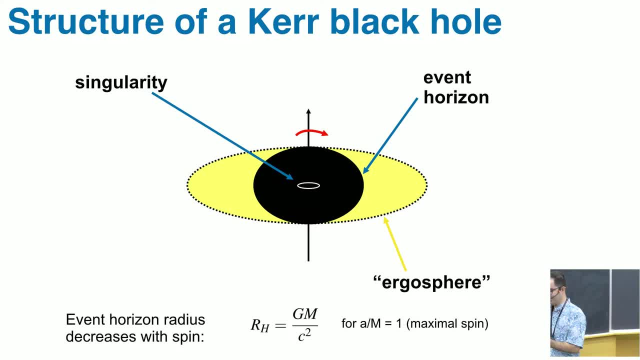 but it's not really working, so I don't know why I'm pressing this. Oh, is it true? Oh, wow, Thank you. So, yes, great. So then, besides the ergosphere, okay, So the ergosphere is a region close to the event horizon. 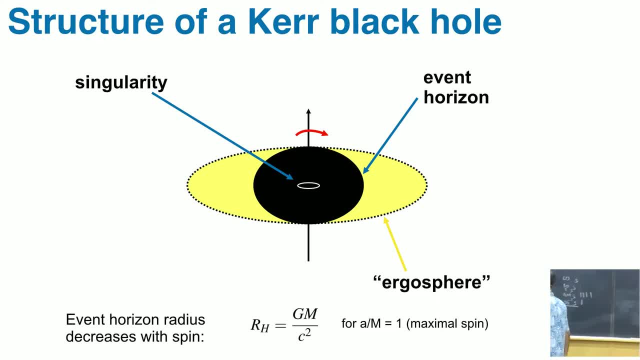 where you cannot have static servers, okay. So if you approach the black hole and then you get inside the ergosphere, what is happening here is that the black hole is dragging the space. the spinning black hole is dragging space around with it. okay. 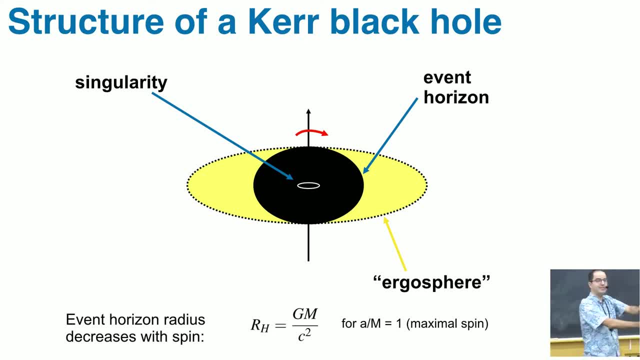 So if you get close, if you get in the ergosphere, it will be forced to co-rotate the black hole, because space is being dragged with the black hole, a phenomenon called frame dragging. Oh, and also another fun thing is that the singularity. 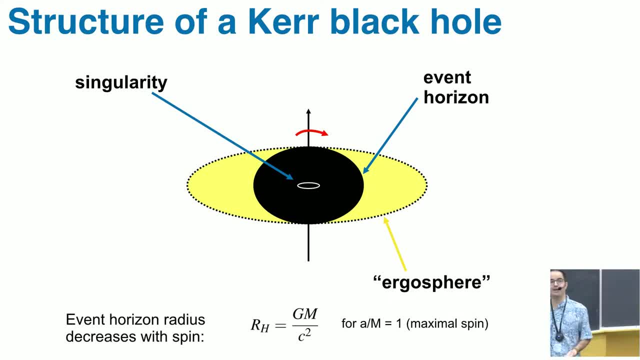 the physical singularity is a ring. because can you understand a point particle with angular momentum in classical physics? Okay, If it's spinning, the central singularity also has to spin. But can you define in classical physics a spinning particle? It's tricky, right. 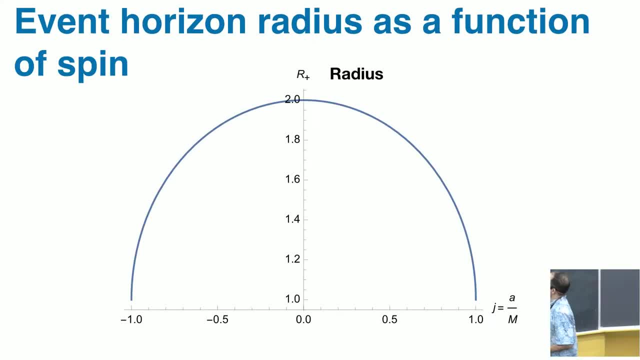 So the singularity is a ring. So this is the size of the radius of the event horizon as a function of spin. So for spin equals zero, we recover the short-shoot radius. For maximal spin, the event horizon shrinks to half the radius of the short-shoot radius. 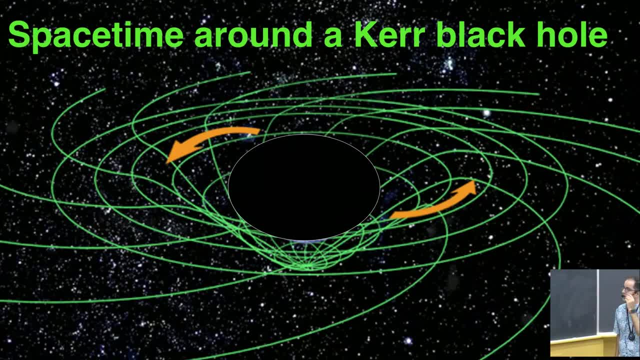 And this is what I mean by frame dragging. okay, So we can imagine: if you try to build an embedding diagram for the space-time around a black hole, it's dragging space, it's dragging observers. This is what the space-time geometry looks like. 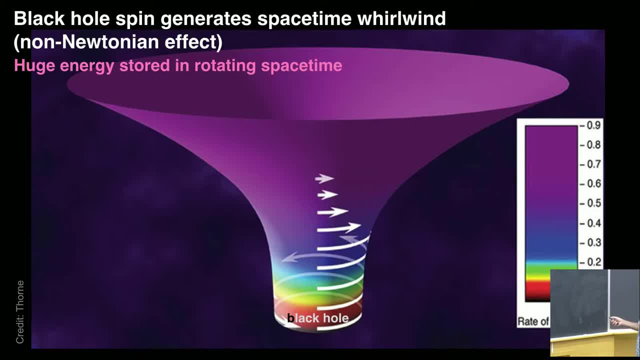 around a Kerr black hole. Here is the frame dragging effect. The space-time around the black hole has a huge amount of rotational energy stored in the space-time And if you are smart you can extract that rotational energy stored in the space-time around the black hole. 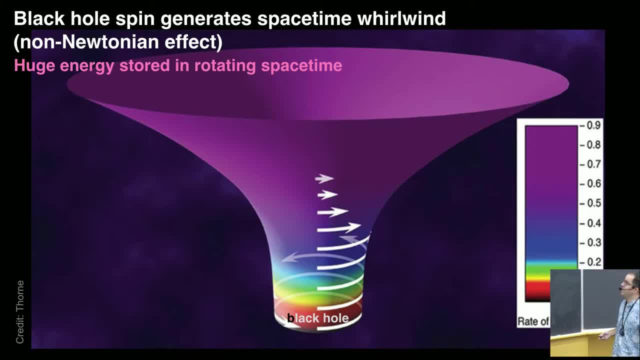 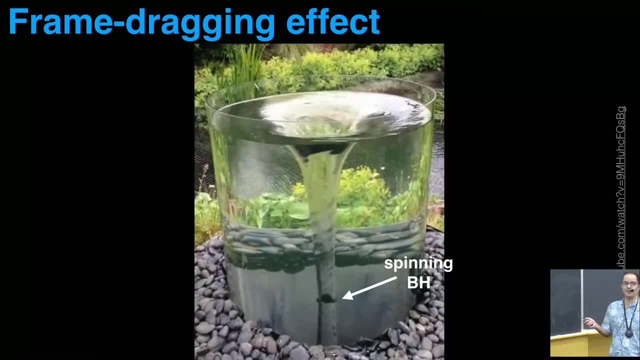 So I like this analogy to understand what is happening around a Kerr black hole. If you go to one store, I don't know where you can buy this sort of device for your garden. if you are a millionaire and you have a huge garden. 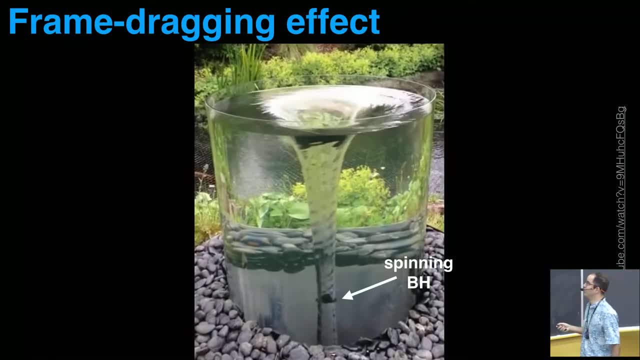 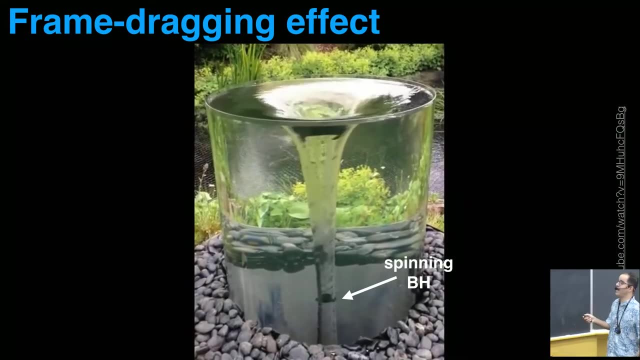 and then you can buy this kind of device here. So this is a metaphor for the distortion of space-time around a Kerr black hole. Imagine that this is a kind of embedding diagram for the geometry. Imagine you have a Kerr black hole sitting there. 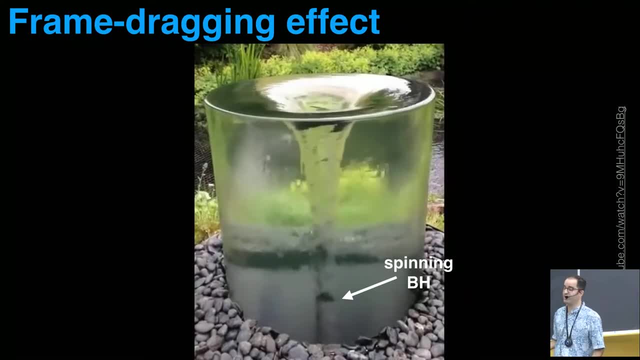 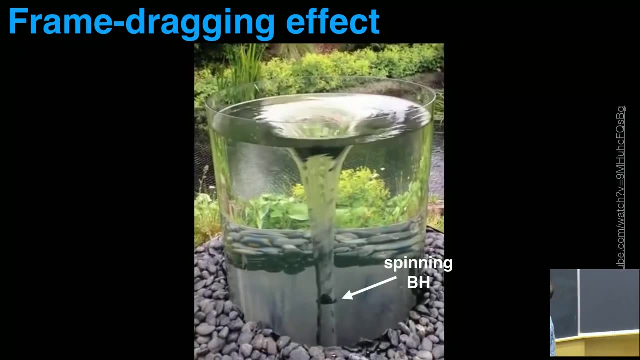 and imagine that in this metaphor, the water represents space-time. okay, If you drag an ant here, the ant will be forced to co-rotate with the water. In this metaphor, if you drag an observer, the observer will be forced to co-rotate. 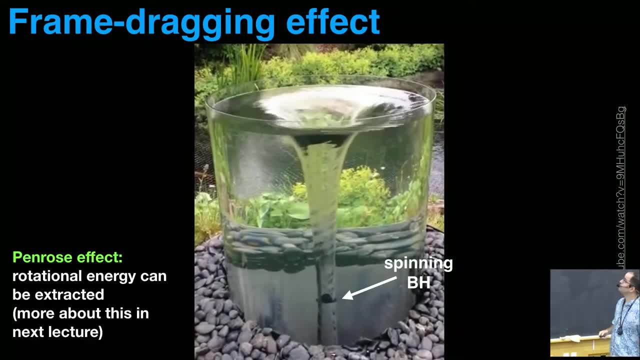 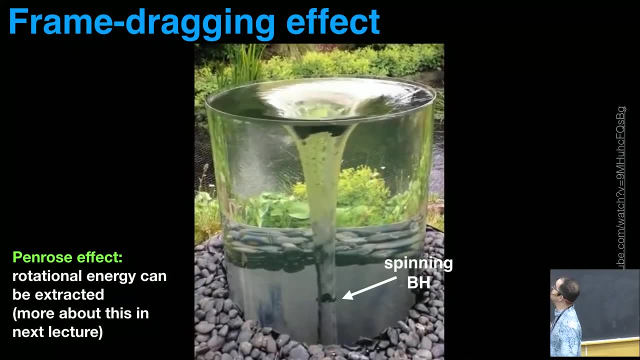 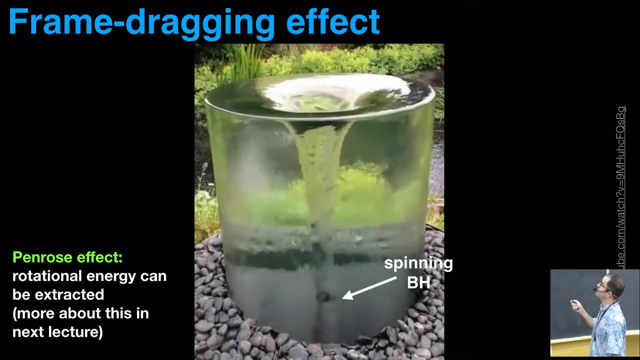 with the rotating space-time of the black hole. In fact, in the 60s, Roger Penrose, he thought of a smart way of using particles and destroying things in the ergosphere of a spinning black hole to try to extract some of this rotational energy. 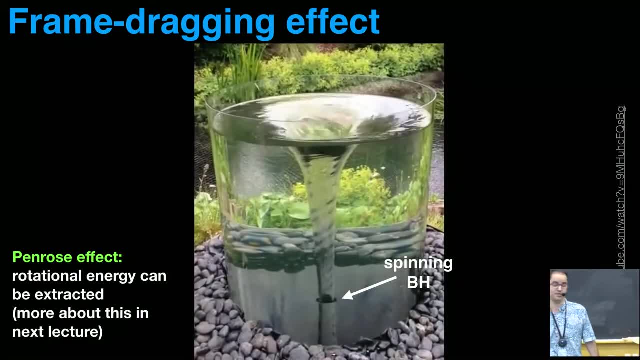 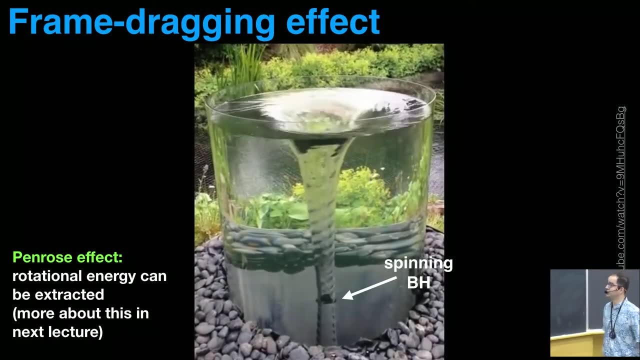 the free energy and power of the physical processes. This is called Penrose effect, the process of extracting, trying to extract the rotational energy of space-time of a Kerr black hole with astrophysical processes. And it turns out that the original Penrose process 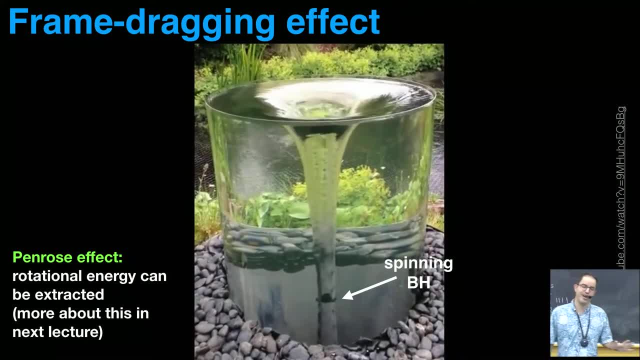 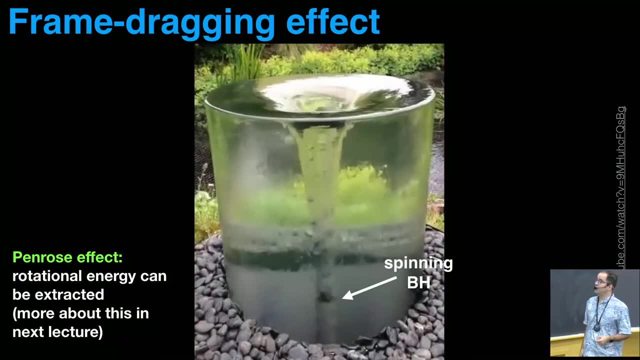 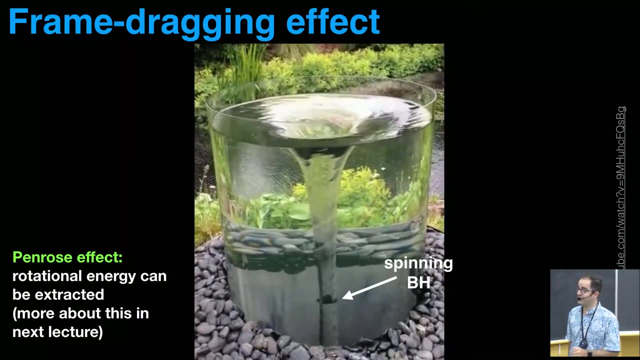 is not viable. It's very hard to extract this rotational energy with the original Penrose process proposed by Roger Penrose, But it turns out that you can still extract the rotational energy of the black hole with other things which I will mention in the next lecture. 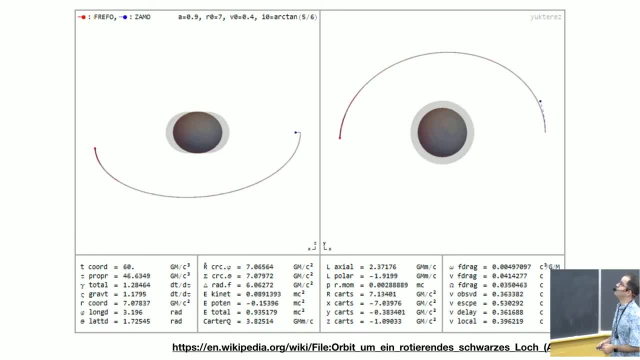 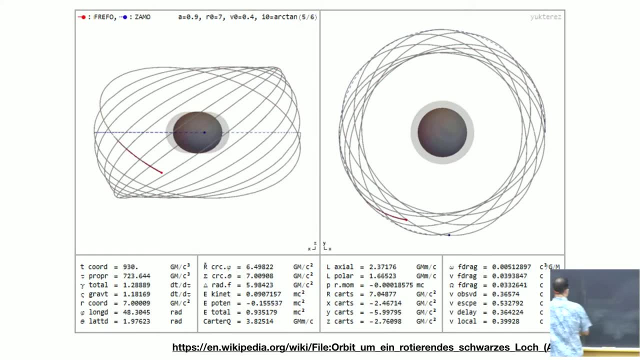 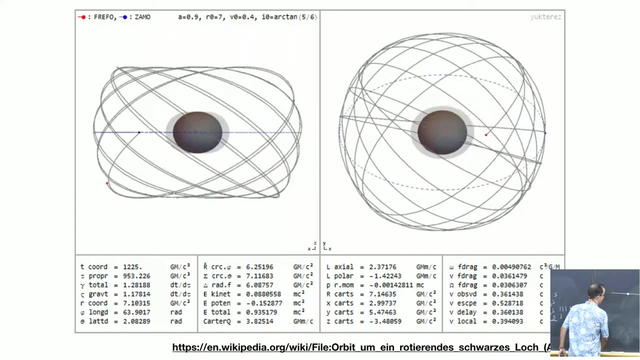 Orbits of test particles are way more complicated- around a Kerr black hole, Around a Schwarzschild black hole. if you throw a particle on a Schwarzschild black hole, it will always be able to define a plane. The particle will be stuck in a plane. 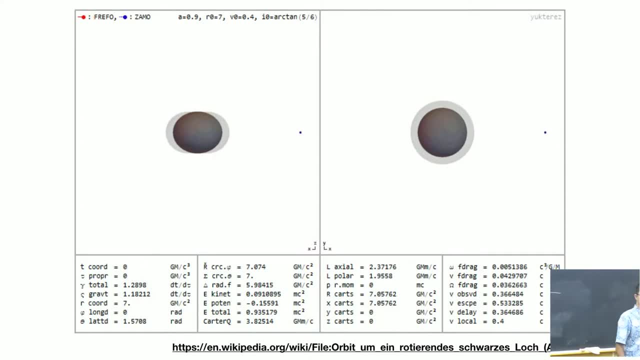 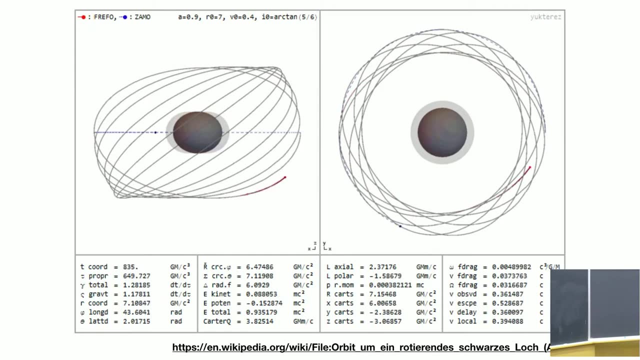 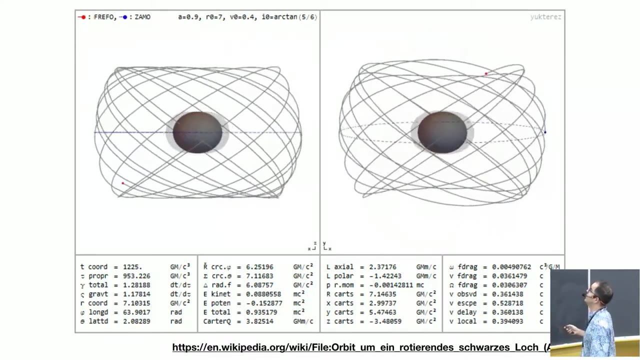 just like the Newtonian problem, the two-body problem in the Newton's mechanics. But in the Kerr problem this is way more complicated because the space-time has less symmetries than the structure of space-time, So orbits are more complicated. This is an example of a time-like orbit. 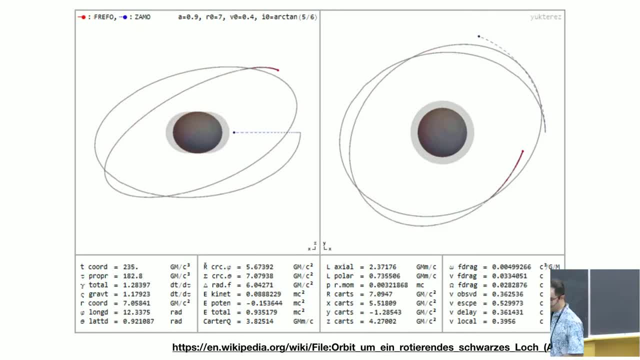 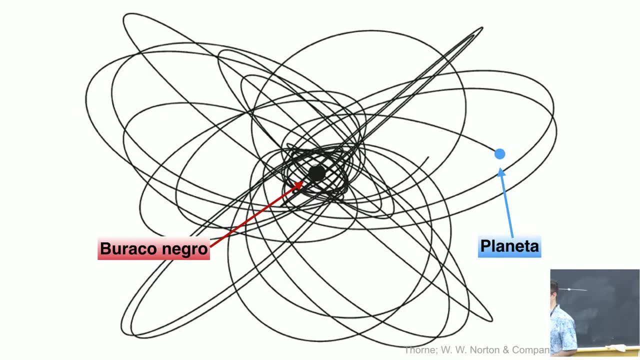 of a particle with some initial conditions. So if you were able to sustain planets around a Kerr black hole like Christopher Nolan and Kip Thorne proposed in their Interstellar movie- I wish there was a second movie of Interstellar- The orbit of your planet will be quite tricky. 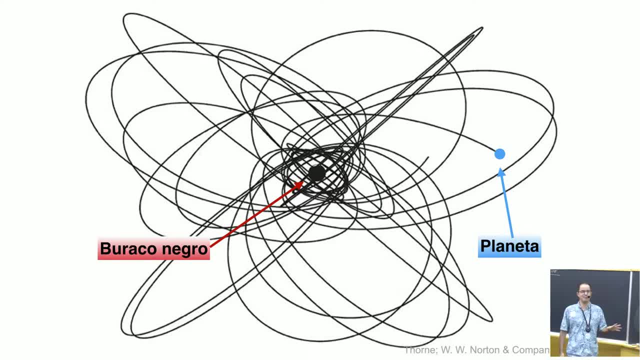 quite complicated. I don't think it will be pleasant to live in a planet orbiting a Kerr black hole. The weather will be really interesting as the planet crosses several times the equator of the accretion disk. So I really would not like to live in such a planet. 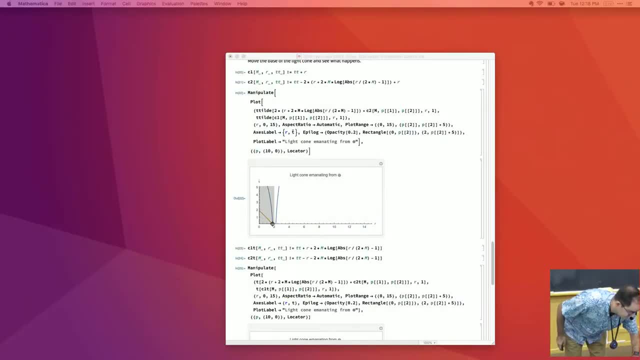 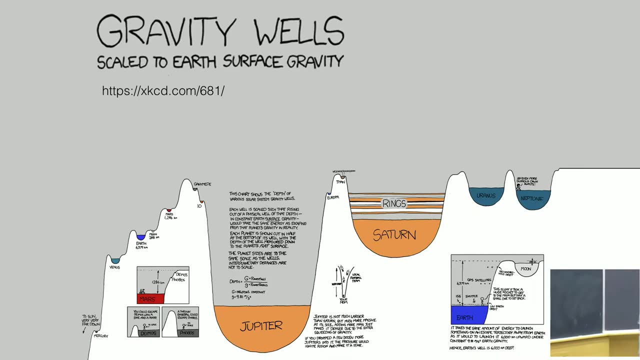 Finally, finally, to wrap things up about this very broad review of black holes in GR. I really love this graph, this cartoon made by the XKCD guy, the guy who draws the XKCD series. I don't know if you are familiar with XKCD. 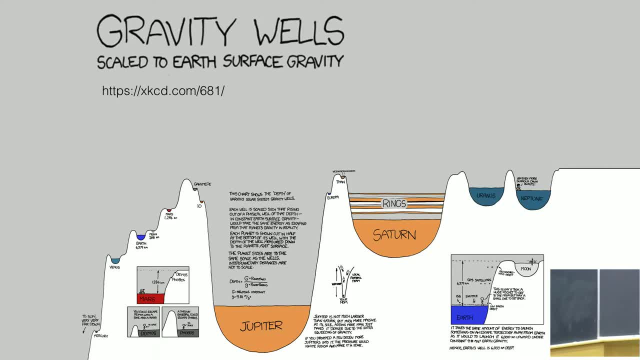 But this is a way of representing how extreme the gravity of a black hole is in the universe And this is a very nice way of visualizing the gravity with the potential wells. the potential wells Here, these are the potential wells of planets in the solar system. 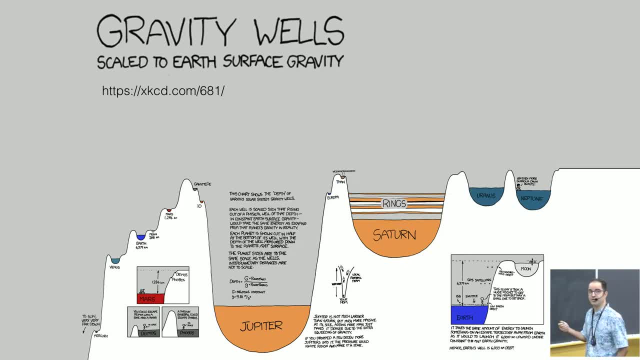 So the corresponds to this gravity of the different planets in the solar system. Here you have Mercury, Venus, Earth, Mars, Jupiter, okay, Saturn, blah, blah. Herculobus, planet Herculobus- There is a crazy guy here in Sao Paulo. 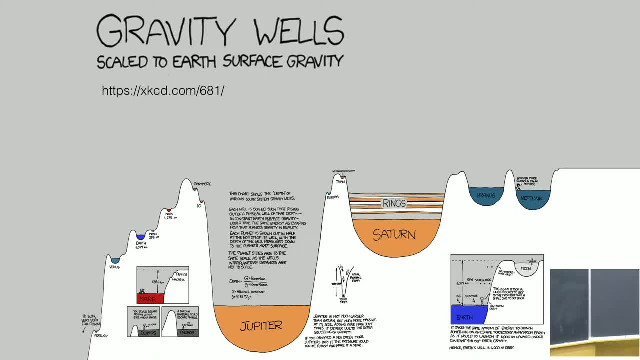 who goes around putting signs on everywhere about some fictitious planet called Herculobus. I hope this is only in Brazil and not in Argentina and other neighbors, okay, So Herculobus, the fictitious planet, is somewhere down here. 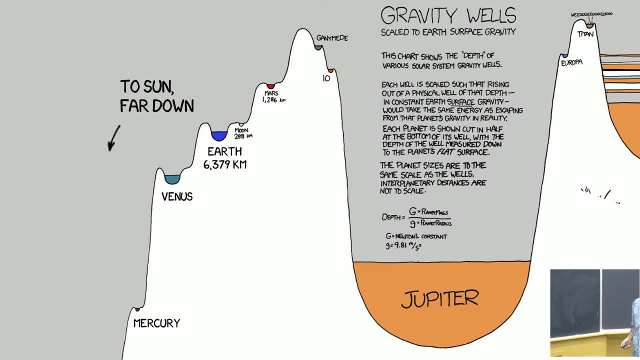 Okay, Right, So let's imagine for fun that the height of the potential well for Earth is one meter. okay, So more or less one meter. Imagine that the gravity of Earth is such that its potential well, let's make an analogy. 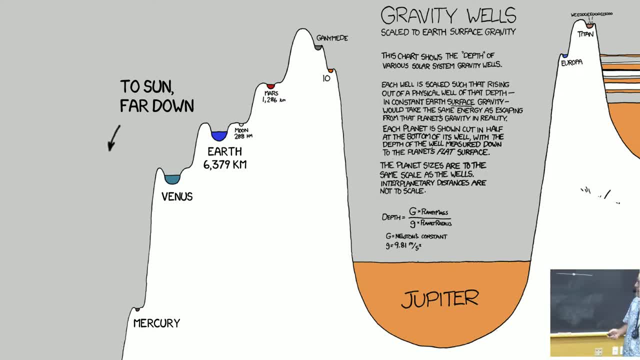 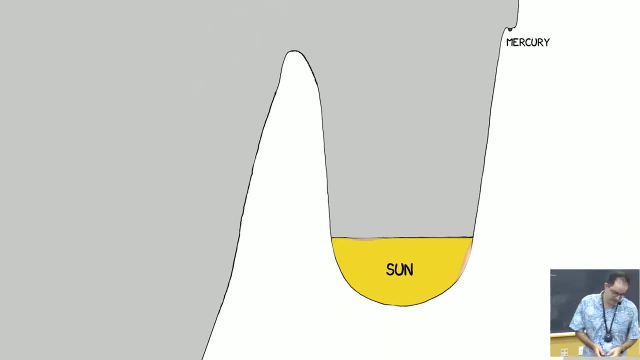 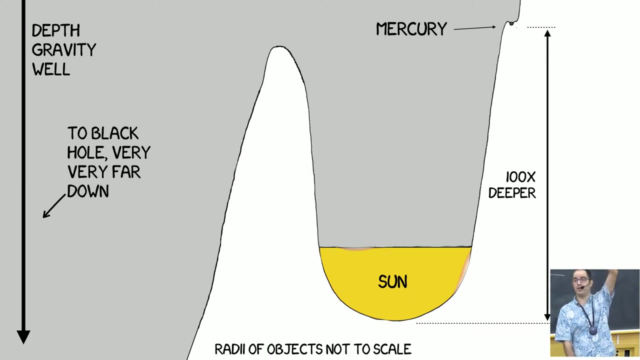 is one meter deep, okay. And this metaphor for gravitational potential: wells, if the potential well for Earth was one meter, for Jupiter it would be 15 meters, okay. For the Sun, the potential well would be three kilometers, okay, Three kilometers. 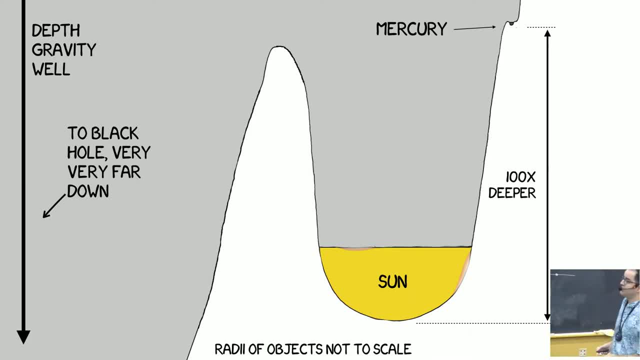 One meter Earth Sun, three kilometers, It turns out. if you want to draw in the same scale, the height of the potential, well, for a black hole, you cannot do this, okay, Because it just doesn't fit. You have to use large scale, okay. 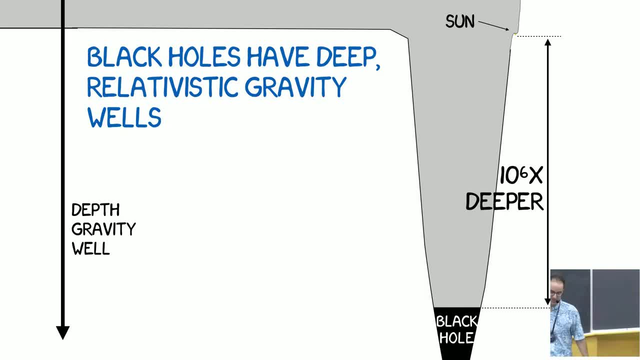 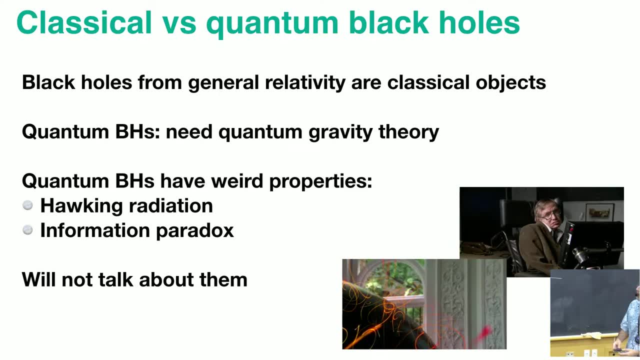 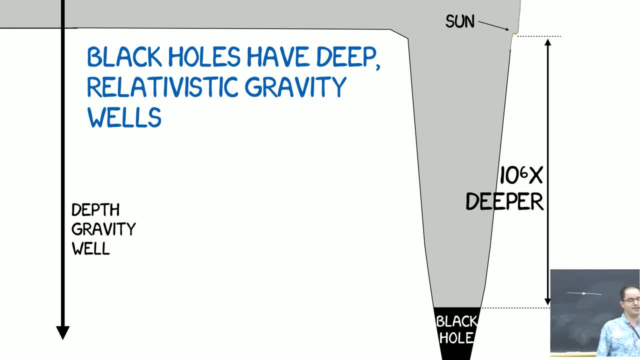 This is, if you try to put in the same scale, you have to use large scale. okay, A black hole. the height of the potential well would be 700,. oh sorry, The height of the potential well for a black hole will be 700,000 kilometers. 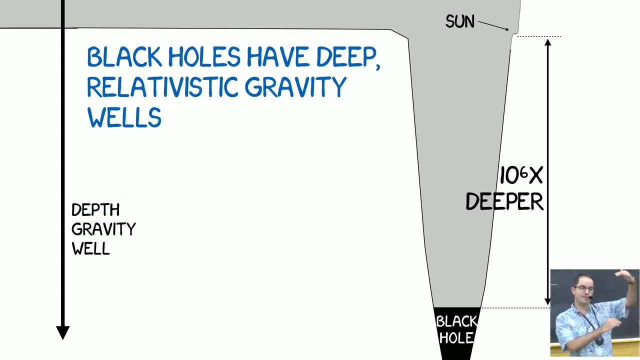 which is two times the distance between the Earth and the Moon. if the potential well for the Earth was one meter, okay, So this gives you an appreciation of how extremely relativistic is the gravity of black holes. If you fall, if you are in the horizon of a black hole, 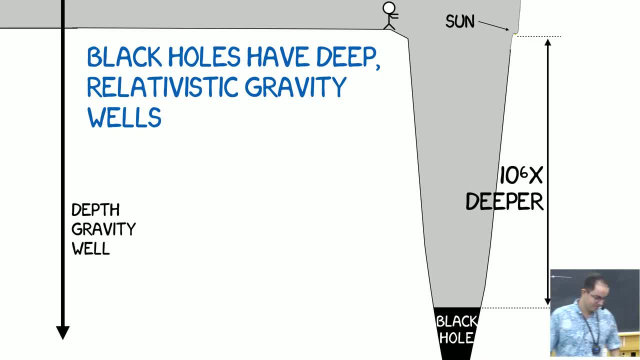 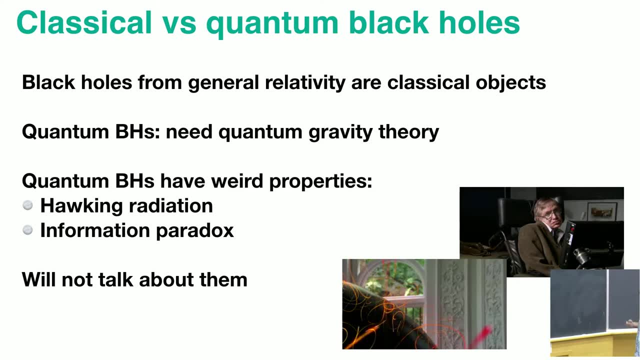 you will be forced to be relativistic. okay, You cannot really fight this. So from now on, of course, all of you know about the Hawking radiation that you can if you have virtual pairs of particles being everywhere in the universe. 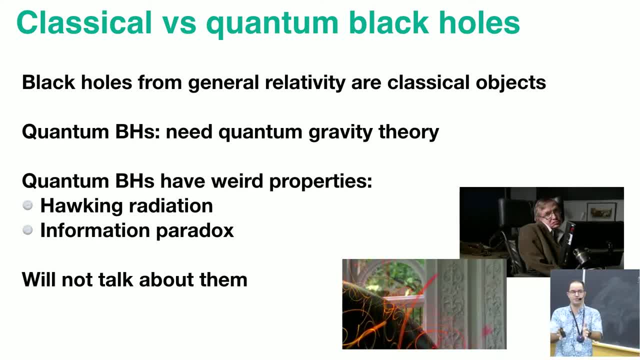 if you put two plates, metal plates, you can turn these virtual pairs in real physical pairs, the Casimir effect. It turns out that this is happening near the event horizon- There is no vacuum in quantum mechanics- So near the event horizon of a black hole. 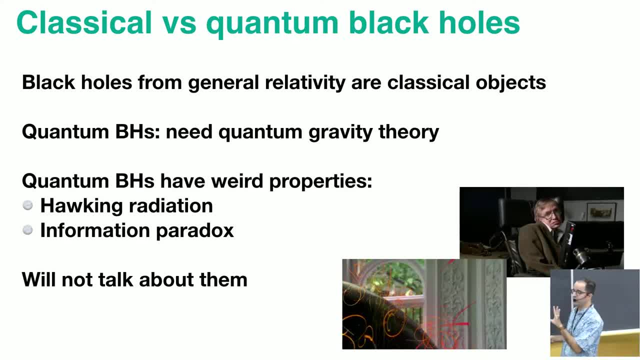 you have these virtual pairs. One of the particles can go to the horizon with negative energy, The other one escapes. okay, The one that escapes is the Hawking radiation. The one that falls decreases the area and the mass with a quantum process. 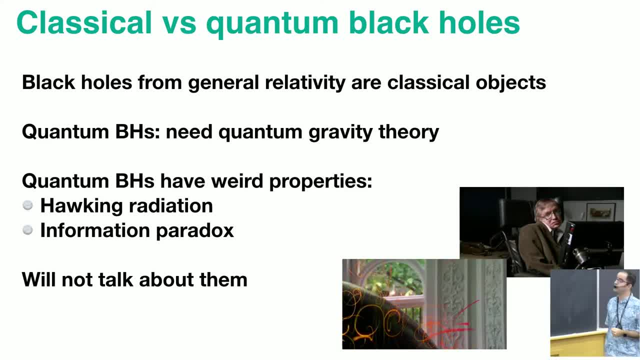 This was a semi-classical calculation by Stephen Hawking in a classical nature paper- 1973, with a very catchy title about black hole explosions in the title of the nature paper. But the thing is, if you work out the Hawking radiation, 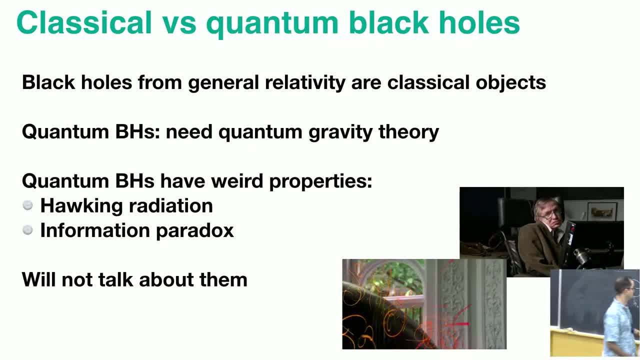 the Hawking luminosity that we get out of astrophysical black holes with masses and about two solar masses. you will find out that this is- I don't remember the numbers off the top of my head, but the Hawking radiation for such a black hole. 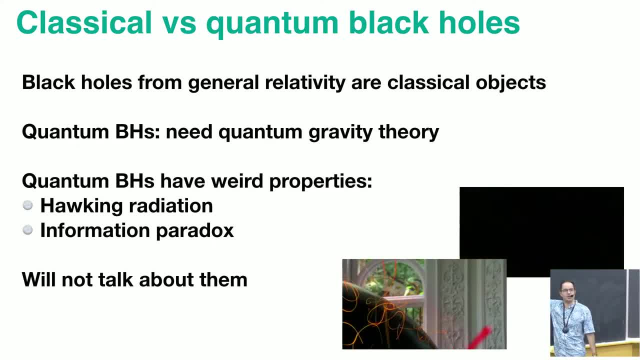 is like more than one billion times less than a solar luminosity or even less luminosity. I don't have the number off the top of my head And if you compare this with the shining glow of the accretion disk around such a black hole, 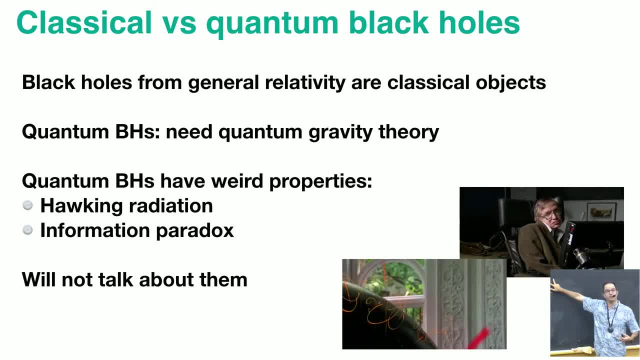 the Hawking radiation is completely meaningless. So for me and astrophysicists, I don't pay attention to the Hawking radiation right now, But when we leave quadrillions of years in the future, our robot overlords the heat pad of the universe. 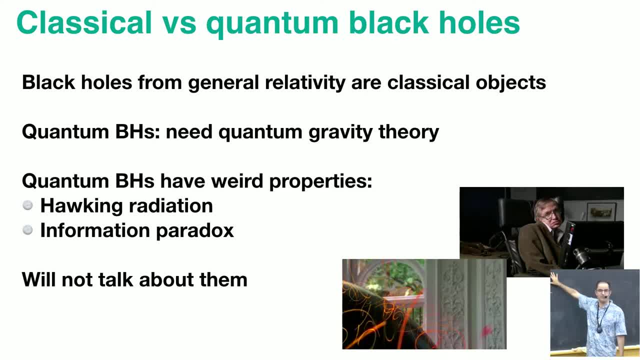 Hawking radiation will be interesting. It will dictate the cosmological evolution of the universe many quadrillions of years in the future. But right now there is no reason to really bother Hawking radiation for astrophysical black holes, So I will not mention Hawking radiation. 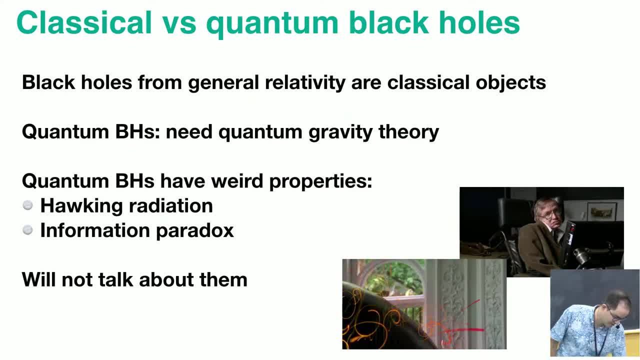 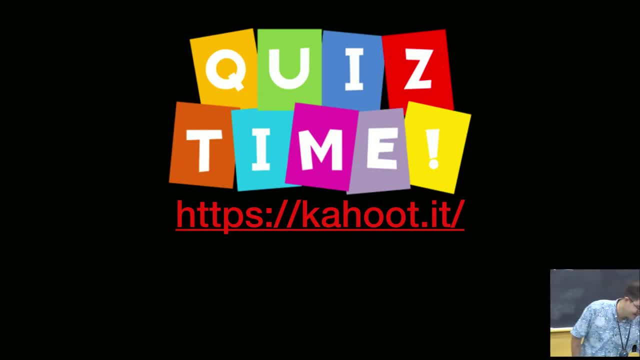 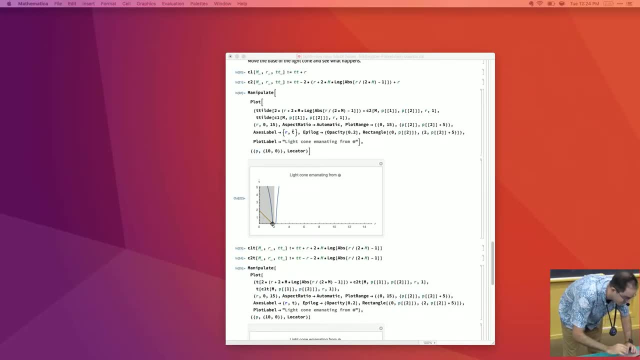 from now on in my lectures. okay, All right, Quiz time. Get your cell phones, get your tablets, get your laptop, plug your AI of your minds in the Wi-Fi, if you have one, if you are coming from the future. 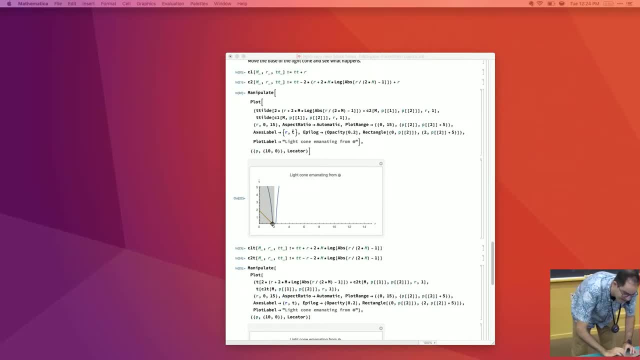 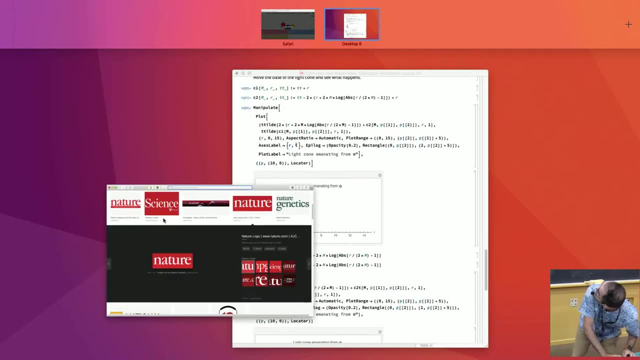 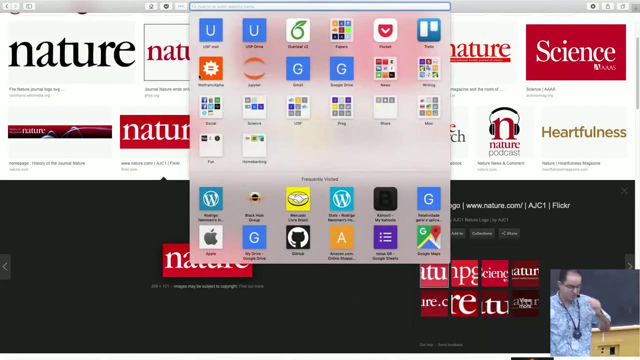 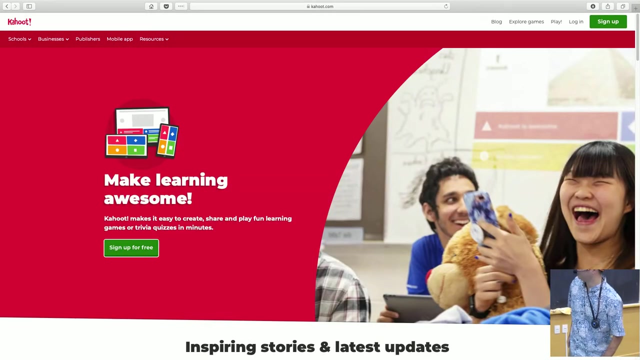 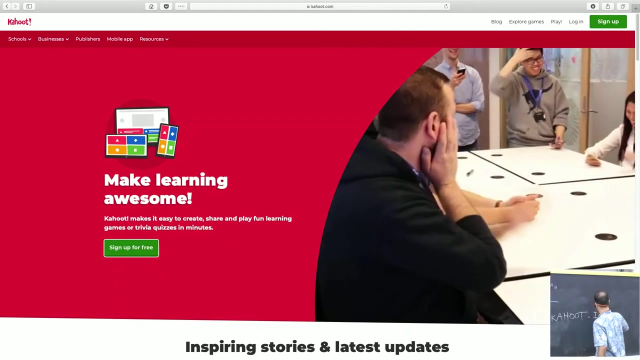 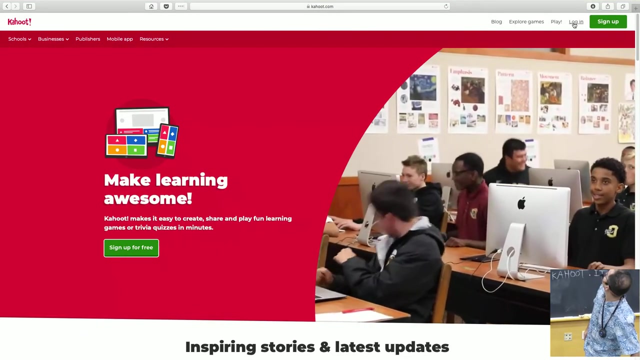 And let's do this. Very simple quiz, Nothing fancy, Just to have fun and see how much you know. Very simple, conceptual questions. So go In the meantime, go to this address. Okay, Let's do this, We are having fun. 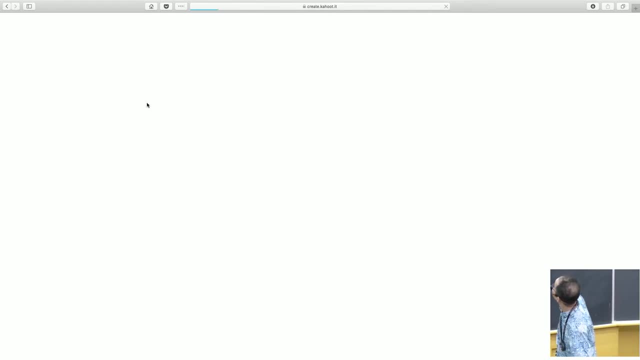 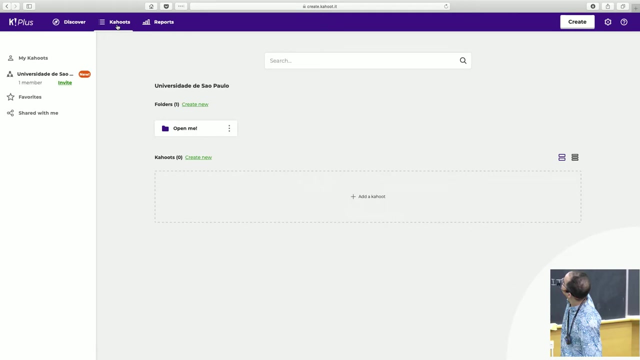 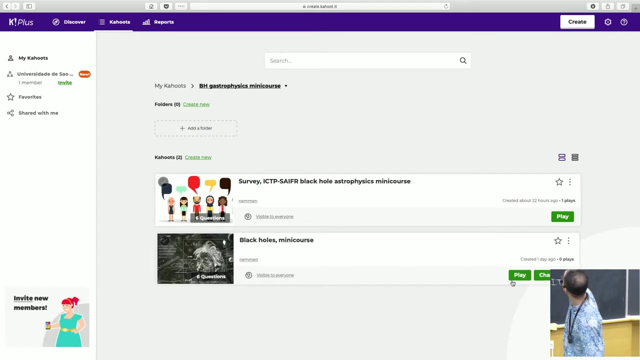 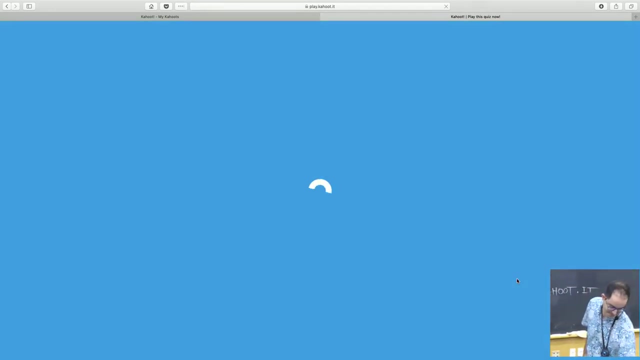 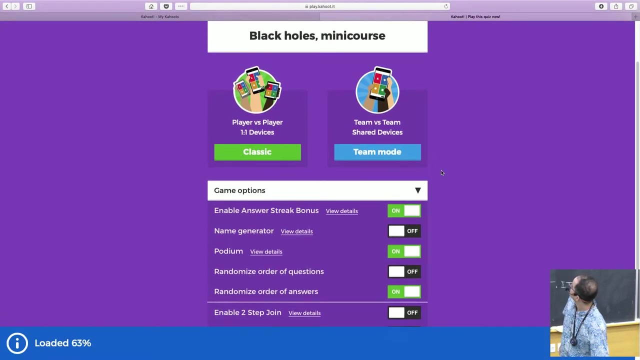 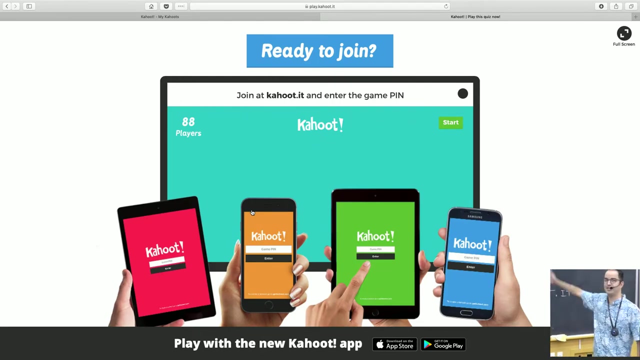 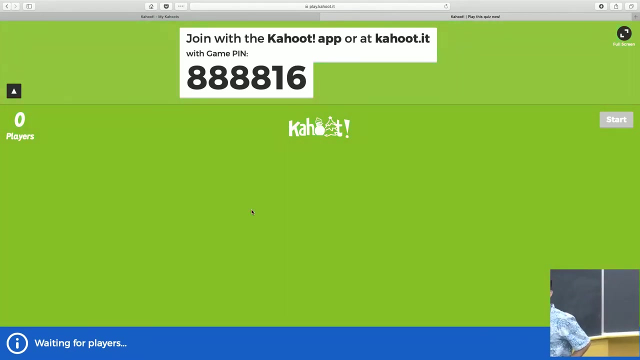 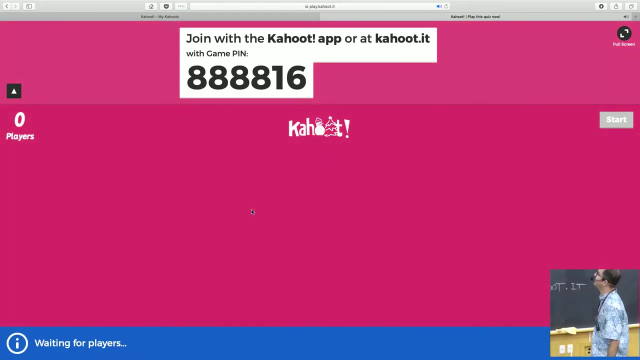 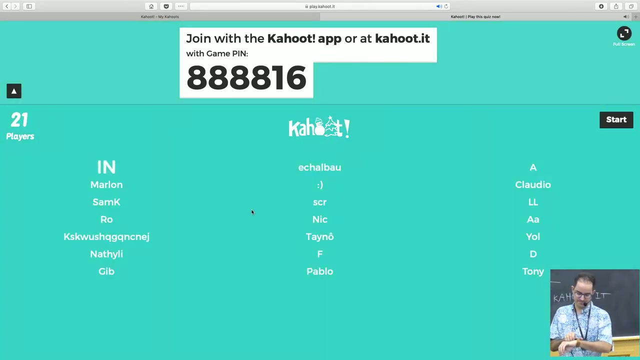 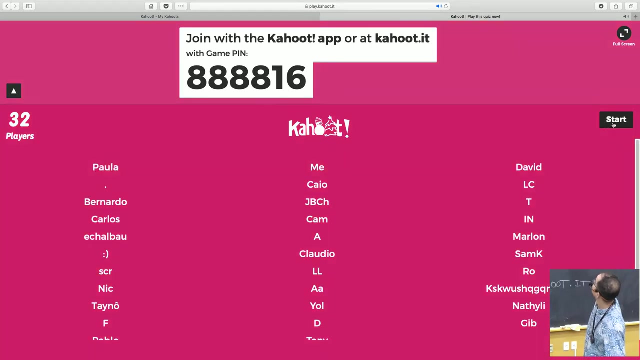 Look. Okay, Are you connected to Kahootit? Let's do this. Please enter this code. Professors are also welcome to join this. 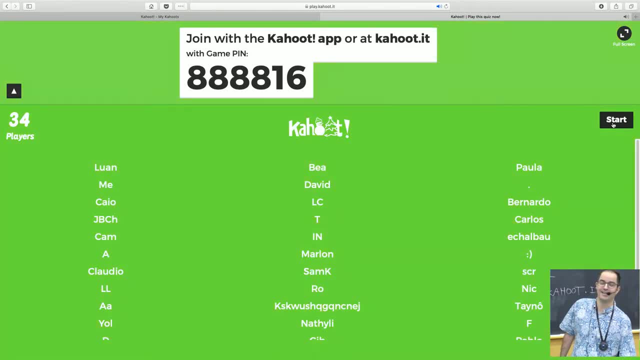 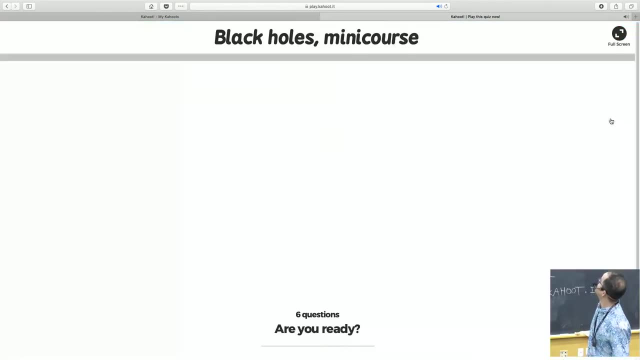 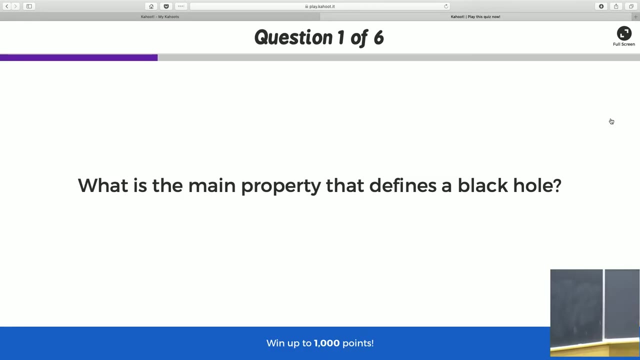 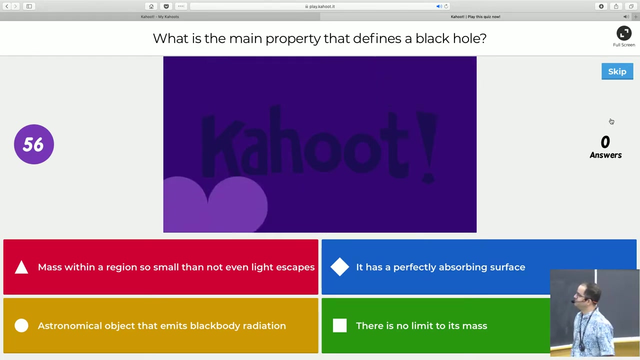 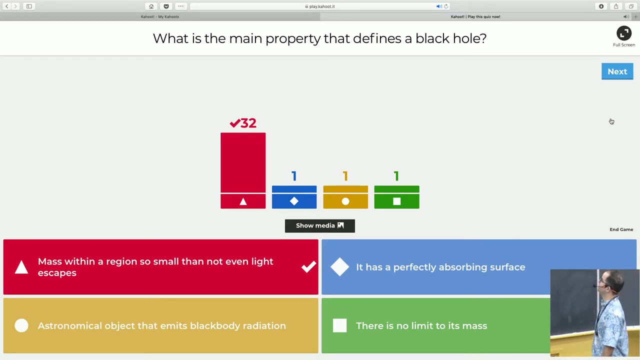 Okay, Most of you got the answer correctly. Okay, What I'm referring to is the main defining property of a black hole. Okay, Very good, Screwer is in the top podium. 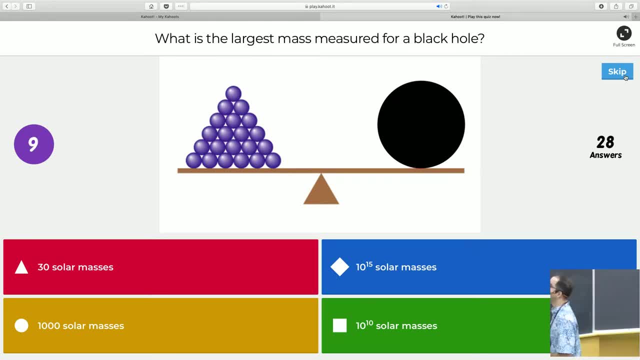 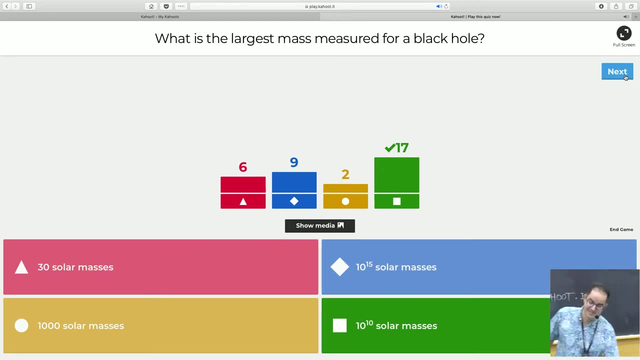 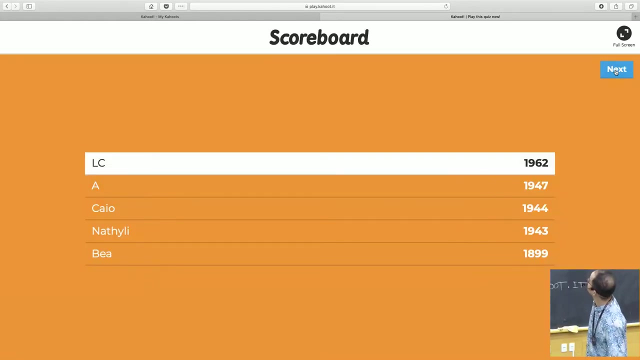 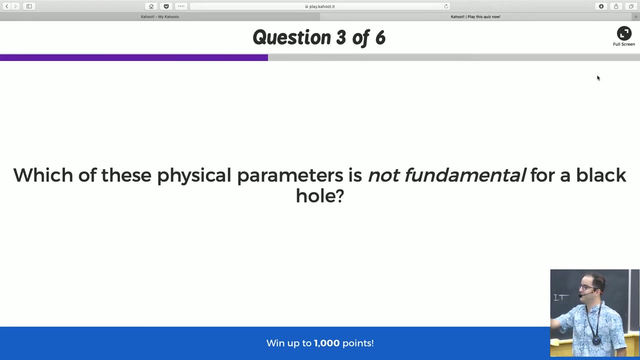 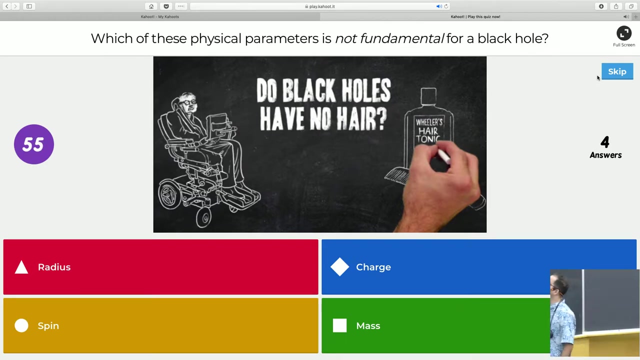 Okay, The largest mass was 10 billion solar masses. as I just mentioned in the lecture, the maximum mass measured for a black hole Curve is in first, now Later. Ah, thank you, I should have put last question. We don't need 60 seconds to reply. Okay, It's. 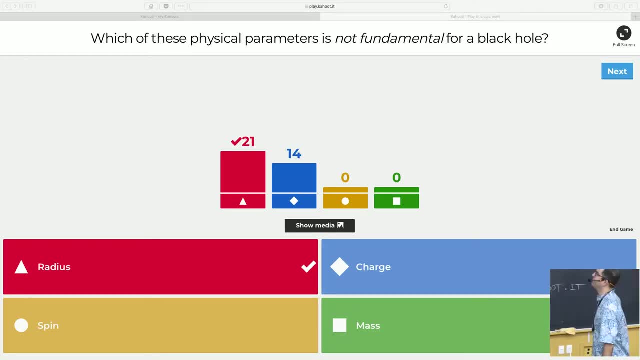 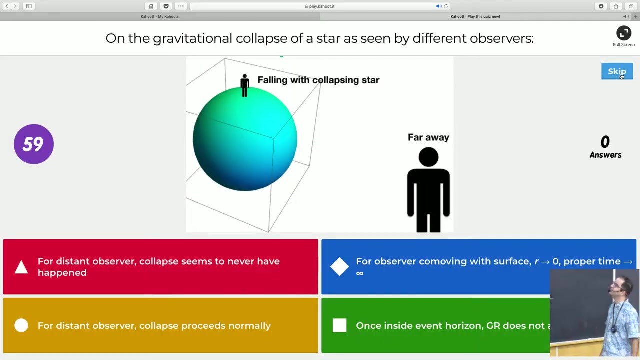 not fundamental. Okay, So radius is really from a theoretical point of view. the radius is derived from the other parameters, Okay, Okay. Okay, So mass of diseasedacaks charge is not really important, but in general This one is tricky. 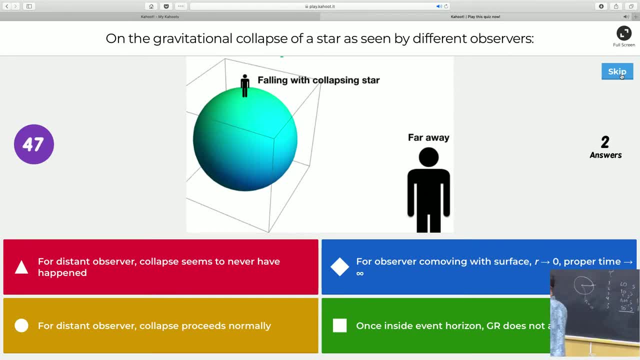 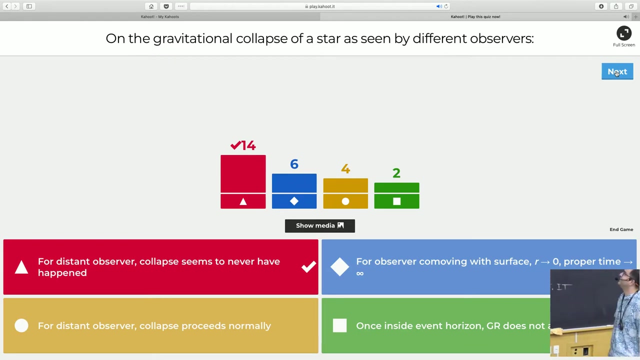 This one is tricky. Aha, we have an almost flat distribution. okay For a distant observer: he or she never really sees the black, the star collapsing. okay For the moving observer: he will go fall in the physical singularity and die there. 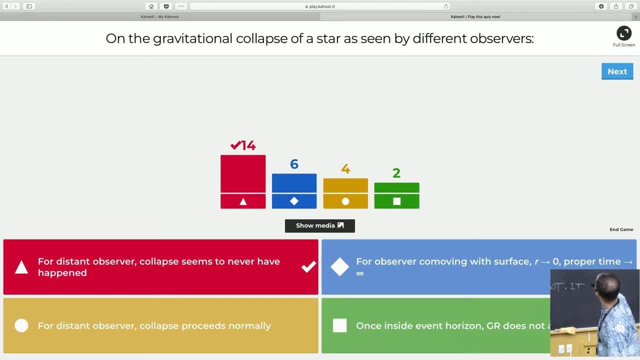 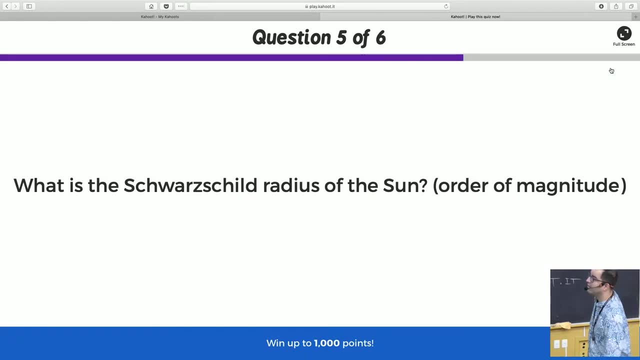 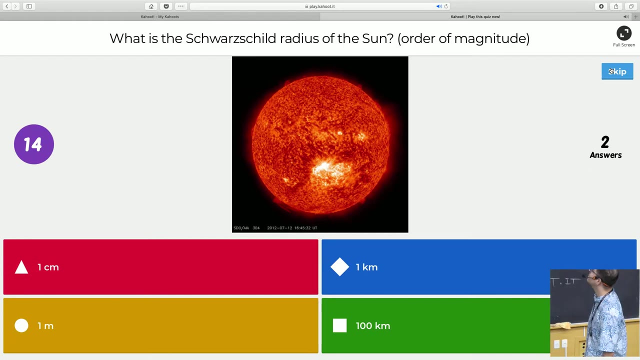 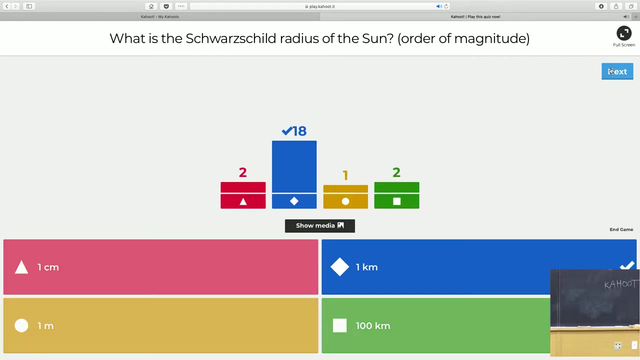 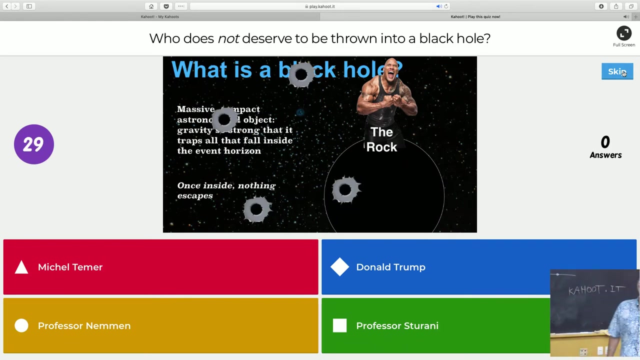 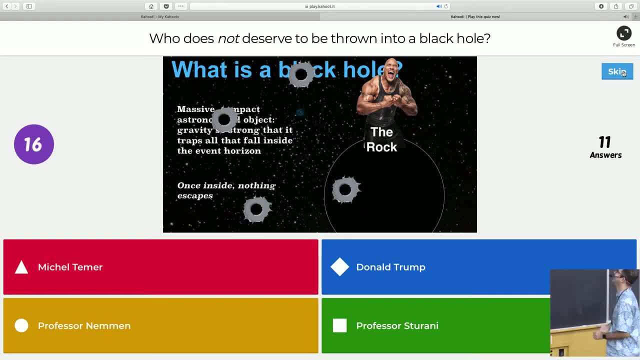 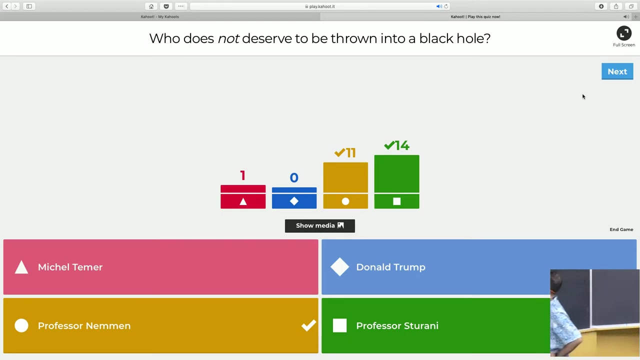 This is a tricky one, Who does not deserve. okay, let's be clear. Let's see. Okay, OK, Very good, Somebody really likes Michel Temer here. OK, Good to know. Yeah, OK, We are done. 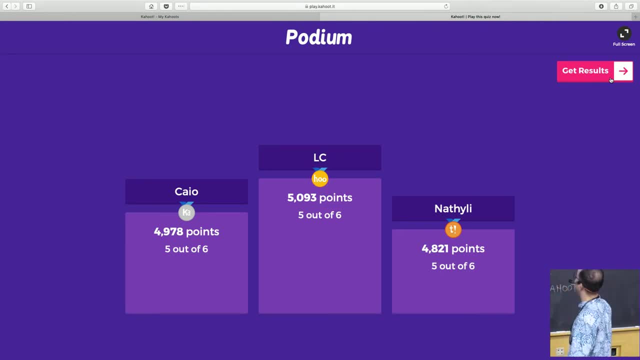 Congratulations, LightCurve. You got the first place. Caio, congratulations. Nachili- congratulations. I will start his results with the quiz and give a surprise prize at the end of the lectures for the top person. So please use a consistent username. 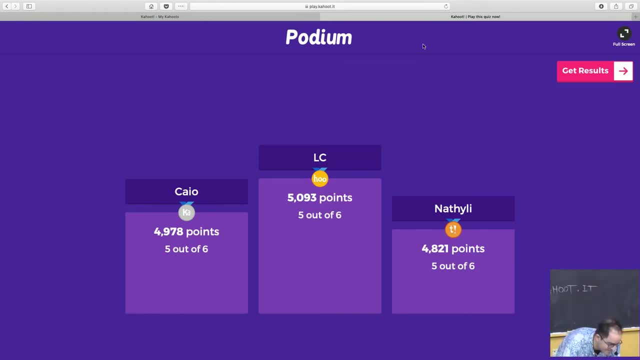 throughout the quizzes. OK, Because I really use this to give a prize at the end of the lectures. OK, We can discuss the appearance of a collapsing star at the end of the lecture or in the discussion section. Let's move on now. 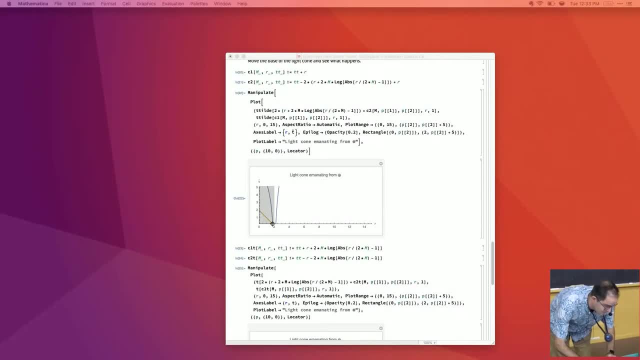 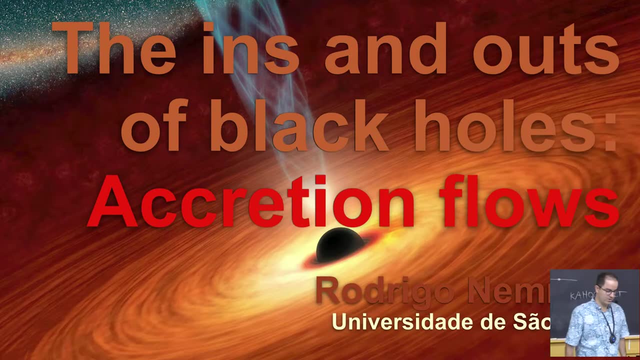 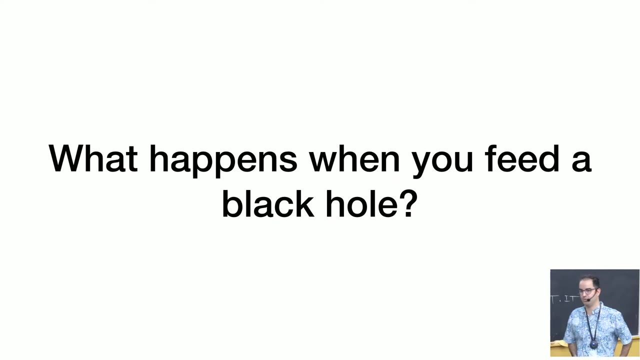 Let's move on now and talk about the ins and outs of black holes flows, And starting with the first question, what happens when you feed the black hole? What happens when you throw test particles in a black hole? We already know the answer. 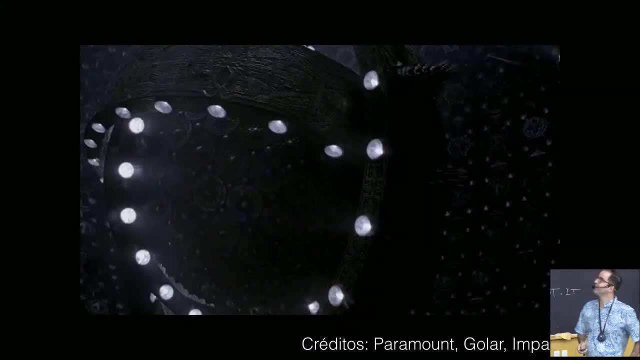 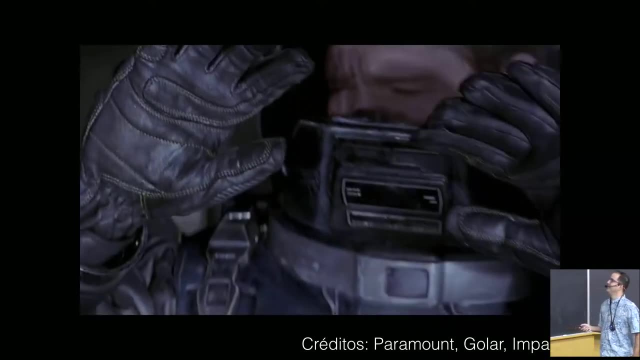 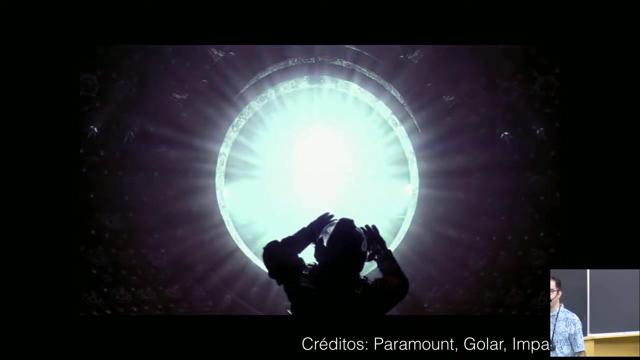 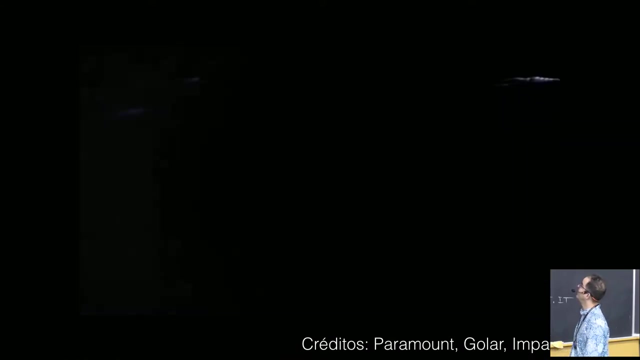 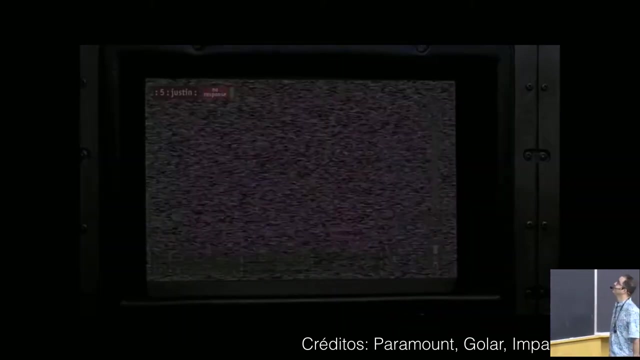 And Hollywood answered us. So here, Here We have a fictitious black hole in some movie. OK, It was found in an abandoned spaceship. Somehow these guys are using black hole to power the energy of the spaceship, Feeding with his hand the black hole. 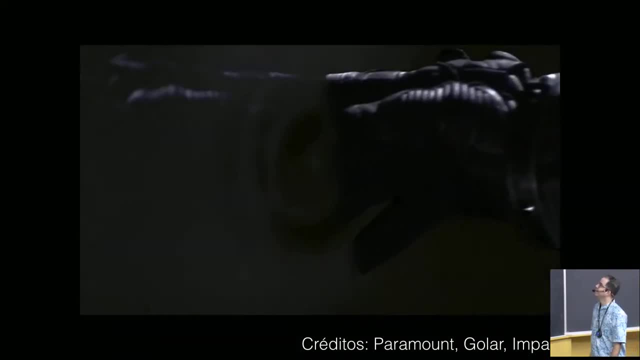 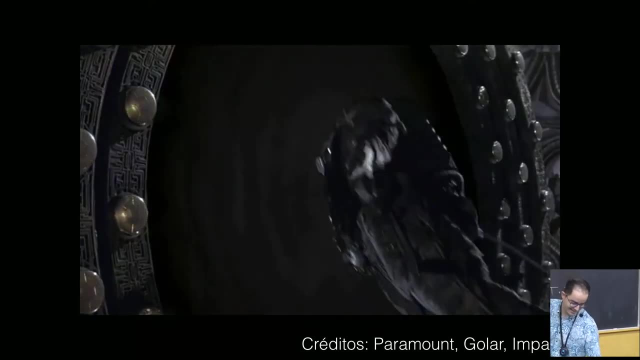 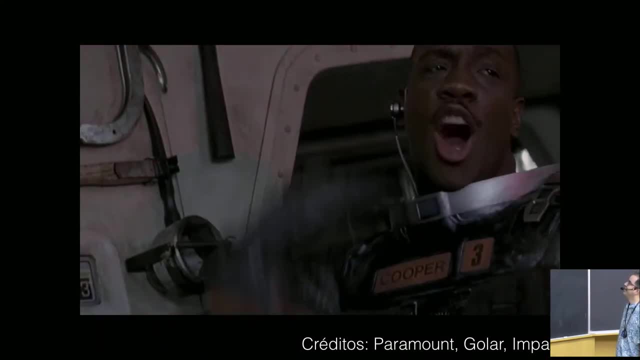 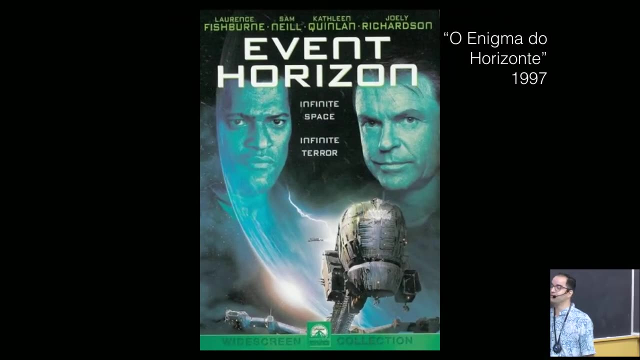 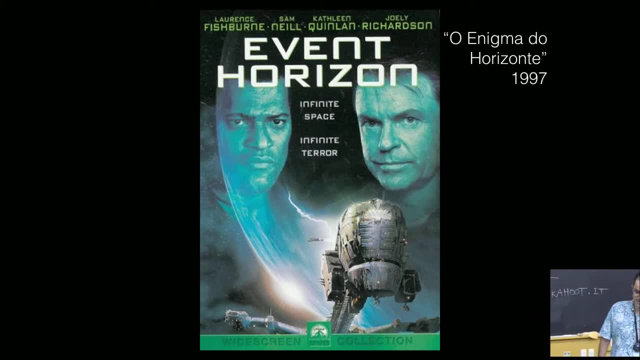 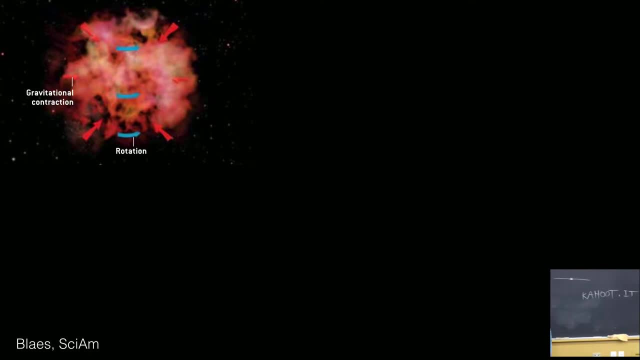 has terrible science, But it's a fun movie to watch. I really recommend it. So this is what happens when you feed a black hole. You feed a black hole with a cloud of gas. They usually have angular momentum As the cloud dissipates energy due to the angular momentum. 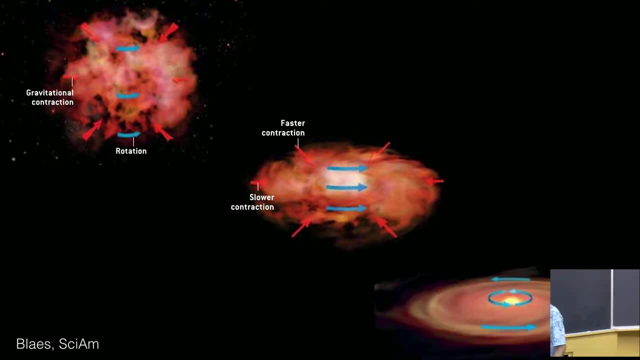 you expect to have the general formation of disks when you have material with angular momentum towards the central object. due to the conservation of angular momentum, This is the lowest energy state of this cloud of gas as it evolves and dissipates energy, And this is why you have disks in galaxies. 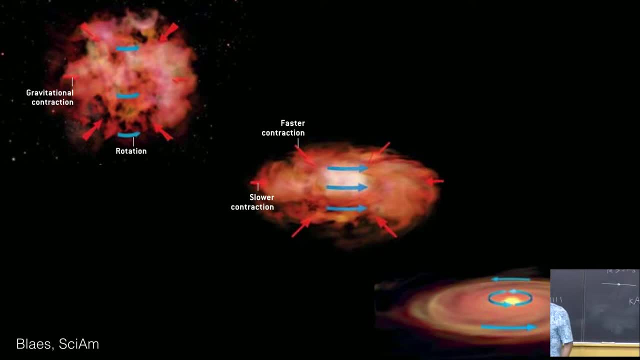 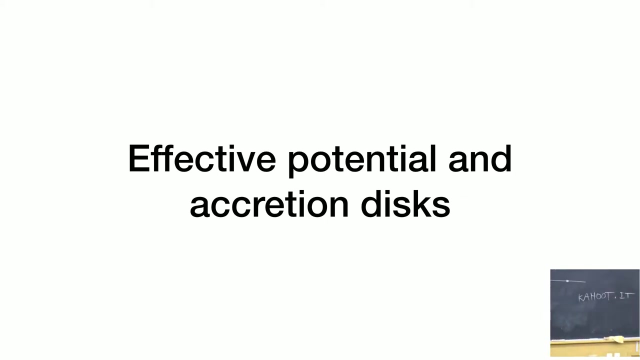 You have disks around black holes. You have disks around young stars forming planets, So disks are ubiquitous in the universe And this is not different for feeding particles onto a black hole, And we can use the theory of the problem in general relativity to understand. 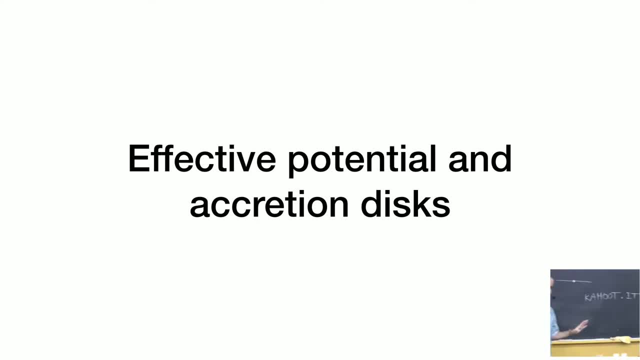 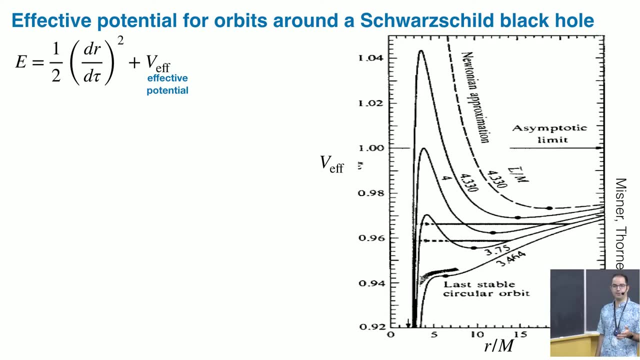 some of the main features of a so-called disk around a black hole. So thank you, Ian, for deriving this lecture So you can write the effective potential for a Schwarzschild black hole, also for a Kerr black hole, if you want to do that. 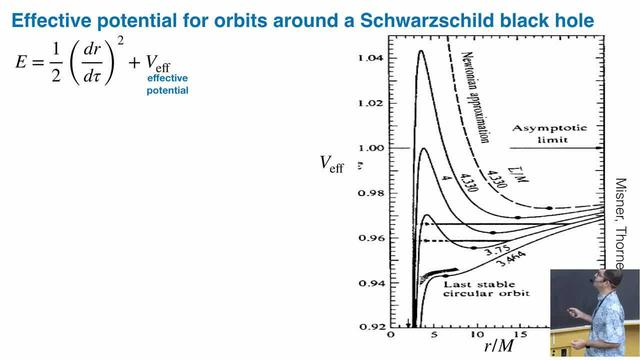 This is how you put the problem in the framework of the effective potential, And then you plot the effective potential and you can use celestial mechanics methods to analyze what happens. So imagine you have a disk. You have a disk of particles circling around the black hole. 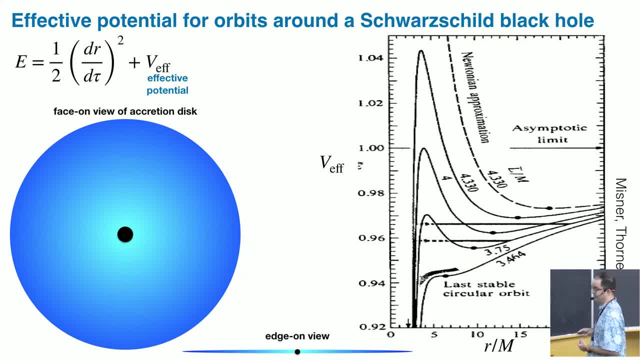 So different particles, different orbits. they have different angular momentum here. So we start putting a circular orbit in the minimum of the potential, a stable circular orbit. at that point It corresponds to this in the accretion disk. You go closer. 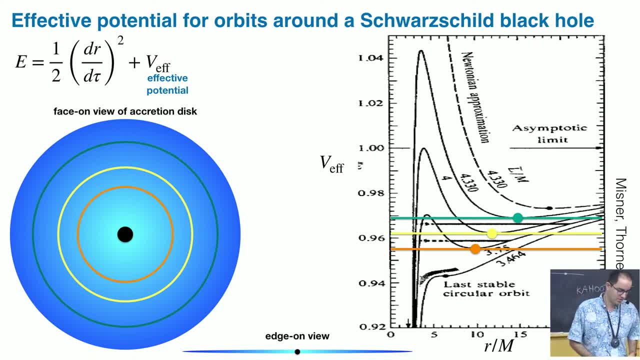 You put another, the yellow orbit. You get closer to the black hole. You put another orbit, You get closer to the black hole, Until the point where the angular momentum is so low that you don't have anymore the feature of the maximum in the potential. 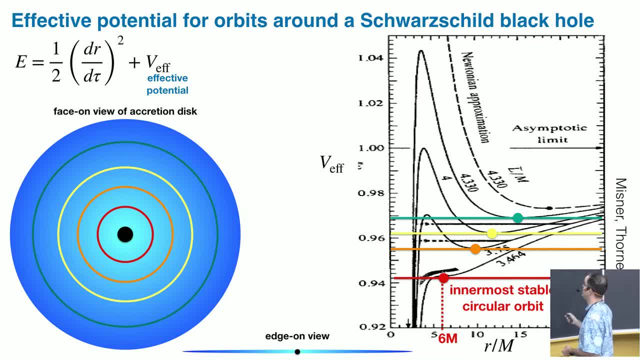 You don't have anymore the pit in the potential feature discussed by Ian yesterday. You have the radius of the stable circular orbit which for a Schwarzschild black hole is located at 6m, So you cannot sustain any more circular particles inside this innermost stable circular orbit. 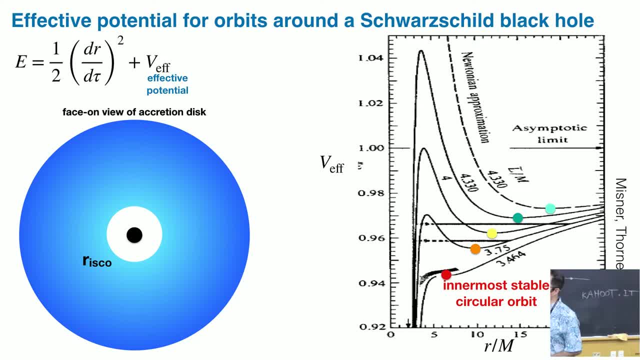 around the black hole. So what happens is you expect in accretion disks around black holes that inside the innermost stable circular orbit you will have literally a hole in the accretion disk. Part of the black hole inside the ISCO will ballistically fall onto the event horizon. 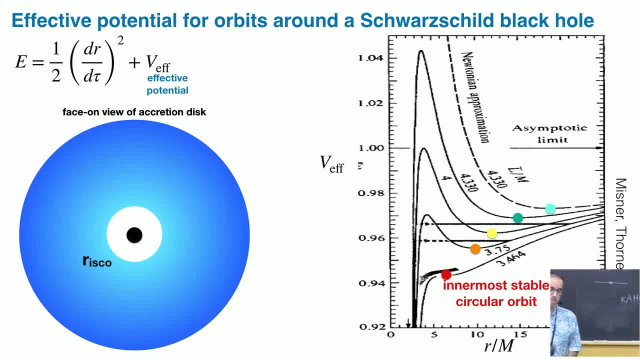 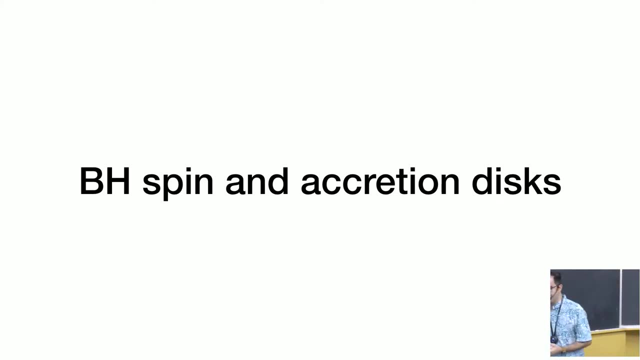 So in the accretion disk. OK, You can understand all of this with this effective potential. This is similar. It is. It's a simple concept, but it has profound implications for black hole astrophysics. Talk a little bit about black hole spin. 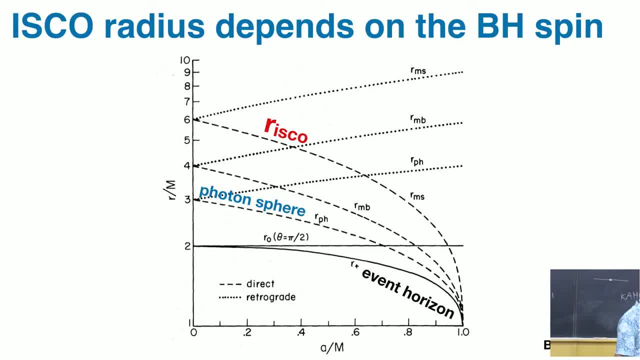 and the effect of black hole spin on accretion disks. It turns out that if you do the calculations of the event horizon and the effective potential for a curved black hole, the radius of the innermost stable circular orbit decreases considerably as you increase the black hole spin. 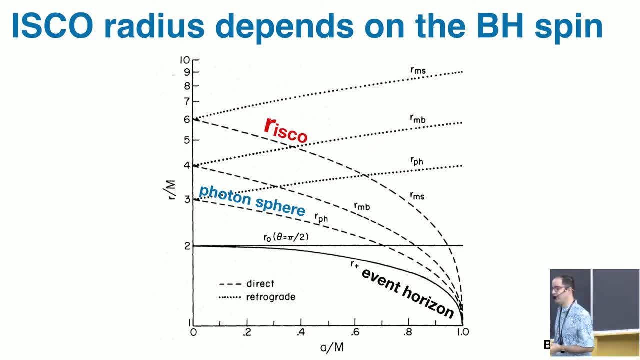 In fact, for a maximally spinning black hole, the ISCO radius touches the event horizon and correlates perfectly with the event horizon. This is the dependence of the radius of the full sphere, where you can have photons in circular orbits around the black hole. 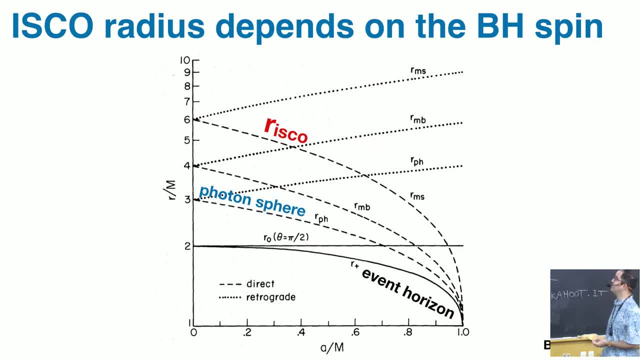 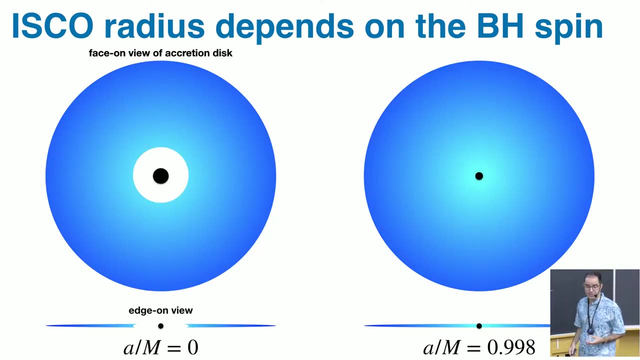 It decreases from 3 to the spin And this is the radius of the event horizon of the black hole, which decreases, as I mentioned, from 2 as you increase the black hole spin. So it's a simple concept. So it turns out that if you have an accretion disk around, 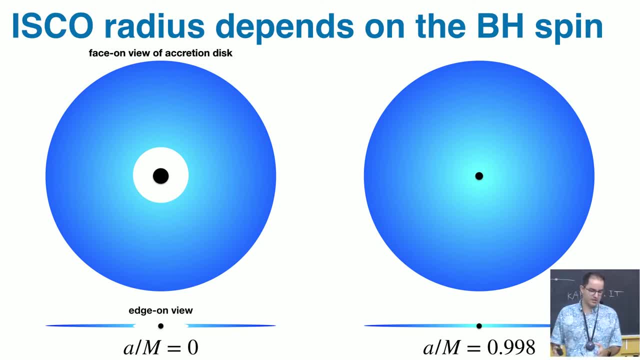 a black hole. on the left side you see the hole in the middle of the disk or a Schwarzschild black hole, And on the right side you see the hole in the middle of the disk when you have a maximally spinning. 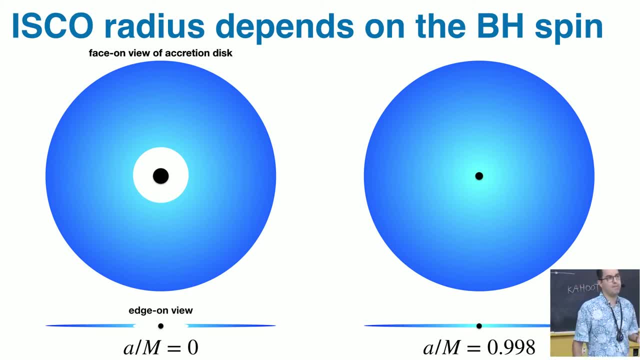 Kerr black hole. So what is the impact when you have particles in an accretion disk orbiting a Kerr, a maximally spinning Kerr black hole? OK, So what is the impact when you have particles in an accretion disk orbiting a Kerr, a maximally spinning Kerr? 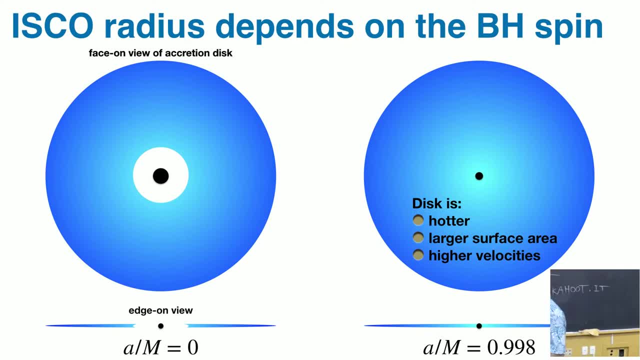 black hole. It turns out that the disk will have access to inner orbits than the disk around a Schwarzschild black hole. So the disk will have larger velocities. It will have a larger surface area because it's going deeper in the potential. 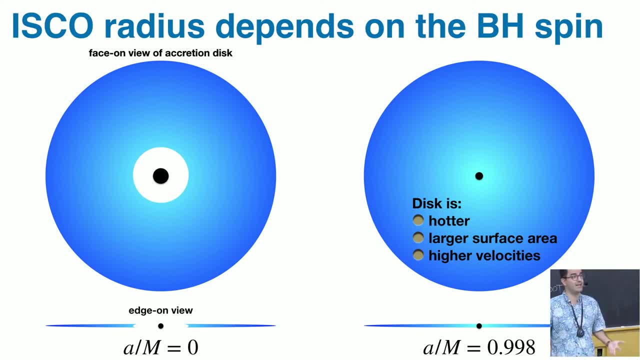 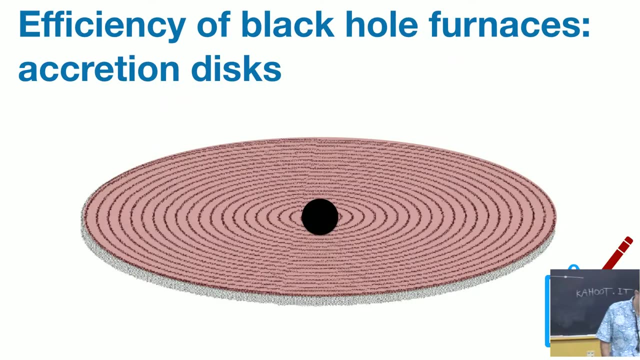 And it will be hotter because it will have higher temperatures of the gas close to the event horizon. So deep implications, as I mentioned, for observational astrophysics, when you're trying to observe and measure the spin parameter of the Kerr metric. 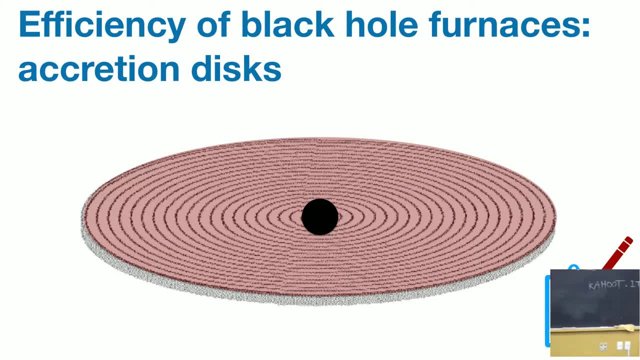 Let's now have a few words about the efficiency of energy extraction from these black hole furnaces in accretion disks. OK, So our agenda now is that we want to derive a simple order of magnitude estimate for the efficiency of energy extraction from these gravitational engines. 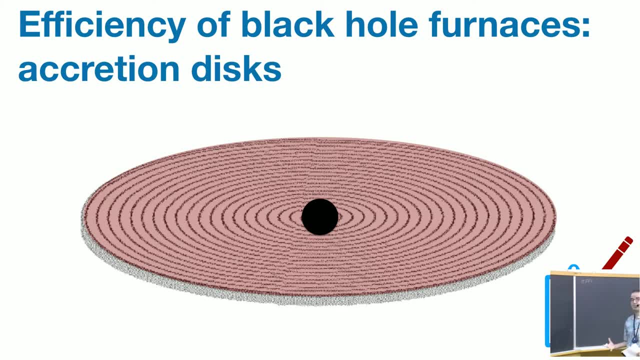 OK. How can you extract blood from a stone? How can you extract energy from a black hole with an accretion disk? OK Ó, Thank you. So it turns out that I imagine you have a nice circular orbit a bit far away. 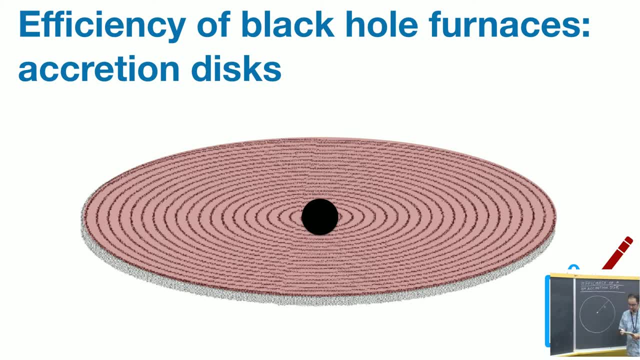 from the central black hole. OK, So we can even say that we can make r, the radius of the orbit, tend to infinity, if we want. OK, So what is happening here? imagine that we have some physical process operating in the orbit of this particle. 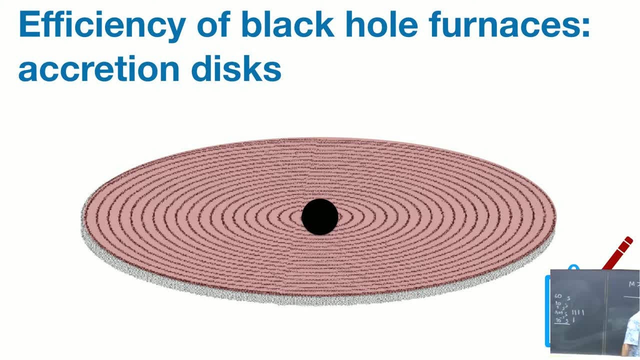 such that it is dissipating the mechanical energy of the particle and it's making loose energy. So what happens when you start dissipating energy for the orbit of this particle around some central generic object? okay, The particle will start depending on how fast this energy interaction is occurring. 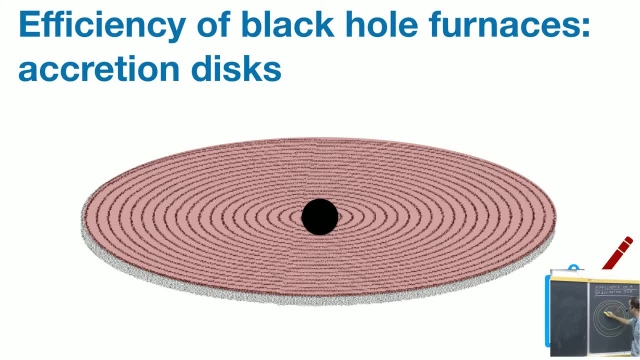 the particle will start losing gradually energy and spiraling towards the central object. okay, If you turn on some mechanism for dissipating the energy. okay, So the particle, of course, is losing orbital energy and the actual process that dissipates this energy. 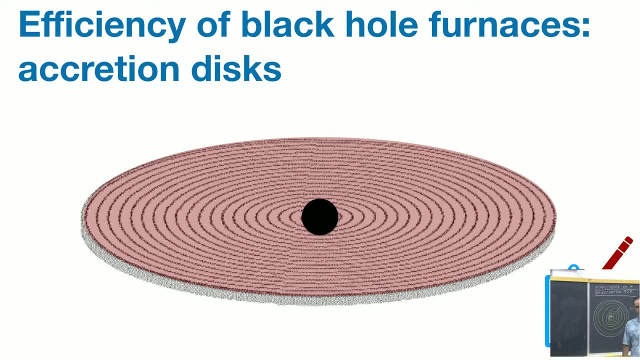 is turbulence. These disks are very turbulent. They are dissipating the energy on larger scales towards smaller scales, towards the Kogorov scale of the problem, where it is dissipated in thermal energy. okay, But I will not really talk much about turbulence. 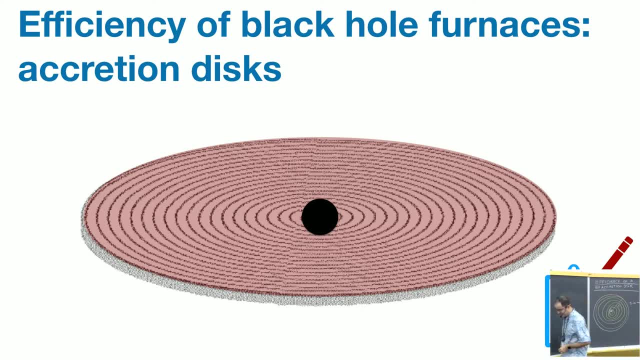 because turbulence. there is a joke- I don't remember if it was Heisenberg or Feynman who said this joke, that somebody I think- I don't remember if it was Feynman or Heisenberg or somebody else. 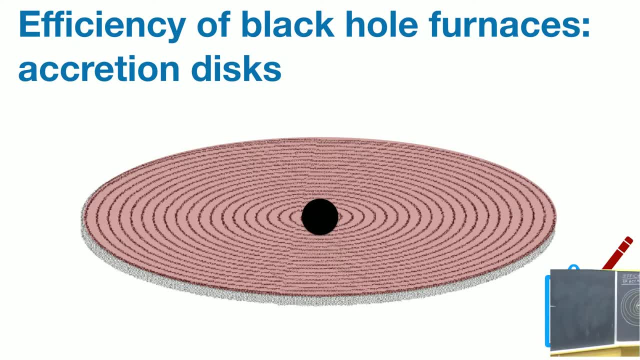 they asked this person: suppose you died and you wanted to ask questions. you wanted to ask. you wanted to ask questions to God. what would you ask God? And then this person said: well, I would like. the first question I would like to answer is: 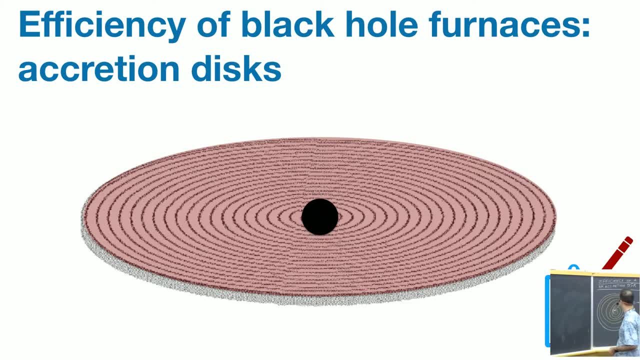 what is turbulence? How to understand turbulence? okay, Turbulence is one of the complicated classical problems that we have. But anyway, so there is. it's losing orbital energy, it's converting this orbital energy into thermal energy and it's radiated away eventually from the disk. okay, 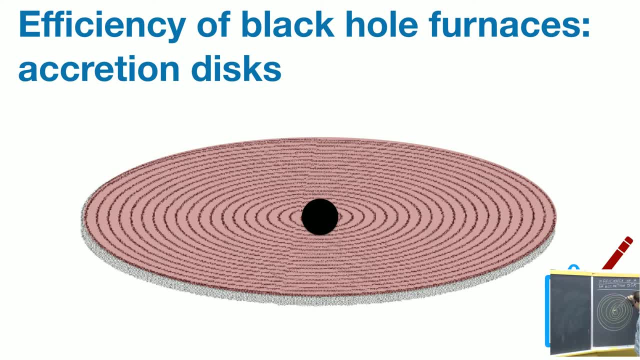 So, by the time the particle fell from this radius towards, potentially, the event horizon, the black hole, how much energy was released by the particle as it spirals inwards? okay. How much energy was lost by the particle and dissipated in the system? okay. 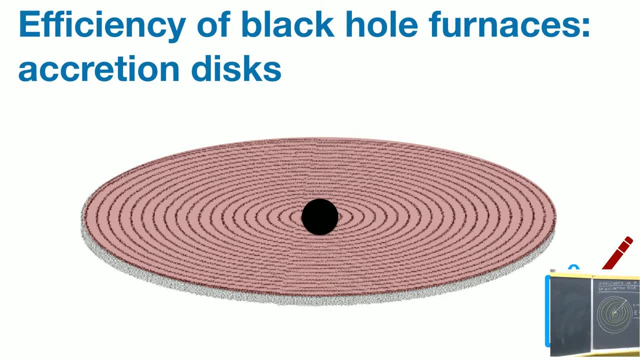 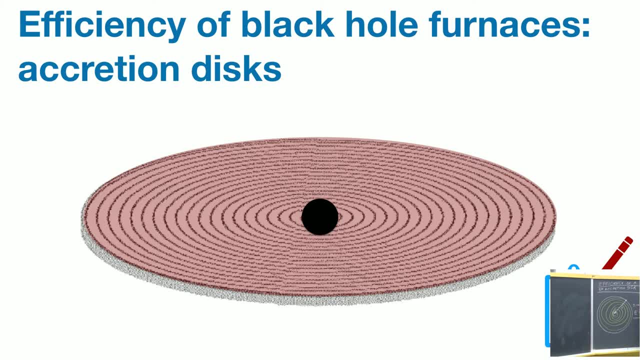 Let's imagine that infinity, the velocity, the distance is very small, velocity is very small. and when it touches the horizon, let's imagine that the particle stops, okay, And then we can compute the accretion, the energy released by accretion, as the difference. 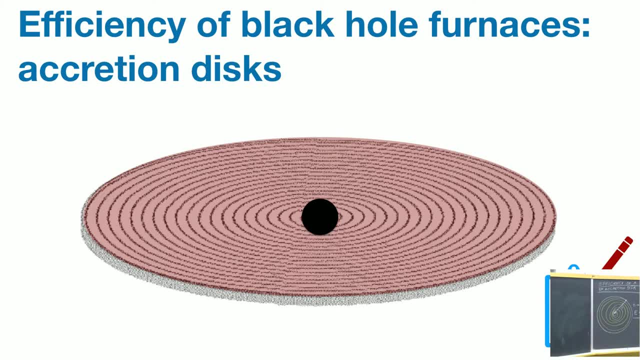 in the potential energy of the particle very far away from the central object, minus the gravitational potential energy of the particle, minus the gravitational potential energy of the particle at the radius where it stops orbiting the black hole and falls into the black hole. okay, 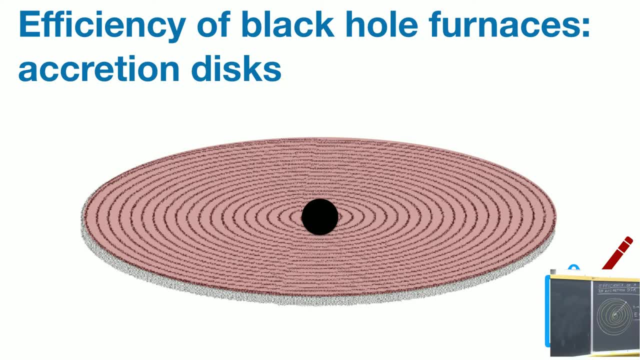 So of course, this is a simple calculation. r tends to infinity. this is not really relevant. it goes to zero. And then let's put the innermost radius where the particle falls. I will call it r dot. So let's put r dot. 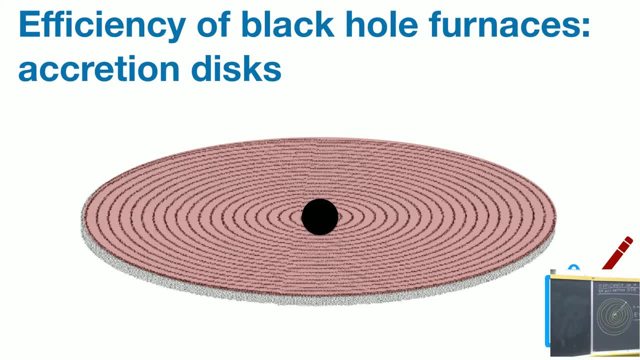 So this gives you an idea of the energy released by the, the total energy released by the particle as something dissipated its energy. okay, It's simple by this formula: g, m, the mass of the central object, the mass of the test particle and the final radius. okay, 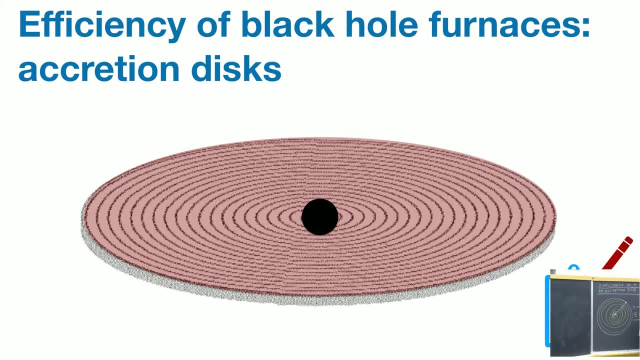 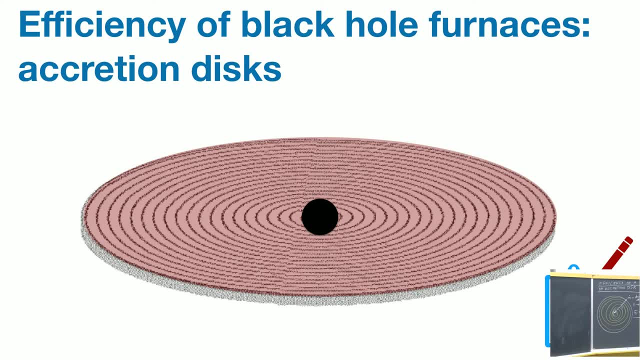 What if you have a continuous flow of particles towards the center object? okay, so far, so good. right, very simple, very easy, only newtonian mechanics, nothing fancy, okay. so if you remember the last lecture, okay, the lecture we use to try to characterize the angle of strength in the sense that 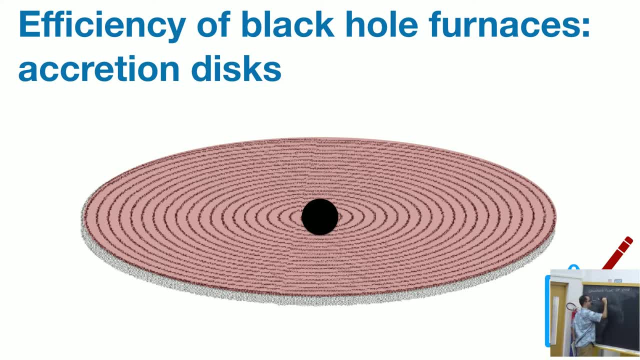 wrote the luminosity of the system as some inflow of rest mass energy factor which controls what fraction of this infalling rest mass energy is converted into luminosity. so you can write the efficiency as the luminosity over m dot c square. we can write the efficiency, but we just derived from new mechanics an actual 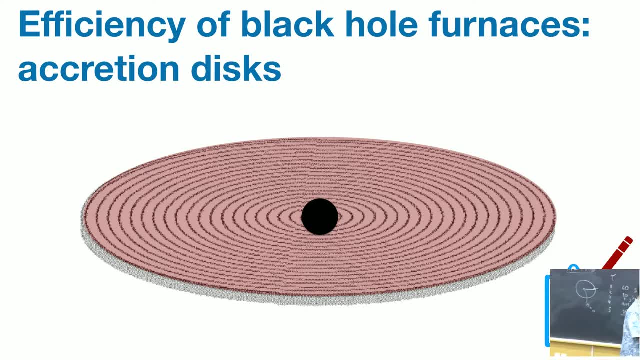 expression for an order of magnitude estimate of the luminosity released by a creation of matter, which we can just put here, and i will draw and see this geometrized unit. so we have here- sorry, oh no, yeah, it's correct, yeah, and we get in the end that the efficiency of energy release is simply the ratio of the mass. 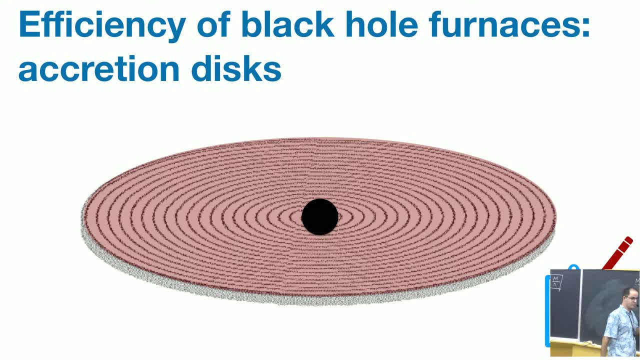 of the central object divided by the radius, where the particle stops orbiting, the black hole just falls in ballistically onto the black hole. okay, so this is, let's call this, the efficiency of release of energy by accretion. okay, and it is really. the efficiency of accretion is depends on how compact your center is. 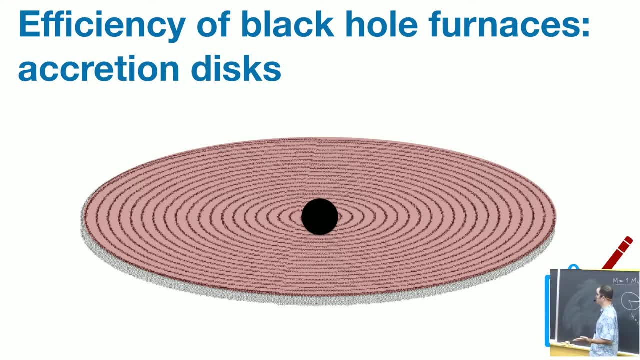 the more compact. in other words, the larger the ratio of mass over radius here, the higher the the efficiency that you will have releasing by accretion. okay, so now, if we consider a schwarzschild black hole solution as the object, okay, let's for fun, let's just let's not think about. 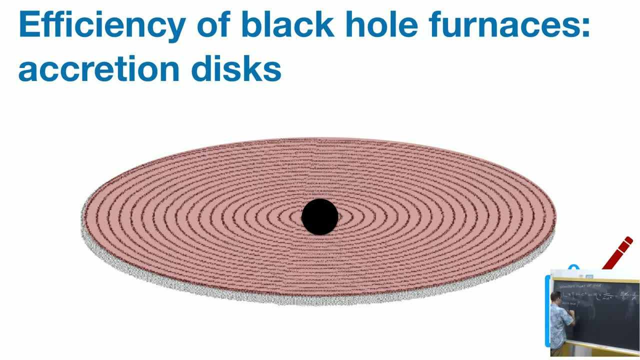 consider that the final radius of the is the schwarzschild radius. okay, in that case the efficiency is of a christian will be m over, sorry, 2 m. so we will have here m over 2 m, so we will have over two, which is 50 freaking percent of efficiency of energy release. 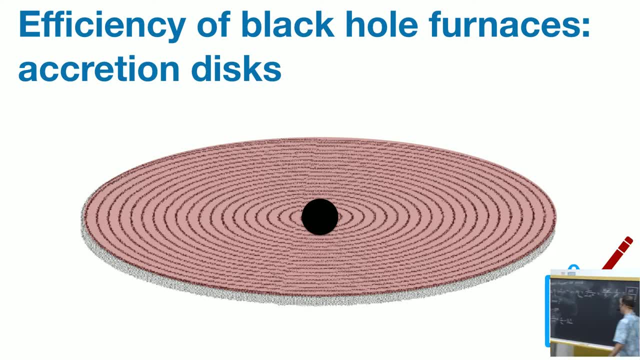 if you have a schwarzschild black hole, okay, it's an magnitude population. okay, this is huge. okay, if it's a black hole, okay, that's a huge ratio and you can produce a black hole. okay, it's a product of mass by power: okay, so you use the dot equation. okay, this is huge. okay, you can produce a lot of energy with this. 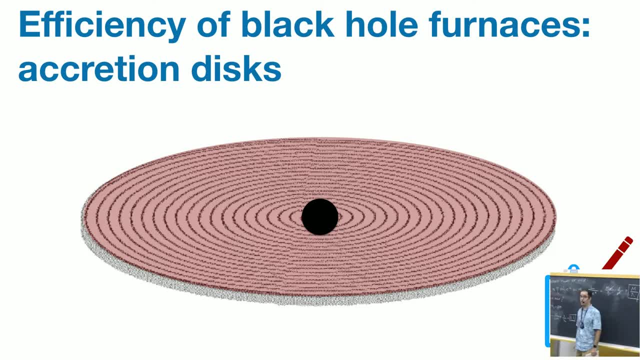 calculation. okay, this is huge. okay, you can produce a lot of energy with this. This is huge. If you are an engineer, in the efficiency of this engine you will lose your sleep getting excited with things that we will never be able to achieve with machines here on Earth. 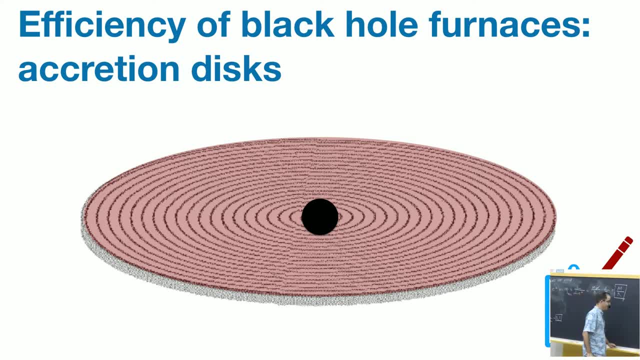 The thing is that, in practice, the last orbit, as we just learned, we learned yesterday and we revised today, the last orbit is dictated not by the Schwarzschild radius. the last orbit is dictated by the innermost state of the nuclear orbit. 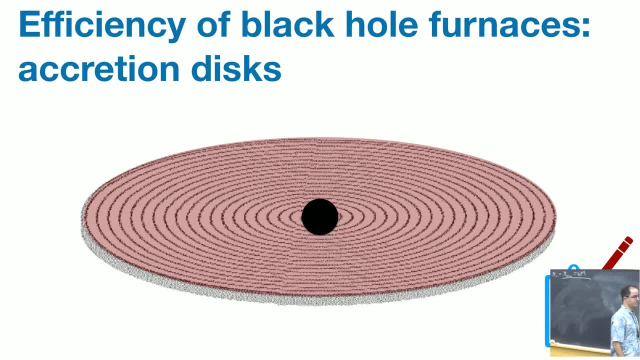 That's the R dots that we should use in the formula to estimate the efficiency of energy release. So the Newtonian equation is a bit more sorry. the GR calculation, The equation of this efficiency And the calculation you have to do then is simply: 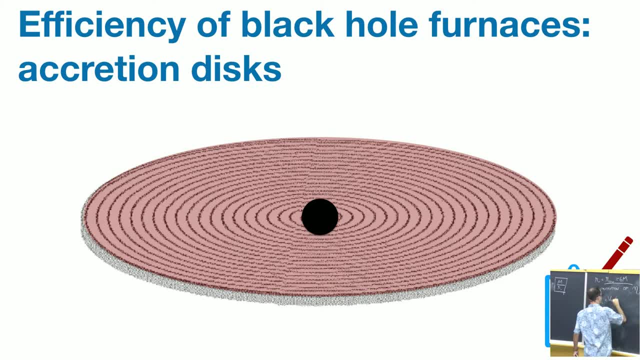 the difference between the potential here at infinity minus the effective potential of the Schwarzschild radius At the isco, which is 6m, and do this calculation And here for the angular momentum of the orbit, you can derive that for the innermost stable circular orbit. 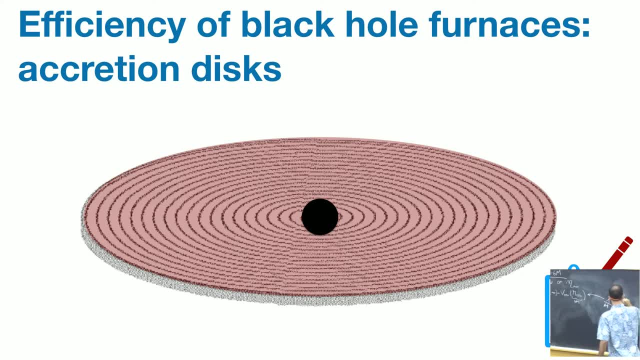 the angular momentum. this is homework if you haven't done this calculation. It's a homework to derive that for the isco, The angular momentum, The angular momentum of the orbit, is square root of 12, okay, So when you put this here, you'll derive that this efficiency will actually be 1 over 18,. 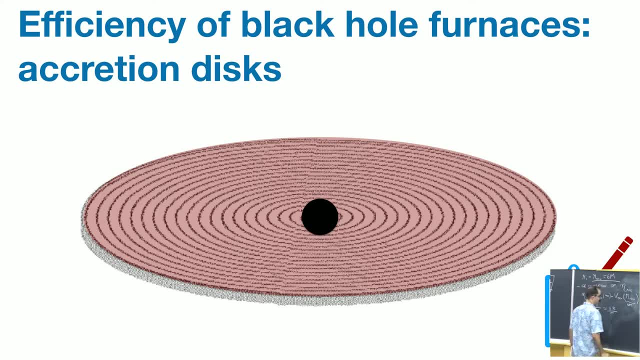 which gives you around a 6% of efficiency. You can round that up to 10%. okay, So this is the efficiency of energy extraction around a Schwarzschild black hole. So it's the efficiency of energy extraction around a Schwarzschild black hole. 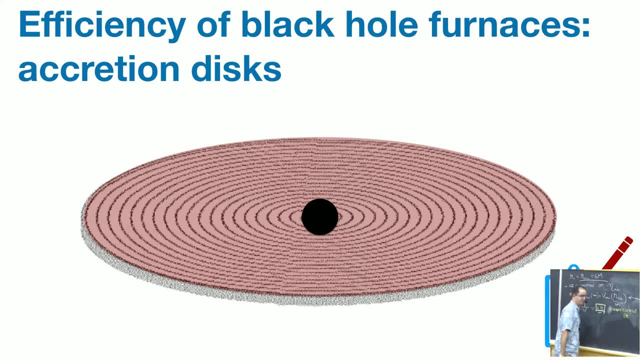 Okay, 6% is the efficiency of blood that you can get out of the stone, The energy that you can get by dumping garbage, slowly dumping garbage into circular orbits around a Schwarzschild black hole. Okay, Now, if you do this calculation, if you repeat this calculation, I will not do the steps. 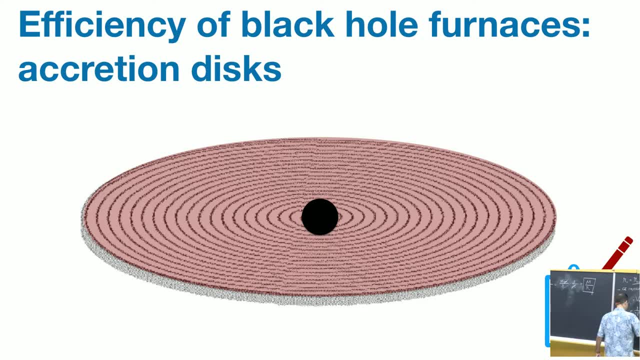 but if you do this calculation for a Kerr black hole, for a Kerr black hole, the Kerr black hole, the ASCO is smaller, so you have extra energy. for a Kerr black hole, the calculation gives you 42% efficiency for a not exactly. 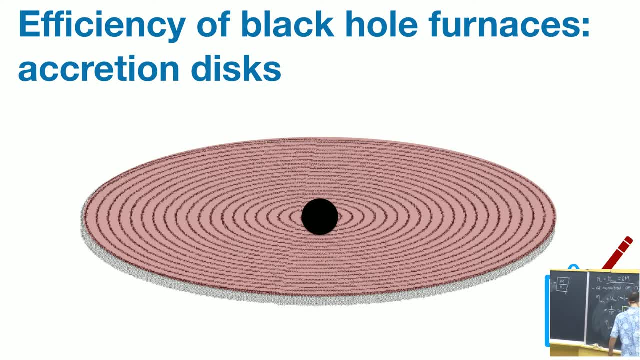 a maximally spinning black hole. to have maximally spinning black holes, but for the highest spin that you can conceivably achieve in astronomy due to the back reaction of photons that are accreting onto the. so you can have efficiencies ranging from 6% to. 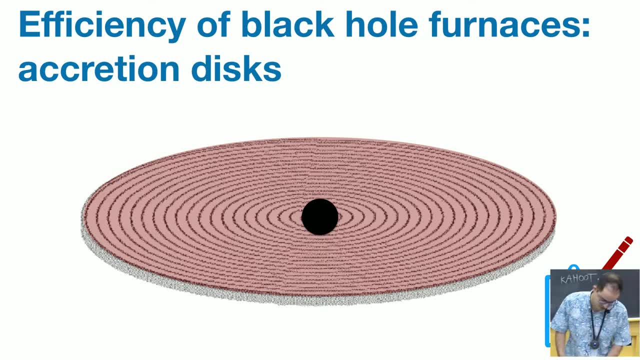 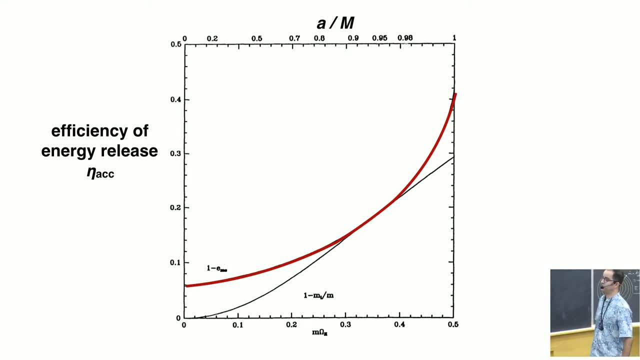 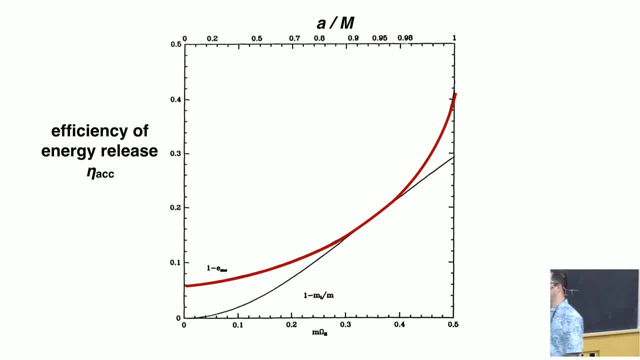 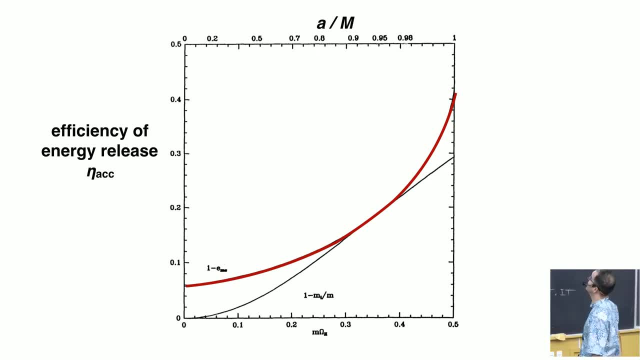 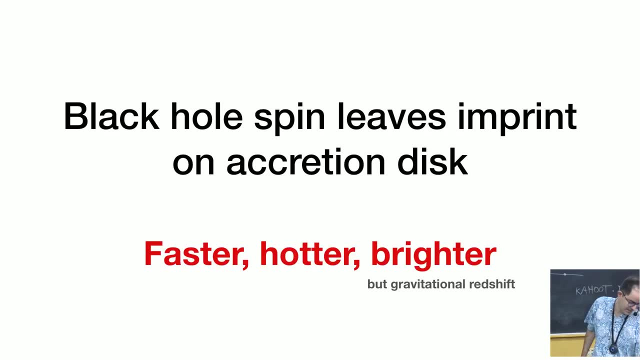 the upper axis. ok, so you can see it going from 6% continuously up to 40%. so black hole spin in conclusion. black hole spin in the conclusion. in conclusion, in the release of energy by a question. discs is the one of the most efficient engines of energy extraction in the. 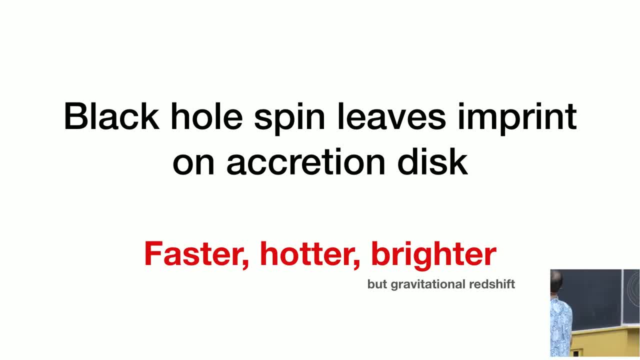 universe. ok, number one and number two: black hole. spin leaves a considerable imprint on the accretion disk. it's faster, it's hotter, it's brighter, ok, but there is also more gravitational redshift which will lower the luminosity of your disc at the same time. for a curve, maximally spinning curve, black hole. so 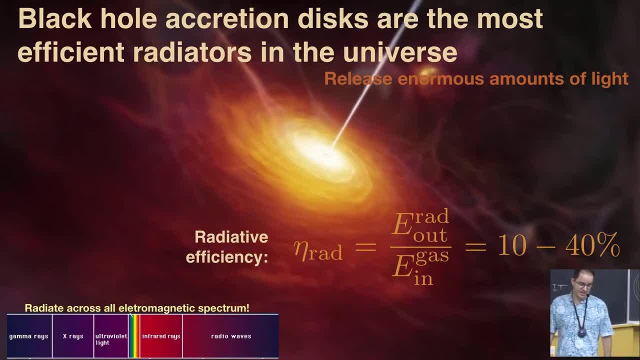 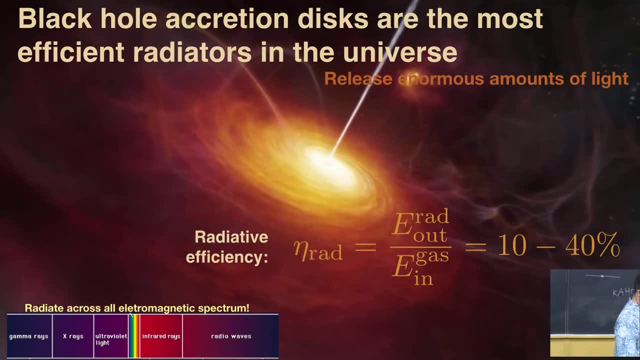 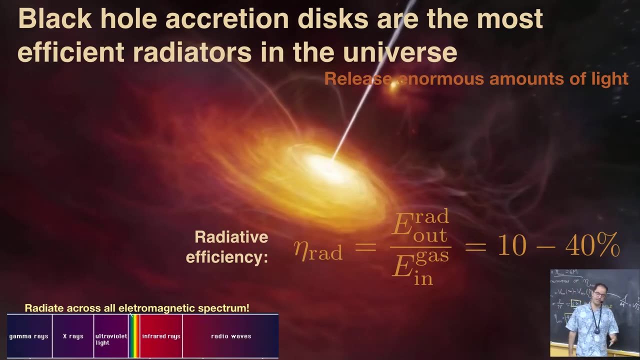 the conclusion here: black hole accretion discs. they are the most efficient radiators of electromagnetic energy in the universe. ok, they release in principle. only looking at these two numbers here, these two efficiencies, you can have gigantic amounts of energy of conversion of mass into energy due to this energy. 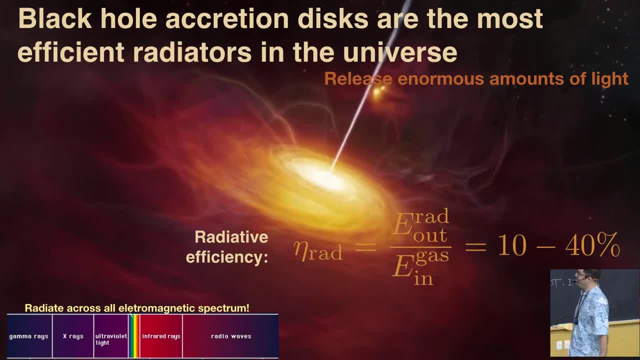 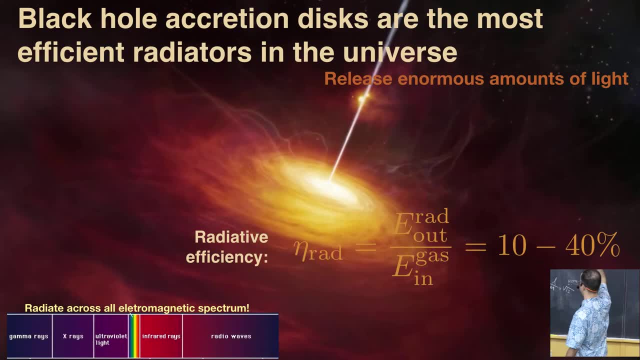 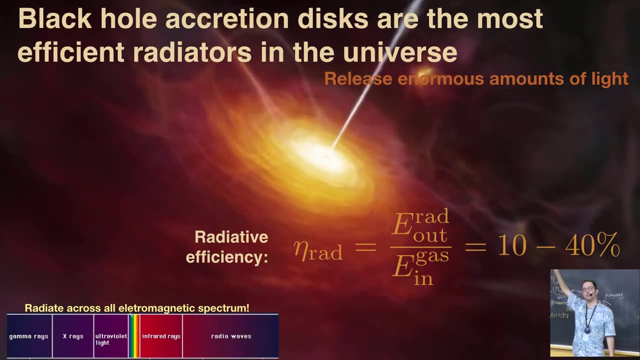 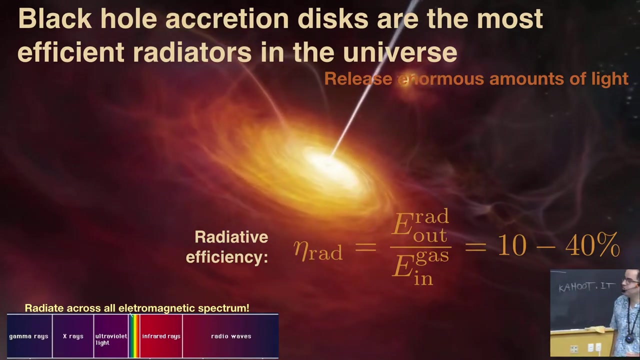 ok, expect in principle to see this energy flowing in the electromagnetic spectra somewhere in the electromagnetic spectrum question I will address in the next lecture. are in the electromagnetic spectrum? will you see this energy being extracted from the space-time around the black hole? to give you some conflicts here, these numbers might not look like much. okay, between 10. 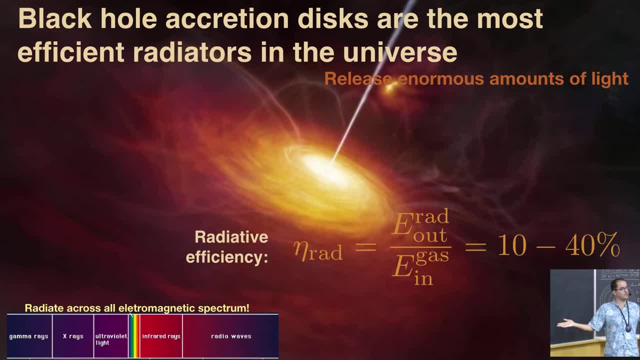 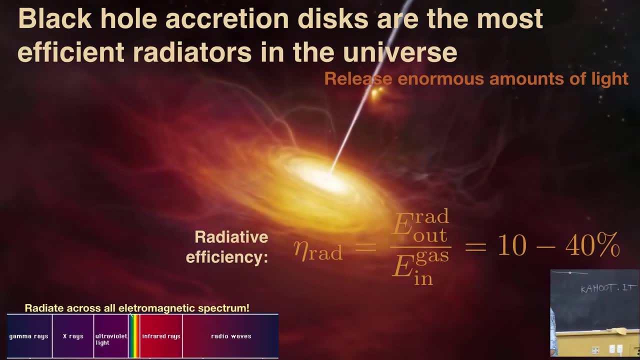 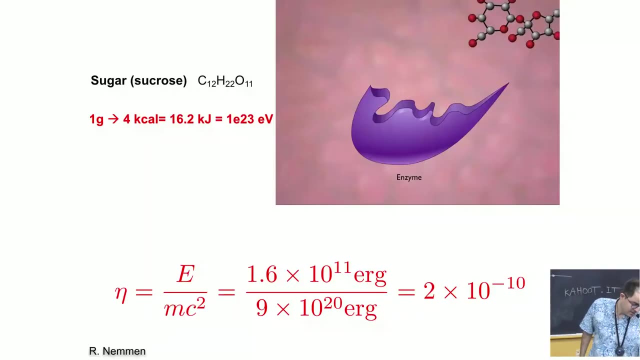 to 40 percent. okay, who cares? okay, but let's compare these efficiencies with typical efficiencies of process processes that are important and cherished for, important and dear and close to us. so let's imagine you give one gram of, you give one gram of okay to to some, to an end okay, and it releases. 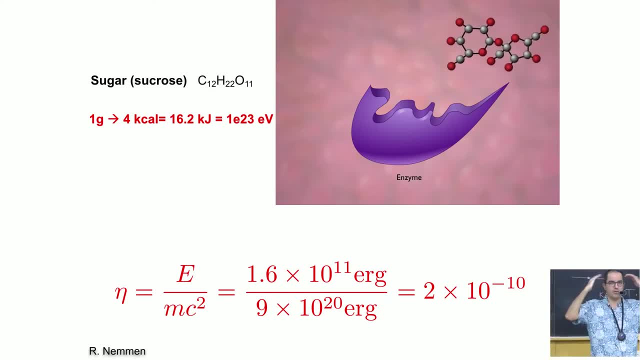 energy which will power your muscles. it will power your thoughts. okay, how much energy can you extract by one, from one gram of sugar, by one gram of sugar? okay, the efficiency of this process is 10 to the minus 11. okay, so they are. it's a very inefficient process, okay, our evolved biology over after 12, 14 billion years. nature. 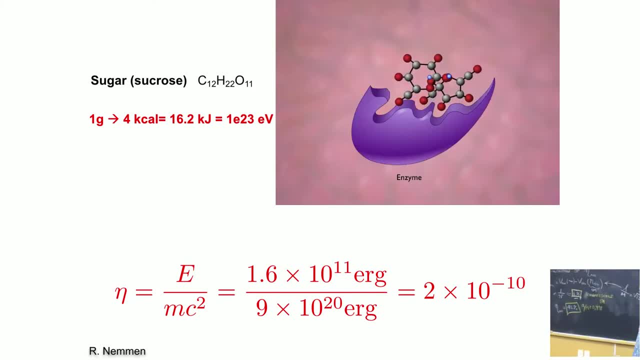 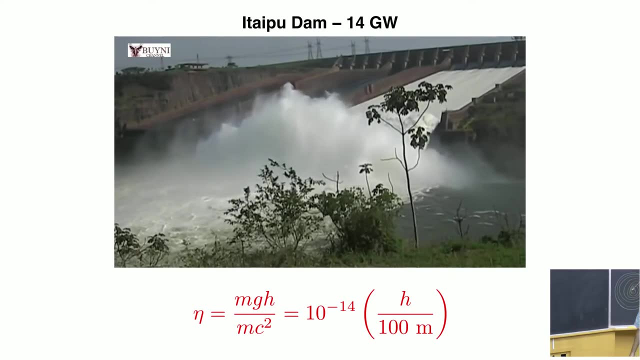 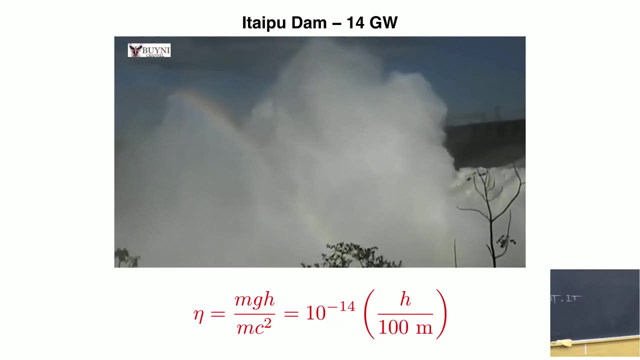 evolved a highly inefficient engine of extracting chemical energy from sugar. let's now consider a man-made machine. okay, a hydroelectric dam like the Itaipu dam? okay, you give one gram of water into this engine? okay, extract some of the potential energy of the water falling. how much energy can? 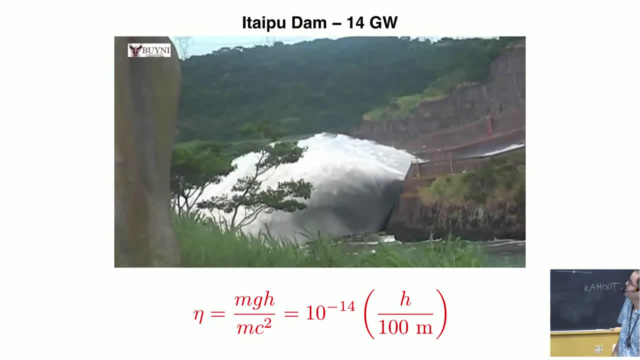 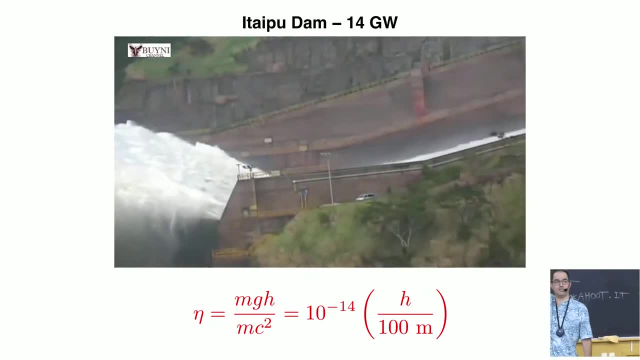 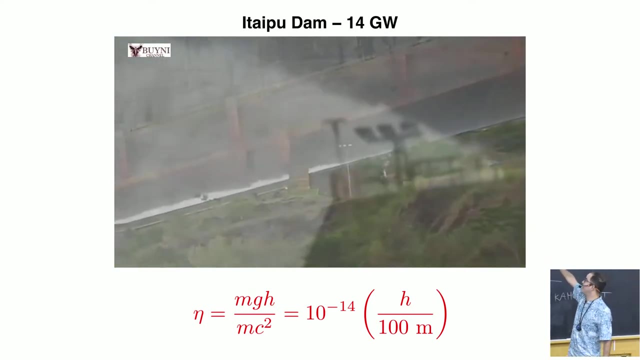 you get from one gram of falling water. you can very easily compute the efficiency to get a number which is 10 to the minus 14, which is a thousand times as efficient than our biological engines, walking here and thinking: okay, you can bump this up to around 100 efficiency if water falls close. 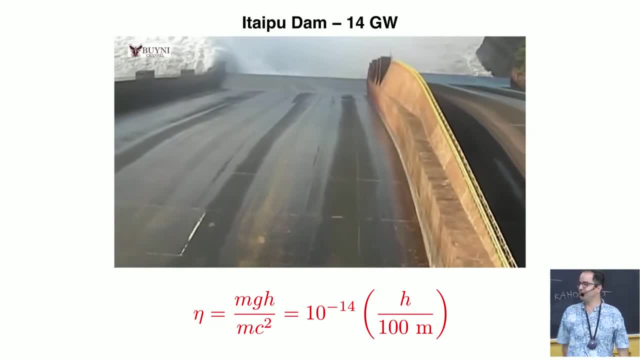 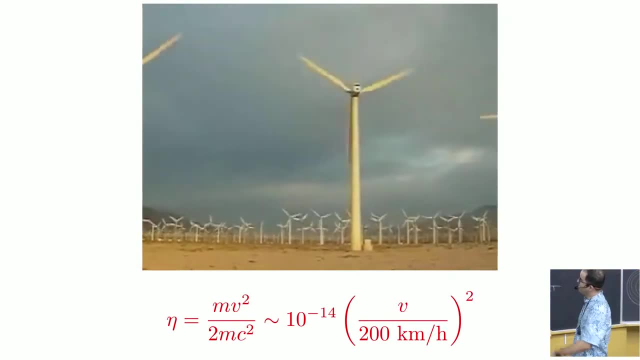 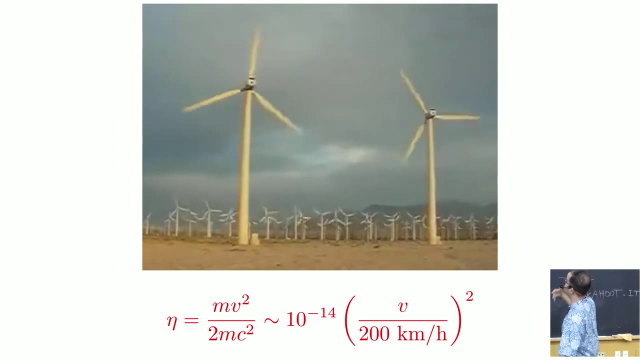 if you have an Itaipu dam with a height of close to the size of the solar system, I think now let's consider uh extraction of a eolic energy. you write a very simple calculation. you write the the the energy extracted by the kinetic energy of air, its efficiency of 10 to the minus 14.. okay now 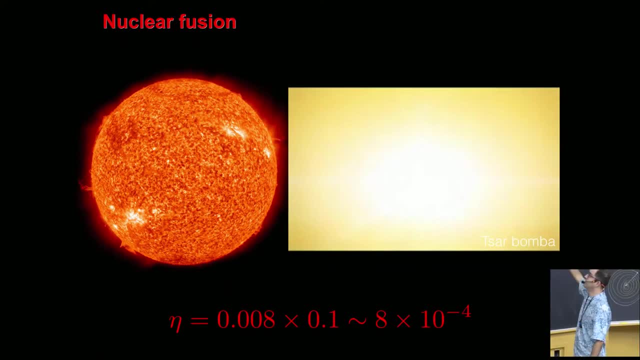 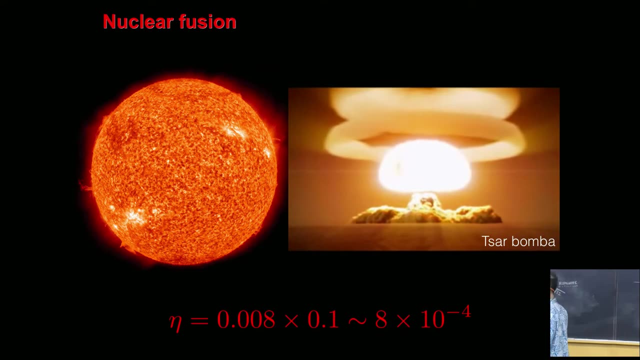 you go to nuclear fusion and what you'll see here is one of the- I think it was the largest, probably- nuclear test that side, Bomba, which I think was 10 megatons. no, probably, I don't remember, probably 10 megatons. okay, the efficiency of extraction of energy when you fuse nuclei to is 10 to the minus. 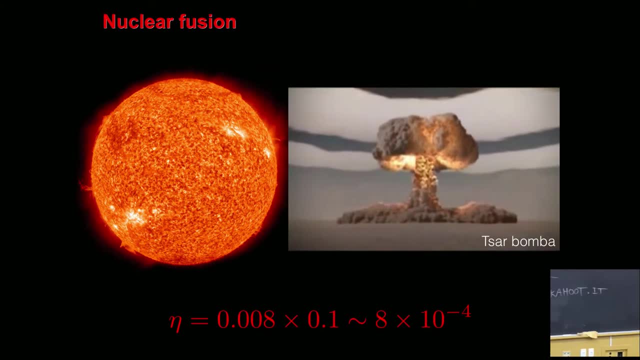 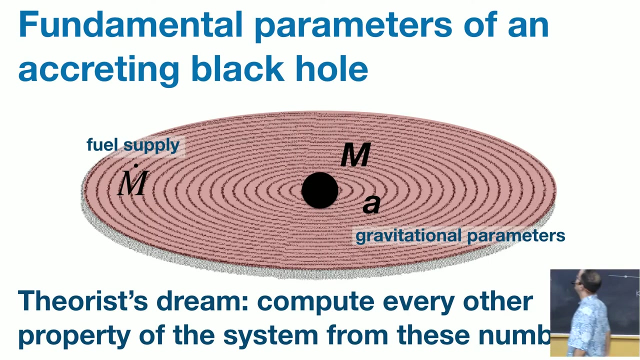 three more. okay, so this qualifies black hole engines powered by gravity as the most efficient engines in the universe for for obtaining electromagnetic radiation. wrap up, Ricardo. yeah, uh. so what are the fundamental parameters of an accreting black hole? okay, we know that one of the parameters is the mass, the second parameter is the spin and the third better. 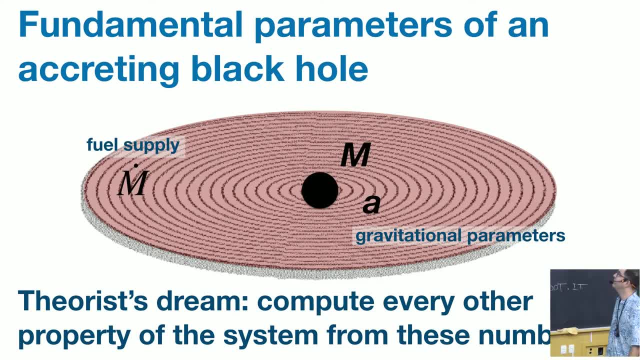 is the accretion rate, the rate of inflowing matter that is flowing towards the central object, which we call m dot, the m dot that I define here. okay, this is a fundamental parameter in astrophysics. okay, this is related to what some physicists call dirty physics. okay, it's not only the gravity only. 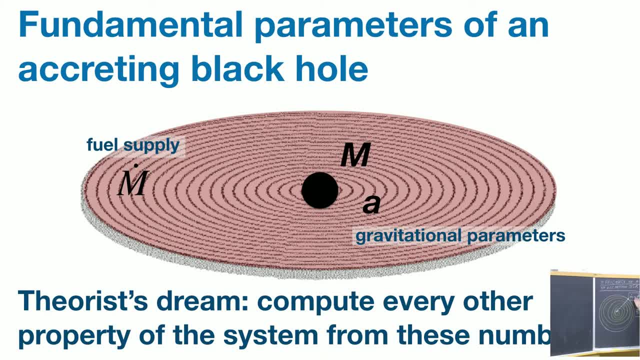 the, the space-time Dynamics, okay. you have to worry when you have fluids around the black hole, with things about hydrodynamics, okay, viscosity and these kinds of things. it is a theorist's dream to compute every conceivable property of the system to give to your astronomer friends to compare. 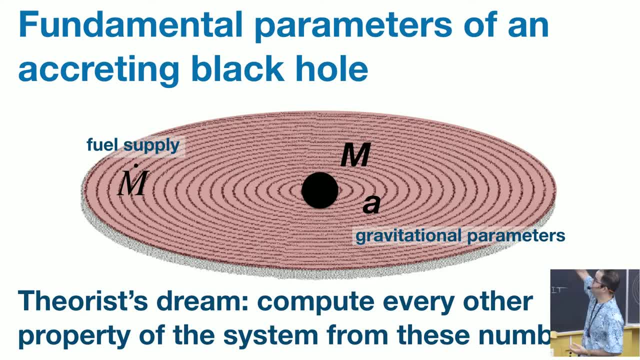 stream to compute every property from just these three numbers of about a black hole in astrophysics- from the mass, the spin and the accretion rate. okay, so the next lecture. I will quickly review some concepts of fluid Dynamics, talk more about accretion discs and move on to outflows from black. 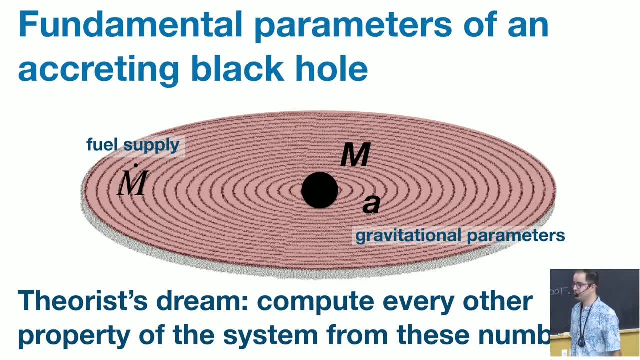 holes and their radiation signatures. thank you, hi. you have a full supply for the for the mass of the black hole. they have something similar for the angular momentum, or it's a fixed parameter? uh, yeah, in the accretion, this, the accretion disc, is a feeding mass and it's feeding also, uh, some amount. 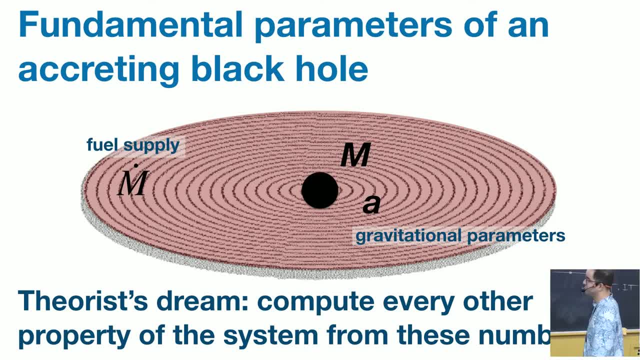 of angular momentum which will, over time, change the mass of the black hole and will change the spin of the black hole. okay, and here I put, the mass is the most important. of course it's very hard to reduce to only these three numbers because when you have fluids, things, things, 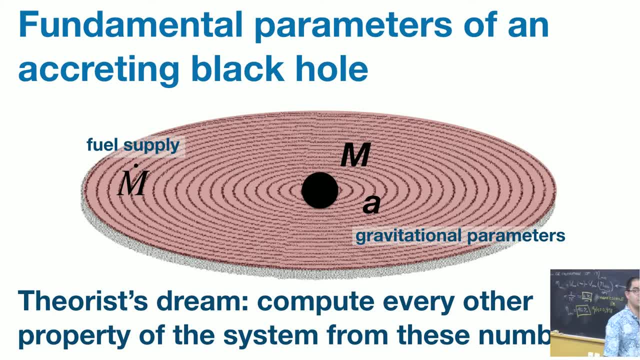 get more complicated. you have them as I will talk tomorrow: the Navier-Stokes equation and turbulence and this sorts of uh and magnetic fields also, which I will just barely mention because MHD it's a complicated, so one one big unsolved puzzle in black hole astrophysics is. 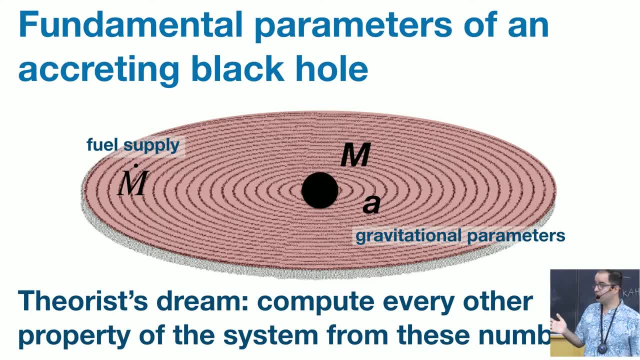 what is the final spin of black holes? okay, so LIGO is helping us to address this question. okay, should we have maximally speed black holes in 10 to maximally spinning black holes, or in between, or they tend to threshold, uh, to structural spins? okay, in in binary systems this. 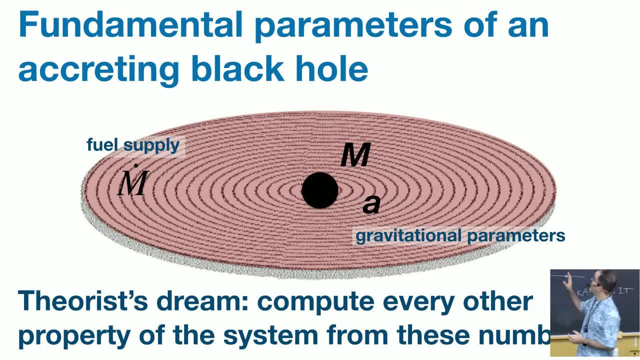 is a. this is a bit more complicated, but when you have one single clean black hole accreting mass, this is also an unsolved question which will have cosmological implications. so in one of my, one of my lectures, I will touch on this issue of the spin evolution of supermassive black holes, and it can. 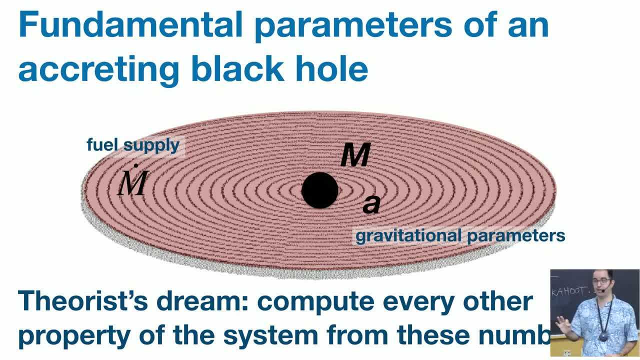 have magnetic impacts on the galaxies and cosmology. okay, so this is very interesting: the connection between the micro and the macro in the cosmos. yeah, so sorry, just a follow-up on this, but can you relate the amount of angular momentum donated to the central black hole to the M dot? so 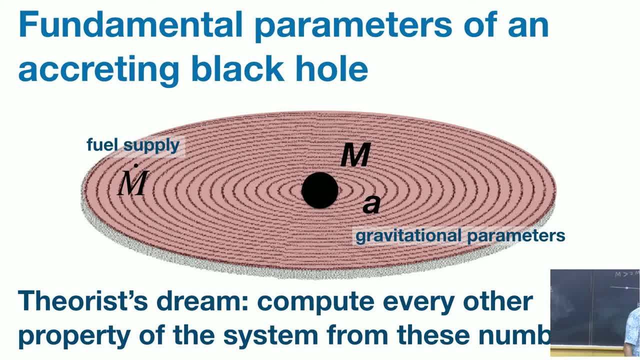 can they be related? probably yes, I don't have a clean argument to give you a clean analytical argument, but hook up an exercise for the students. yeah, it would be an interesting. it would be an interesting exercise and I will mention we are now doing numerical simulations of accretion onto black holes and for sure you can do a virtual. 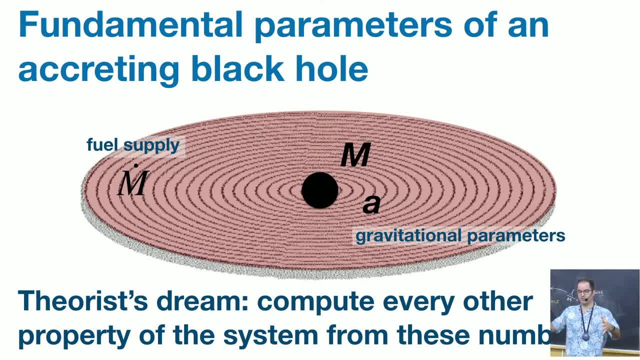 virtual reality, a virtual laboratory, a controlled experiment, and you can measure it in the simulation. if there is a relation between the accretion rate and the angular momentum, this is a good question actually. so think about it. you can assume it was on circular orbit and then, oh, analytically for sure, I it's not. 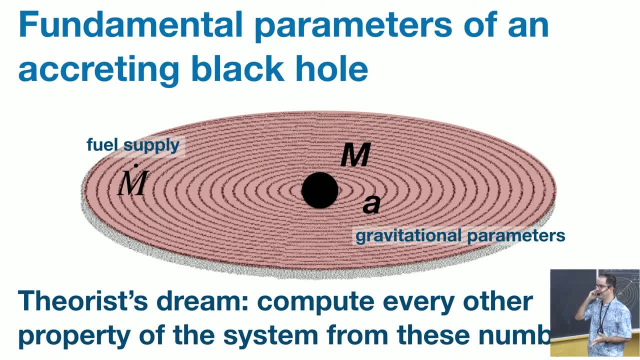 clear to me if it's a meaningful relationship. but sure, analytically you can do it. for a simple type of equation, disc hi, can a sure side black hole become a care black hole in the opposite? true, yes, yes, uh, sure to begin with, and it will be very hard to actually form a structural black hole in nature because 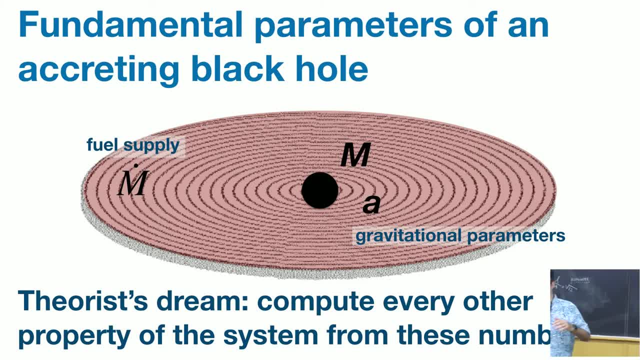 usually the collapsing Stars. it's either a neutron star or some other more massive Star. they usually have non-negligible amounts of angular momentum. okay, and it will be very hard to get rid of all these angular momentum with. the thing is, astrophysics is messy, okay, astrophysics. 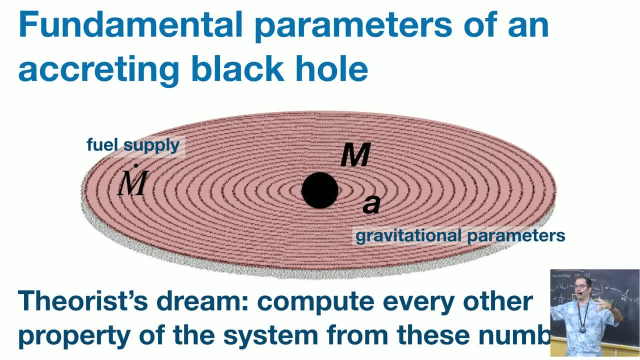 When you have a collapsing star, the star is losing mass, There is radiation pressure blowing away the outer layers of the star and it collapses. okay, It's usually very nonlinear processes, as nonlinear sometimes as gravitational waves, So it will be very hard to form a Schwarzschild black hole. 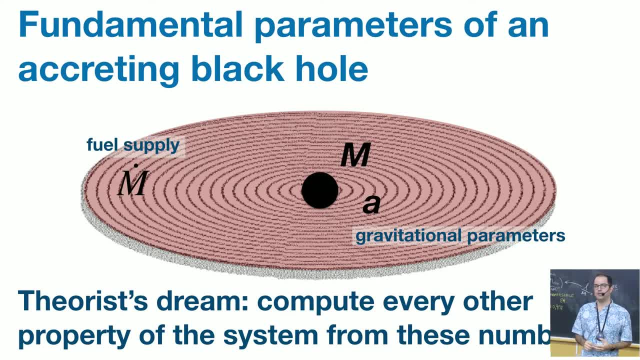 from any generic collapse. okay, So usually you start with spins around 0.3, 0.2 for typical black holes and you can either decrease that. Another way you can decrease or increase the spin is by merging black holes. okay, 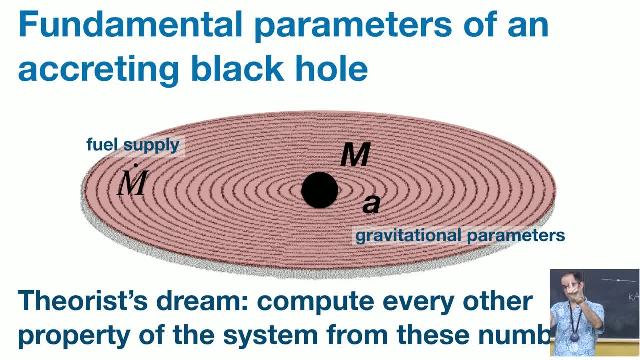 By merging black holes, two black holes with different orientations, The final black hole. you can play with the parameters such that the final black hole can decrease the spin, okay, depending on the mass emerger. But yes, you can either turn a Schwarzschild into Kerr and vice versa, okay. 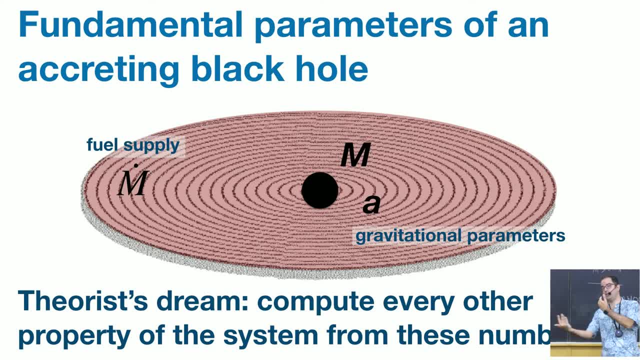 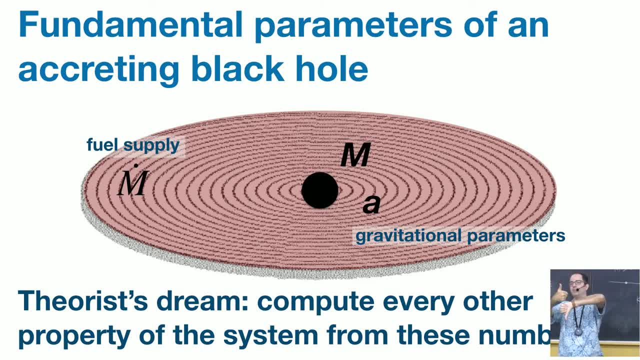 suppose this is the angular momentum of the black hole. okay, So you can play such that you keep feeding matter with different angular momentum and decrease this spin vector of the black hole. So just in the observation of LIGO they are all broadly consistent with individual black holes. 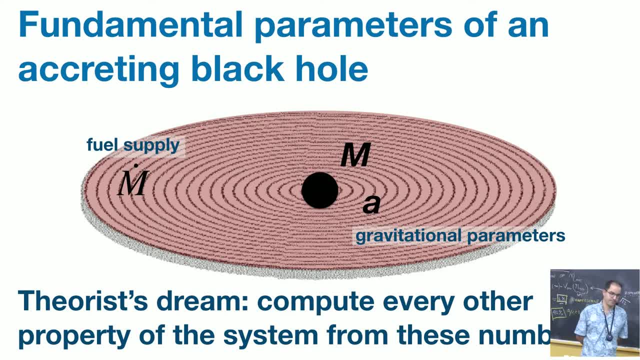 I mean originally black holes having spins up to point two, point three, and the final black point one, point two, point three, the original black holes, uh, before the merger, and the final black hole after the merger, to have been of point seven ish. this is. there are large error bars, but this is the broad. 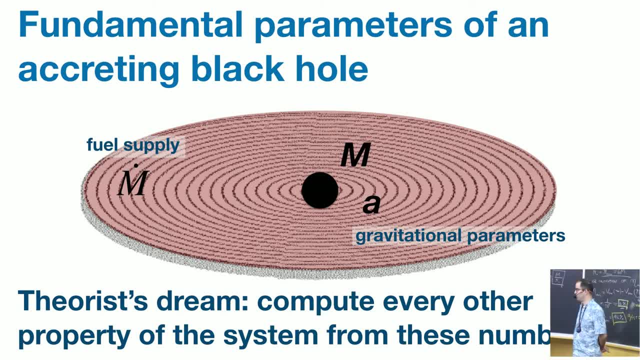 pitch and point two, point three. if you use model models of stellar evolution, you roughly expect point two. point three is the initial spin for astrophysical stellar colors, more or less so. you told us that black hole has a ring singularity, but to be honest i didn't understand this. how can the singularity 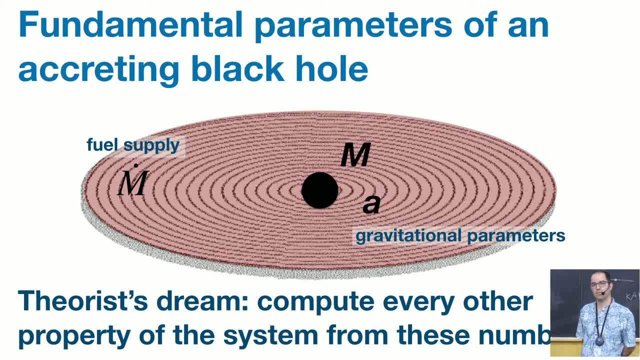 and moves down moves. how can the, how can you have a ring singularity- the way i understand this is in gr- is the classical theory. okay, gr is a classical theory and in classical mechanics you cannot have point particles with angular momentum. okay, because the moment of inertia 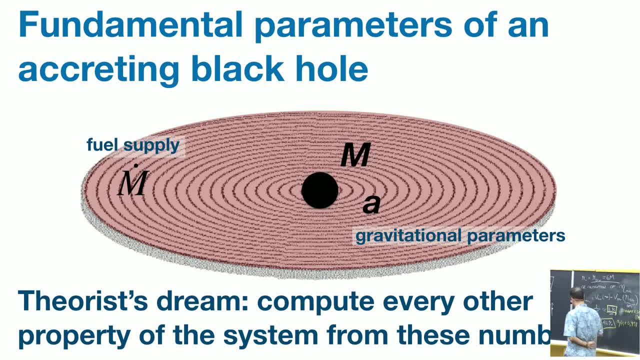 will become will will go to infinity, right? uh, so this is the thing. it's a classical theory. a partial black hole has a point part. it's a the classical black hole. it is a point point particle located at a singularity. okay. all the mass is located at a singularity, okay. 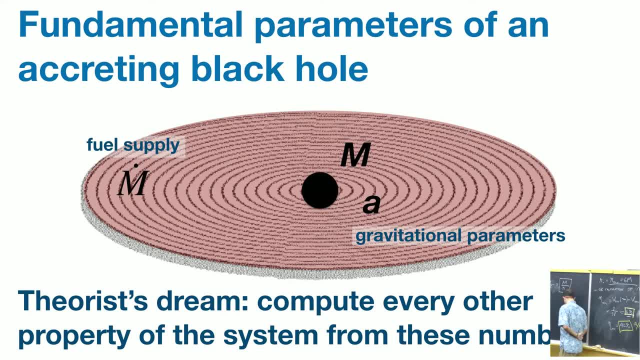 the singularity, it doesn't spin. when you start adding angular momentum to this point particle in the curve black hole, it doesn't have any other choice but to spread this angular momentum into a ring. otherwise the you cannot have point particles with angular momentum in classical mechanics. for that simple reason, maybe one of the other uh speakers can add a bit of uh. 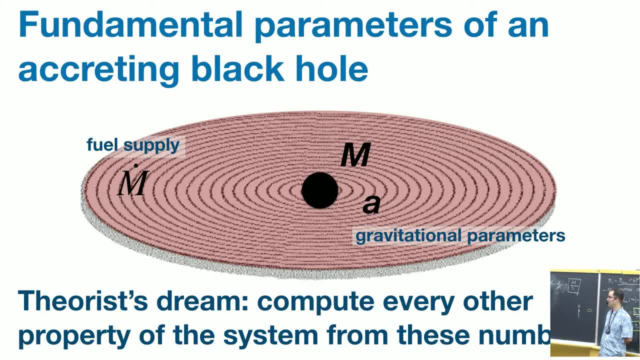 do you have anything to add? angular momentum, mass: they are measured through. i mean, you don't measure the mass and angular momentum by putting a probe. i mean inside the core. you measure the property of the space time. yep, and so by measuring the coefficient, the one over r fall off of the. 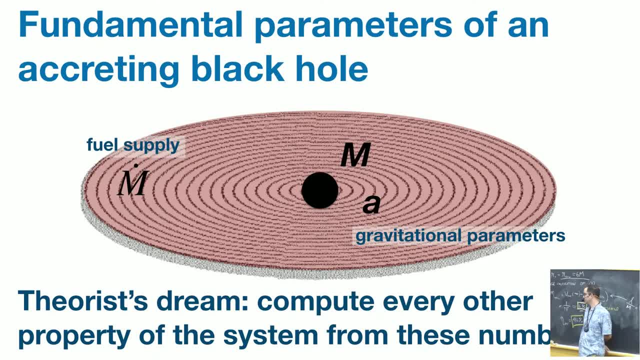 potential. you measure the mass by measuring the torque on test particle. you measure the angular momentum, so it's really a property of the space time. yeah, yeah, yeah, sure, but did i did, uh, following that that comment, since the properties, and only indirectly? how can you be so sure that that these, these numbers that you get, are in fact or are? 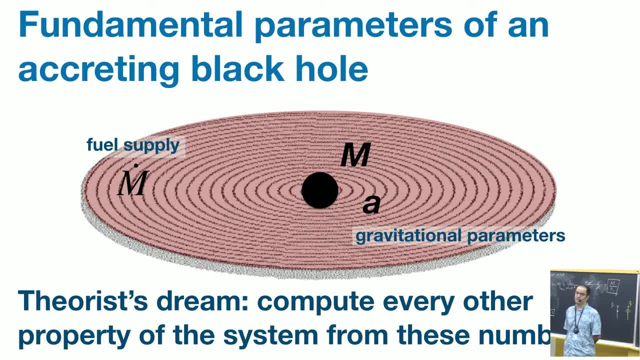 inequivocal from a black hole or in a kevil call for a black hole. the numbers for what? the numbers for following that command? we measure things. we get numbers that we think that are coming from black holes, that how can you be so sure that those numbers that we get are in fact from from black holes? 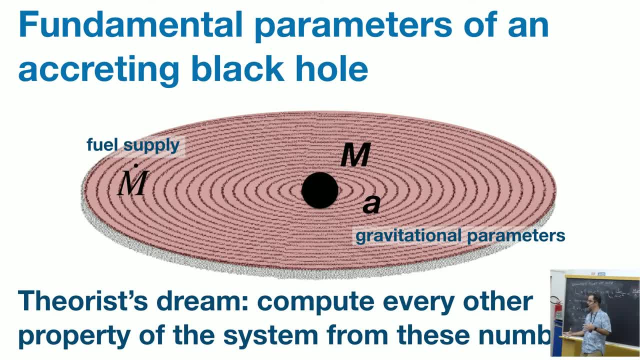 are not already? already, are you referring to the mass, the efficiency of accretion, the luminosity, all the parameters that that define a black? okay, okay. so, first of all, everything i'm doing here, i'm doing on the assumption that we can compare with observations. okay, i wouldn't do astrophysics. 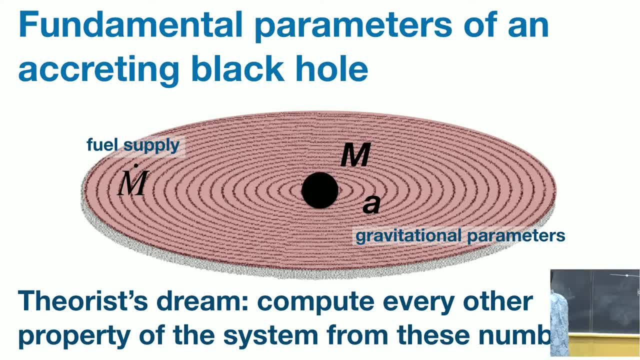 if i couldn't measure the, if i couldn't compare the numbers of my theory with observations. okay, so, regarding the efficiency, there are ways of estimating the efficient, the energetic yield of accretion black holes from observations. okay, there are several different ways. one of the ways is, i will mention, about sig, observational signatures in the 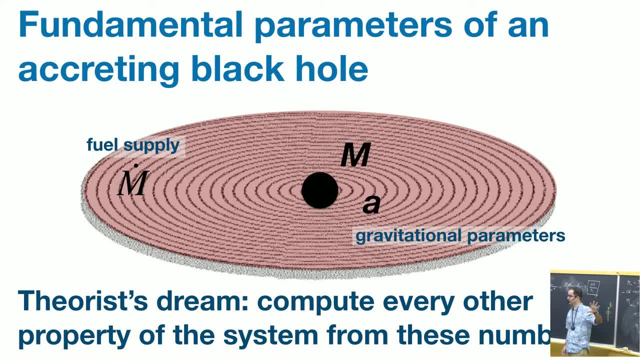 electromagnetic spectrum of black holes in the next lecture. okay, but one of the signatures that you are looking at, a black hole, is counter-intuitively, paradoxically, very strong x-ray emission. okay, not from the event horizon, of course, but from the accretion disk high. 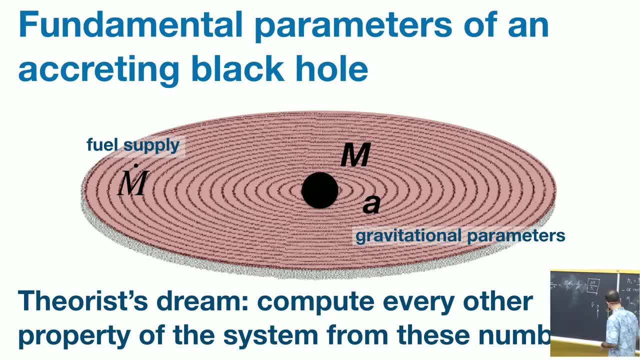 temperatures, high energy, x-rays. What you can do in these systems, what an astronomer can do, is you make a plot of the energy spectrum- okay, energy times flux for the flux of energy, and then you go at the resulting spectrum and you 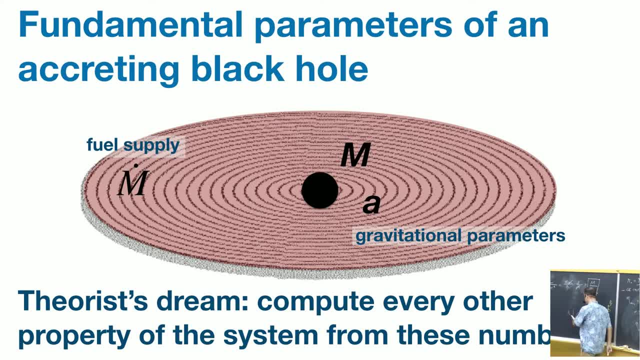 can actually measure the energy that is flowing out of this system- okay, and you can use the physics of GR to try to derive the accretion rate. and then you compare what you observe here with what the theory tells you we find is correct and you can have a view of the efficiency of the system. okay, and things. 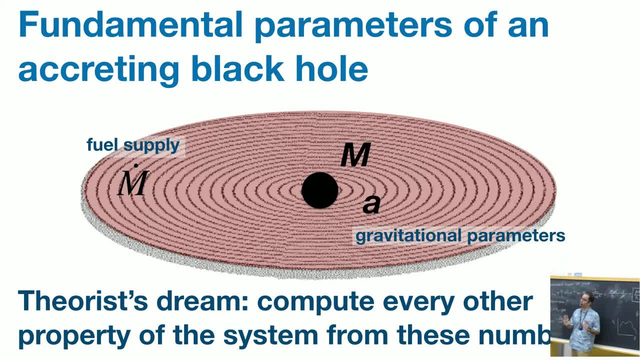 never go the way you want them to go. confronted GR GR always has been able to explain the observations of these accreting black holes. We can play similar games with supermassive black holes in the centers of galaxies. We can play this game. It's more hard with gamma ray bursts. We can keep playing. 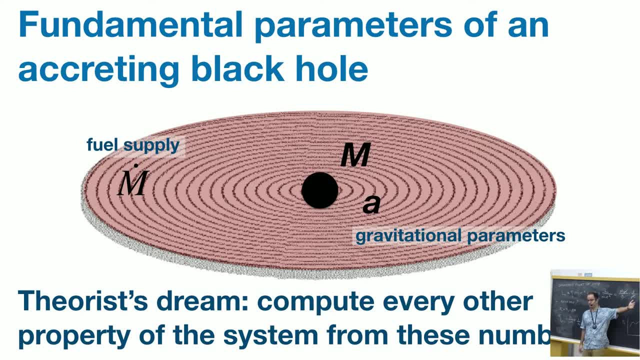 this game. okay, Mass, I will mention next lecture. we can measure mass with test particles far away from the black hole. We can have an idea of spins of black holes. with electromagnetic observations It's harder but we can have an idea. okay, So everything you can constrain from. 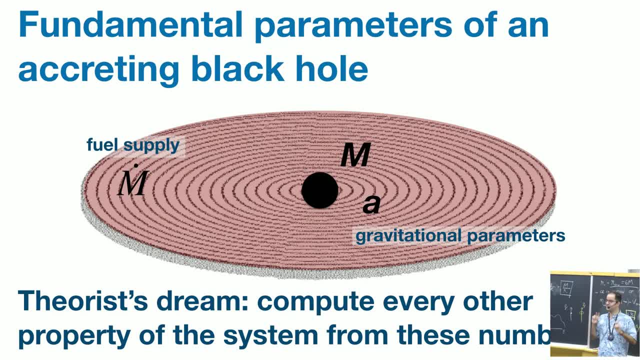 observations. but, as I said, astronomy is a bit dirty because you always have things which are trying to confuse observers. okay, Dust, for instance, other things, but all of these can be measured. okay, Accretion disks: Accretion is essentially a lot of particles that are spiraling and falling into the black. 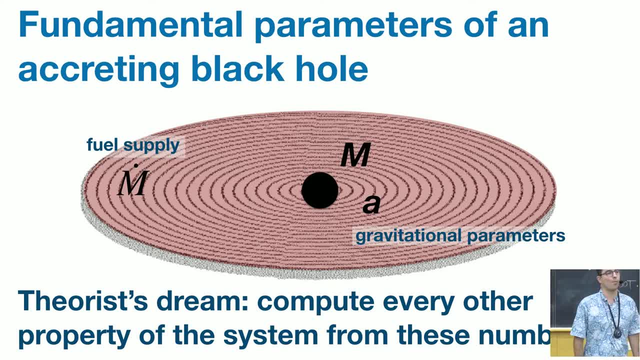 hole In the future, can we see some gravitational wave emission from these systems, some continuous gravitational wave emission, because we have particles fall, spiraling and falling to the black hole. Well, in principle, sure there is gravitational wave emission. okay, You have a non-spherical 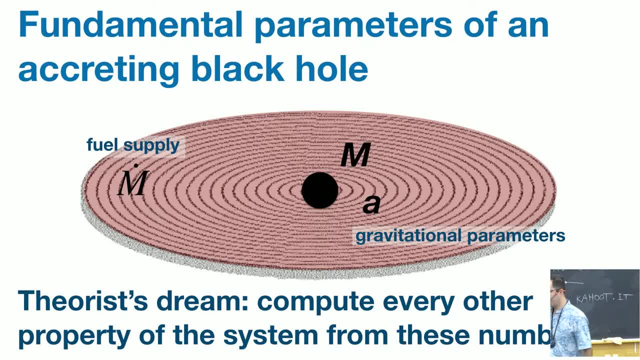 accelerated system. okay, But the thing is that the amplitude of the gravitational waves will be effectively non-observable. okay, I don't think it will be, for the simple fact that for the typical astrophysical systems we will deal with, in x-ray binaries and the centers of galaxies, the mass I have to compute. 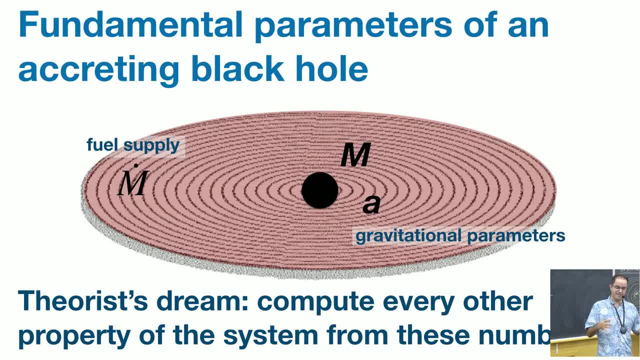 this number okay, from yesterday. but the mass of the accretion disk is many, many, many orders of magnitude lower than the mass of the gravitational waves, So there is a is lower than the mass of the black hole. So the accretion disk, the spacetime dynamics, 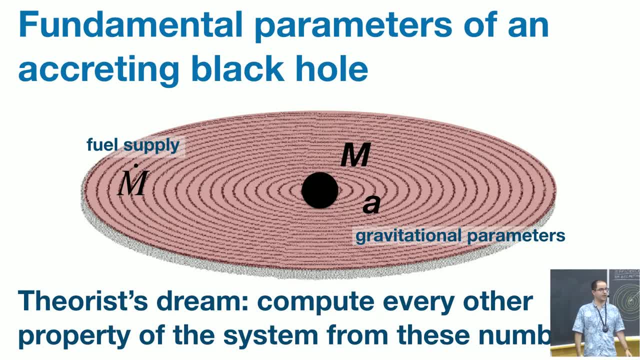 because of the accretion disk is negligible. Now, if you have a binary supermassive black hole, it's a different thing. And also in gamma ray bursts, the accretion of matter from the coalescence of neutron stars. 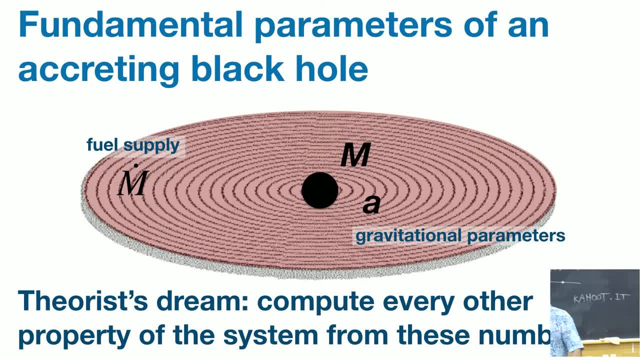 which is the accretion disk itself, because the accretion disk can be important, But not for most of the systems we will deal with. So I think that if the accretion disk would just be a disk, it wouldn't emit any gravitational waves. 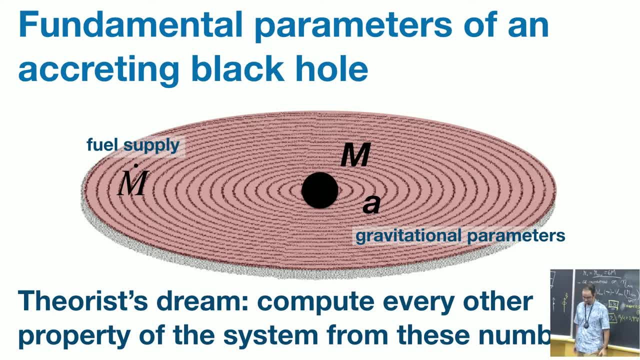 Because of the symmetry. OK, So the inhomogeneities in the disk that would, But then of course very weak. But if you would have some large chunks then you would get. Thank you, thank you. This is the. 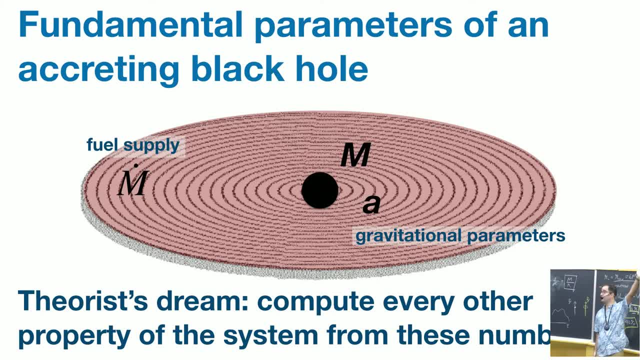 This is the dream's view of an accretion disk. But real accretion disks are inhomogeneous. OK, They are not perfectly spherical or symmetric. OK, Thank you very much. It's not spherical. even axial symmetry. Also, it's not perfect, OK. 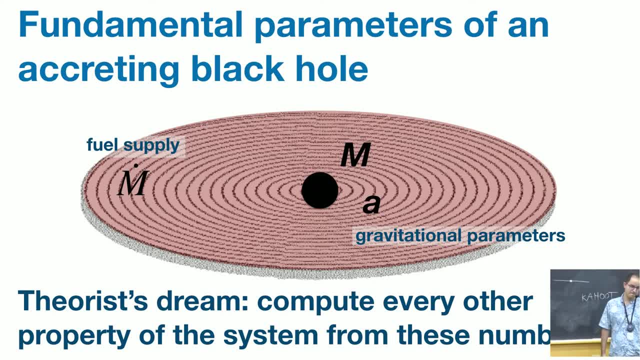 Symmetric does not emit like a black hole. Last question: Well, I'd like to know how the light guns look like in the ergosphere, inside the ergosphere. Oh, That's possible. How's that? Do you have any idea how they look like?